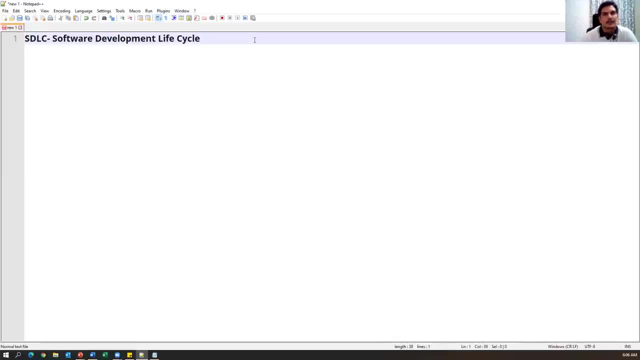 develop the code or develop the software, And after that we conduct testing on the software And finally we release the software to the customer. So in each and every activity should go in different phases. Okay, so what SDLC means? SDLC is a software development lifecycle. 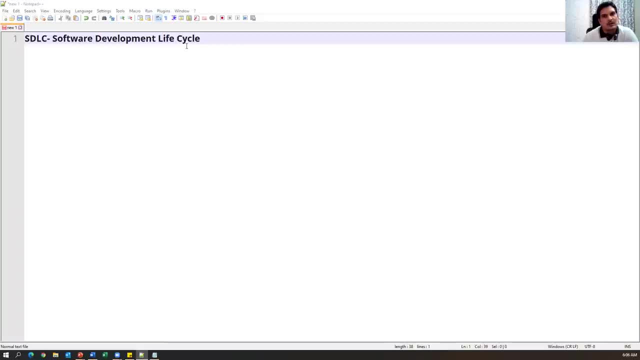 which is a process used by software industry: design, develop and test the software. Okay, so this is a basic definition of SDLC. SDLC is a step by step process which we have to follow to deliver, or to develop, test and deliver the software to the 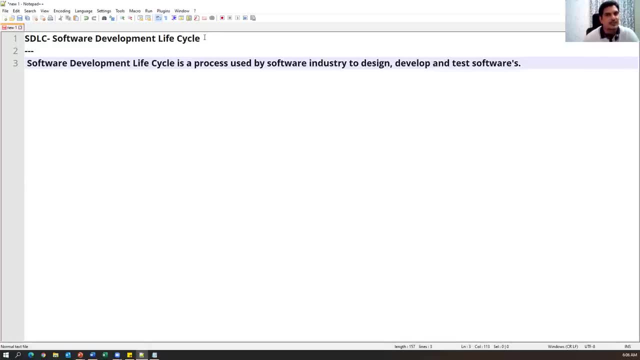 customer. So if we don't have proper process, it is very difficult to achieve it right. So we need to have some process. So if I take any company, there are three P's. are there guys? Three P's are very important. So one P is. 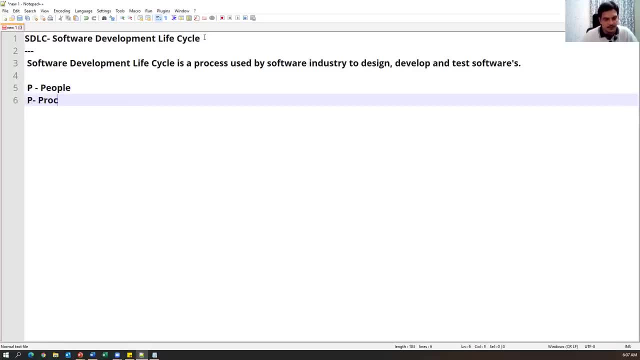 people, And the second P is process And the third P is product. So these are the three main things, or we can say three pillars of any company, not only IT company. So what P? first P means people, So the company means there should be some people. 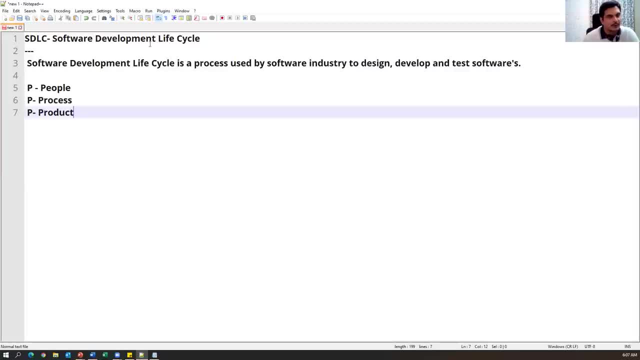 And they do some kind of development or testing, whatever. So people are very, very important. Without people there is no company. So this is one pillar. The second thing is we have to follow certain process And that means there is no коли service. Right, If you want to achieve something, we should have some process and we have to go through certain stages And finally we can achieve the goal. So the second P is representing the process which we have to follow in our company. So the third P is representing the product. So what is product means? finally, whatever we 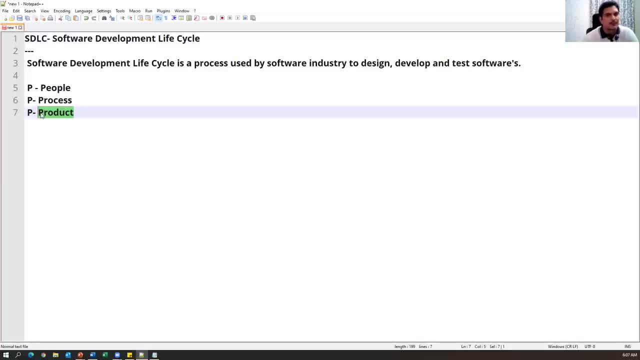 deliver to the customer. that is called as a product or application. So if you want to deliver a product to the customer, the people should follow a certain process. Then we can deliver some product, product to the customer. So these three P's are three pillars of any company. people should. 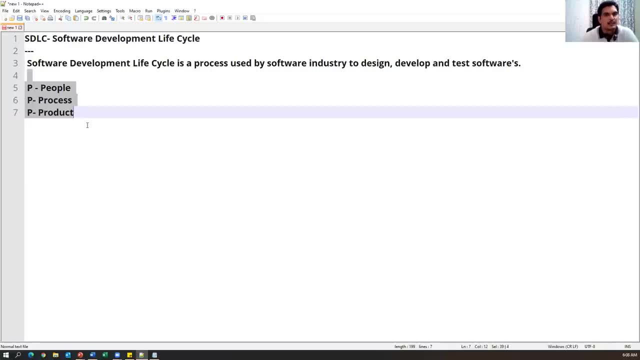 be there. there should be some process and then we can deliver proper product or quality product to the customer. So there are three P's. So this software development lifecycle is related to the process which will normally talking about the process which we have to follow to develop or to design, develop, test the software or deliver the software. Finally, 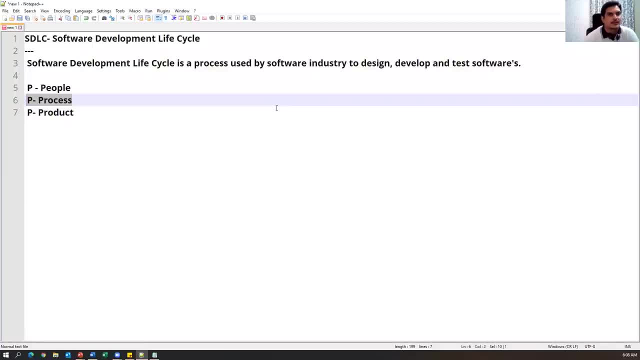 we deliver the software to the customer. So that is simply to say SDLC. So SDLC means it is software development lifecycle is a process used by software industry to design, develop and test the software and which contains certain phases, So the software development. 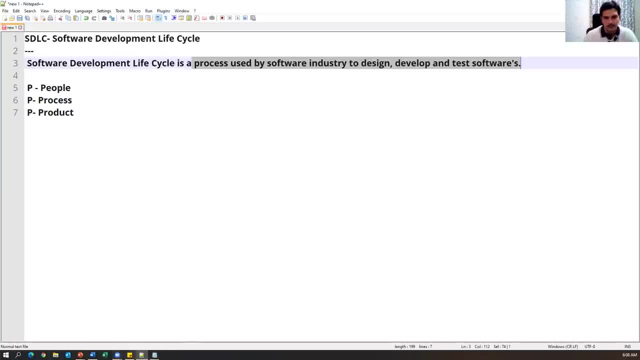 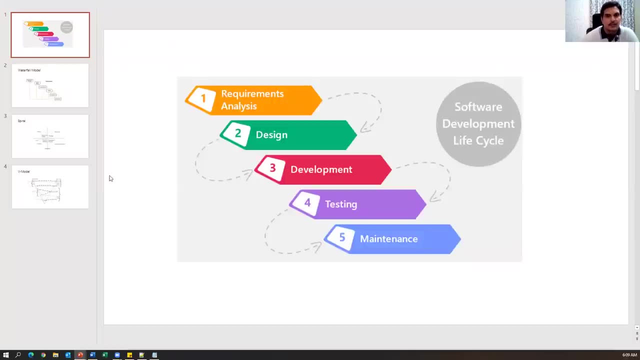 will happen in those phases. So what are those phases? Now let me just share a small presentation, then you can understand. So now we can just look at this picture. So here we start with the requirement analysis and then we have design part, then development. 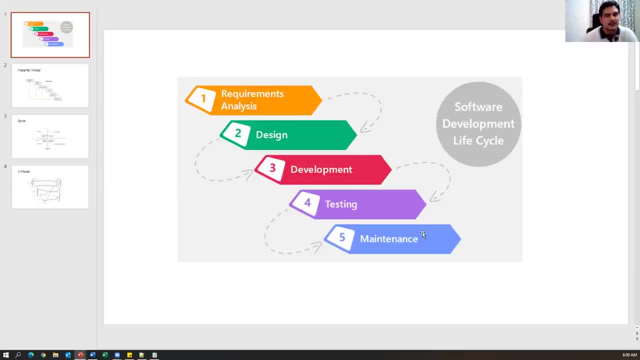 testing and maintenance. So these are the different phases which we have in SDLC. SDLC means software development lifecycle. In every company, we should follow certain process if you want to deliver a product, if you want to deliver a quality product. So this is talking. 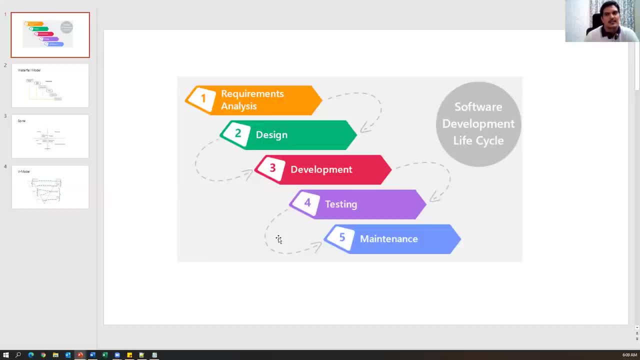 about SDLC, So which contains certain phases, or we can say it is a step by step process which we have to follow. So the first phase is a requirement analysis phase. So what we do in the requirement analysis phase means we have to collect the requirements from the customer, So we have to collect the 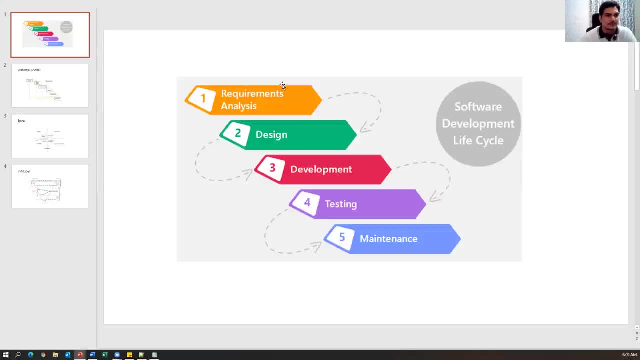 requirements. we have to understand the requirement from the customer. So normally project managers or product managers will be involved in this particular phase. So they will talk to the customers, they will get the requirements and they prepare certain number of documents will be there. So that is the requirement analysis. That's the first phase in SDLC. 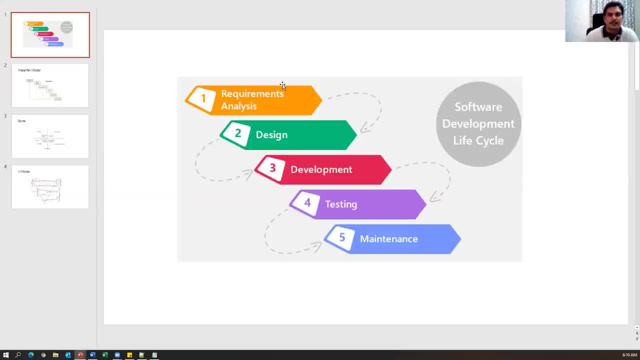 And after completion of requirement analysis, the next phase is a design phase. So in the normal, in the design phase, what happens is the designers will design the software. Okay, so normally, if I just say one example, if you want to construct a house, right, what? 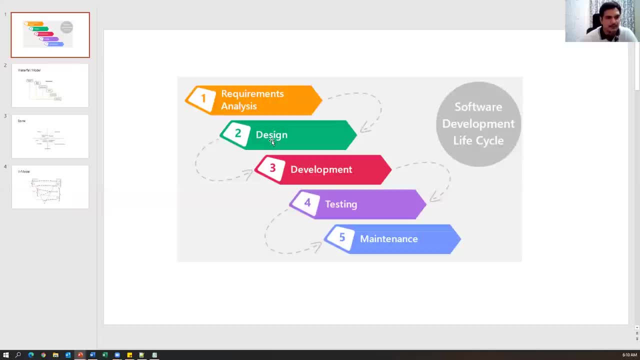 you will do. first you will have a blueprint or we can say plan, So that is a simple design, And later we will develop that. Similarly, once you get the requirement from the customer or client, The designers will prepare the design part. So they will design the software how it should. 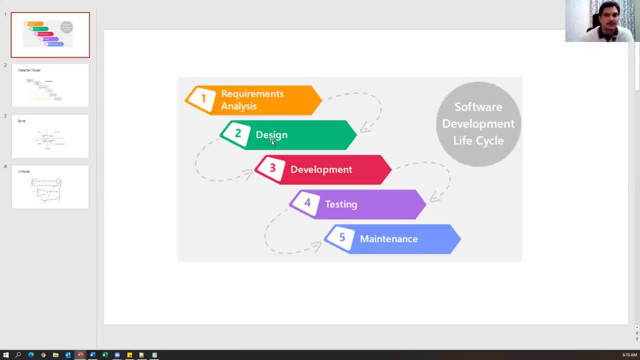 look like like UI part and navigations and everything. And after completion of the design, development will start. So development, or we can say coding part, will start. So developers, software developers- will develop the software by writing different type of programs, by using different type of languages. Okay, so this is a part of a development. Just a moment. 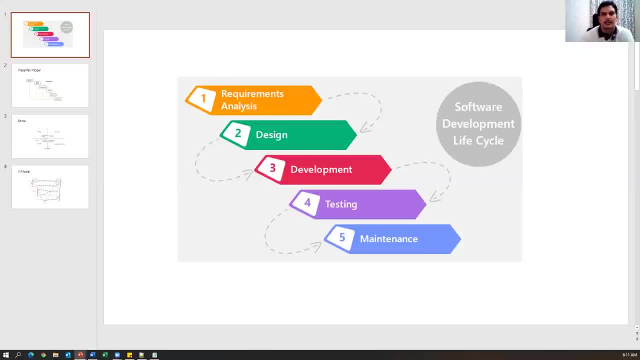 Okay, so development requirement analysis, design and development, And the next phase is the testing phase. So what testing phase means? after development is completed, before delivering the software to the customer, we have to test it. So we have to conduct a different. 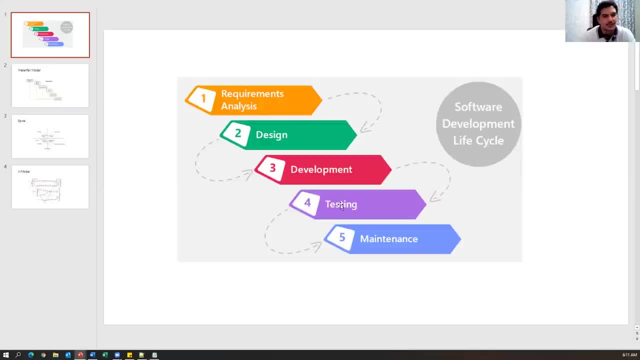 type of testing like functional, non functional, performance security. so different type of testing we are going to conduct as part of testing phase And normally the people who are involved in the testing phase, they are going to conduct a different type of testing. 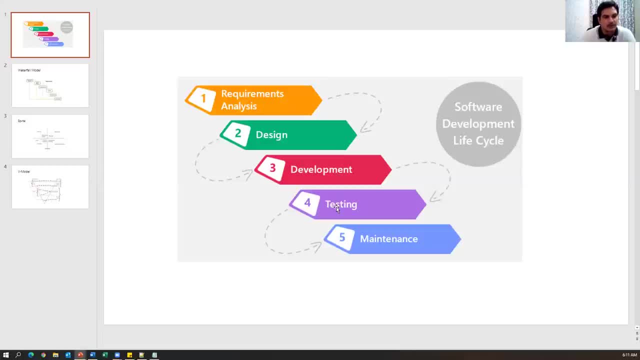 So we have to test them And for the testing phase we can call them as a tester or a QA or QC. All these kinds of people are involved in the testing phase. After that, finally, we deliver the software and maintenance will be start. So maintenance in the sense we deploy. 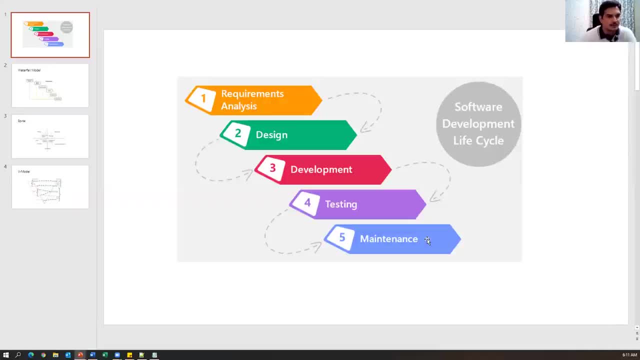 the software in customer environment and they start using the software. So these are the different steps or phases which we have to follow to deliver the quality product to the customer. So this is basically software development lifecycle. Every software development should go through process. that process is called as software development lifecycle process. okay, so this is. 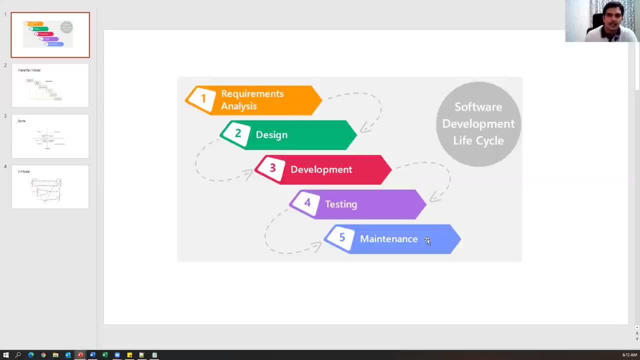 a basic understanding now. so the companies follow certain number of models. so again, this is very high level sdlc, we can say, and companies will design or they follow different models. all these comes under sdlc only, but approach, the way of following these phases, are different. okay, so 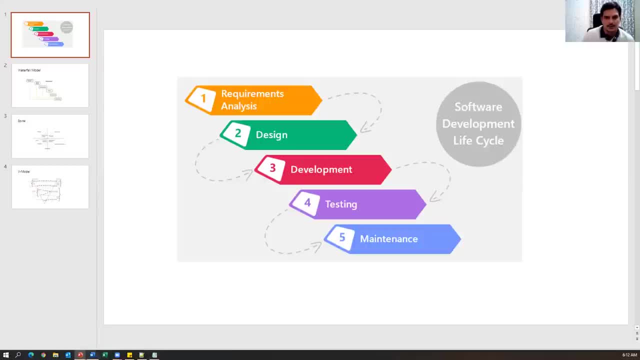 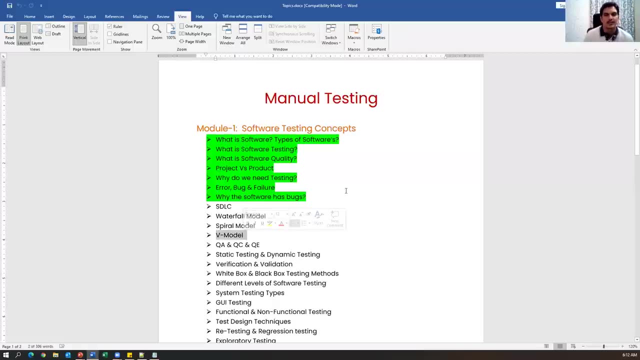 what are those models? so the next topic, what i'm going to discuss, is waterfall model, spiral model, b model. so these are. there are n number of models are there? all these models are comes under sdlc, but i'm just talking about the main models, like previously or traditionally, how the companies 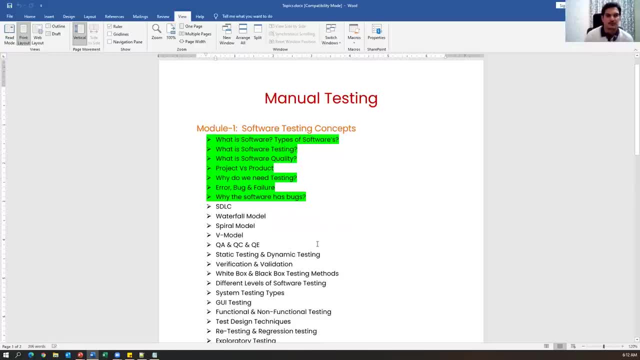 are following, what type of models they are following to develop the software and now what kind of models or companies are following. so i'm just going to explain, like advantages and disadvantages and, interestingly, i'm going to explain the advantages and disadvantages of sdlc. so first of all, what is sdlc? so sdlc is a very, very important model. okay, so we have understood what. 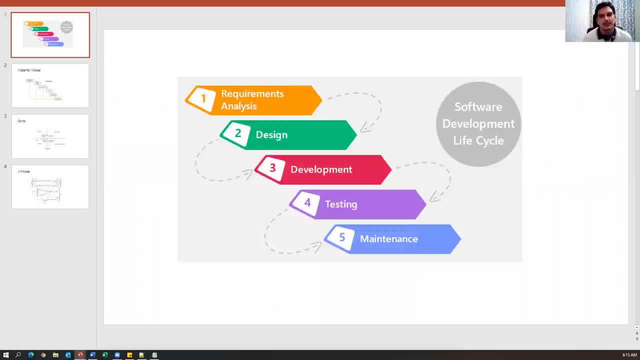 is sdlc. so sdlc is a step-by-step process which we have to follow to deliver the quality product to the customer. now, by using this sdlc, the companies will design their own models- okay, process model, we can simply say process models. so among them, the first and important model is: 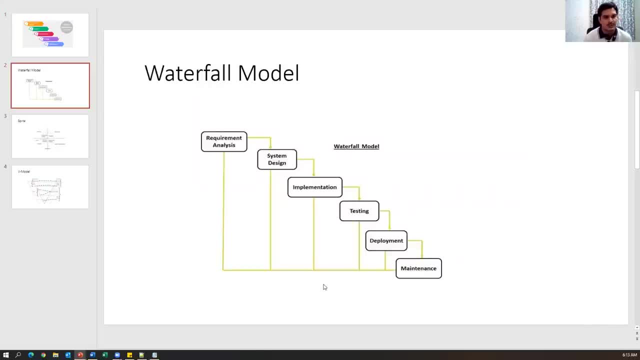 waterfall model. so this is very old and traditional model. so when software industry started the first and initial model, they have started with waterfall model. okay, so very, very old and very traditional model. so waterfall model. this is also called as a linear model. okay, and if i just look at this picture, it seems like a waterfall, like flow, will go down like this: 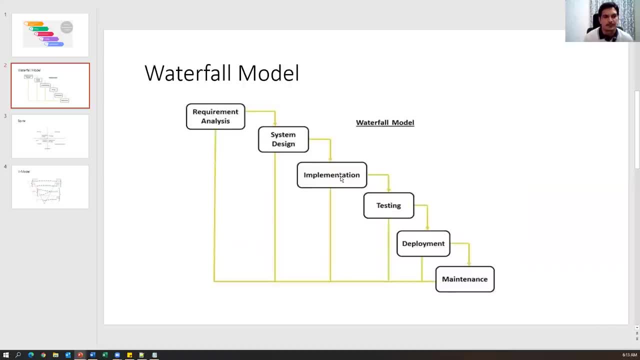 okay, that's the reason we can say: this is a simpler waterfall model. now let us understand what is this model, how the software development will happen in this particular case, particular model, and also we will discuss some of the advantages and disadvantages of this particular model. okay, which is very important for interior perspective, because, even though we are not, 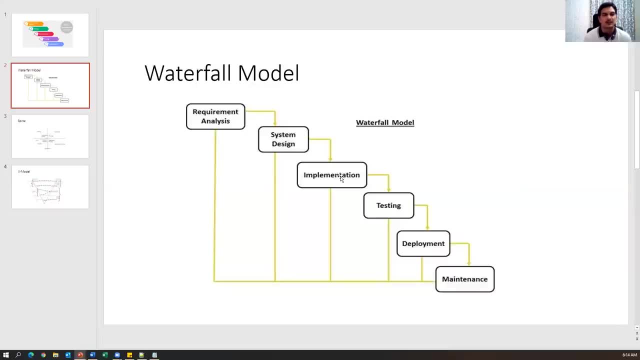 following these models in the nowadays in the company, but we should understand this previously: how models were there and what are the drawbacks we faced and why we are going to implement the new model. so nowadays we are not using these models, but still we have to understand what are. 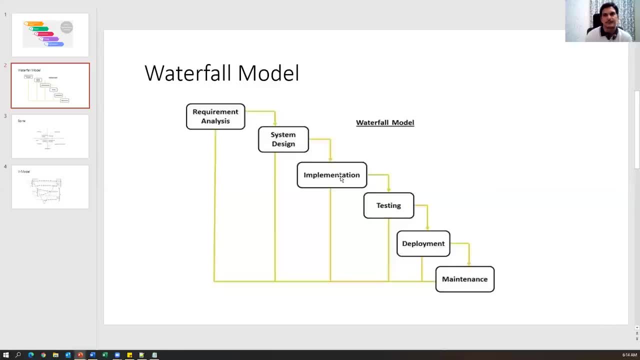 the drawbacks in the model, why we are going for the new models. okay, so all these models again comes under sdlc. the approach is little different, okay, so now let us start waterfall model. so what is waterfall model? this is also one of the model which is comes under sdlc and whatever phases we 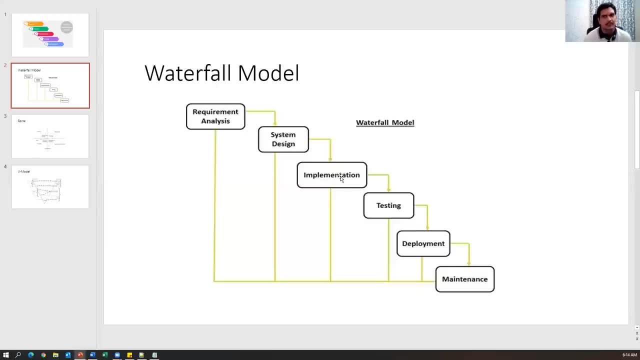 have seen in sdlc. the same phases will be there, but the approach will be different. okay, so again, the waterfall model will start with the requirement analysis. requirement analysis means what? again, we will collect the requirement or we gather the requirement from the customer and we will prepare certain documents. so here the main important is a. 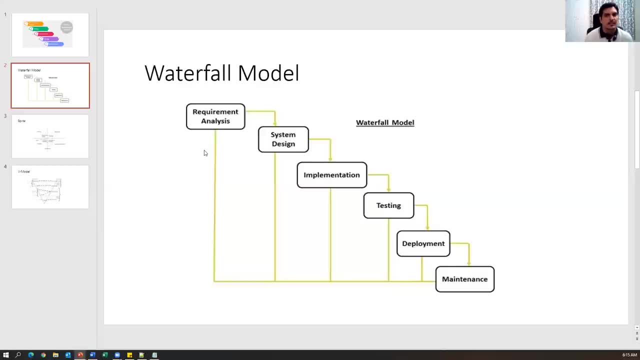 documentation part guys. okay. so documentation in the sense, each and every activity we will document. okay, in this model the documentation will play a very, very important role. so documentation is very, very important. so the first phase of requirement analysis, we will talk to the customers. so we will talk to the customers in the sense: normally business people like project. 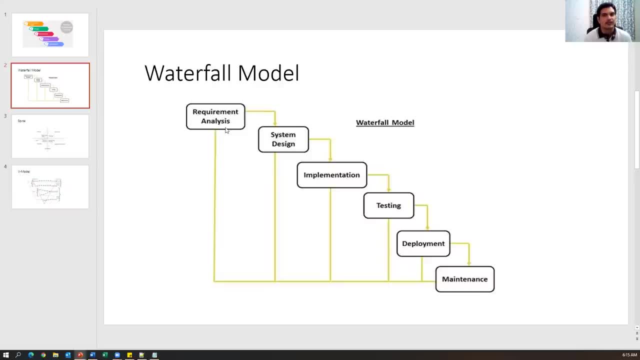 managers, product managers- these people will involve in the communication between customers and companies. okay, so they will collect the requirements from the customer and once they get the requirements they prepare some kind of document that is called srs document. okay, software requirement specification document. so in that document they will document every. 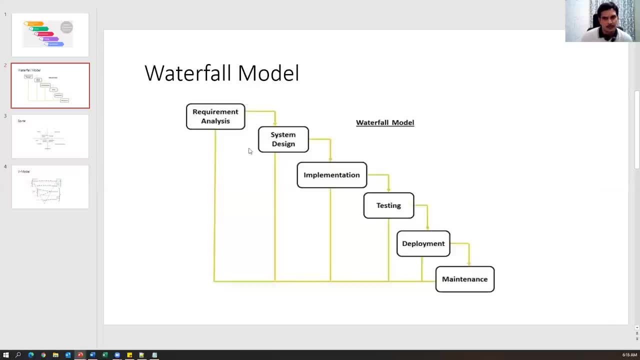 requirement from the customer. so once the document is created, then system design will start. so what is system design means? whatever the documents we prepared during requirement analysis, based on the document, the designers will be there. so the designer says again the different team. so those people will design the software and they will prepare some high level design. we can say hld and 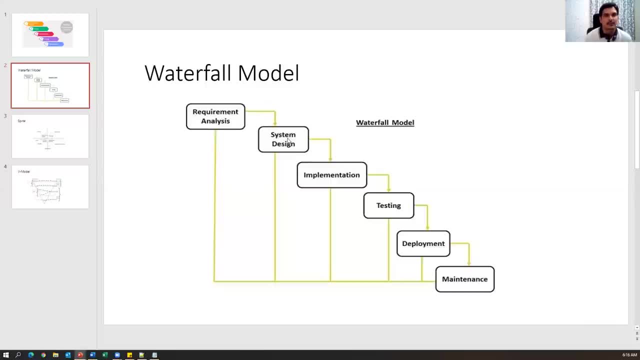 low level design, like: basically, they will design the software and they will prepare the software. so they will divide the entire requirement into high level modules and low level modules, the small pieces of softwares, and finally we'll integrate them. so the second phase is the design phase in. 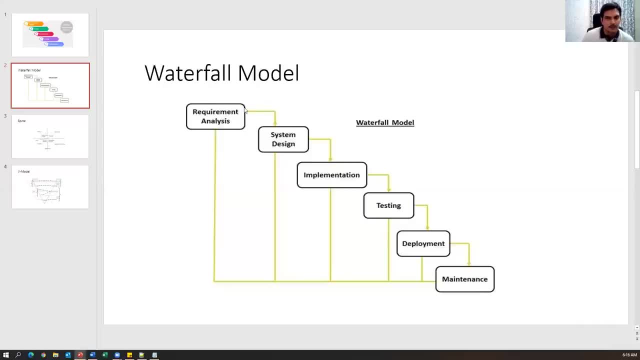 the design phase. what happens? based on the requirement document, the designers will prepare the design document. so once the design phase is completed, then developers will develop or implement the software by based on the design documents, because, as a developer, if you want to develop a software, i need some input. from where i'll get the input? so, based on the design i have, 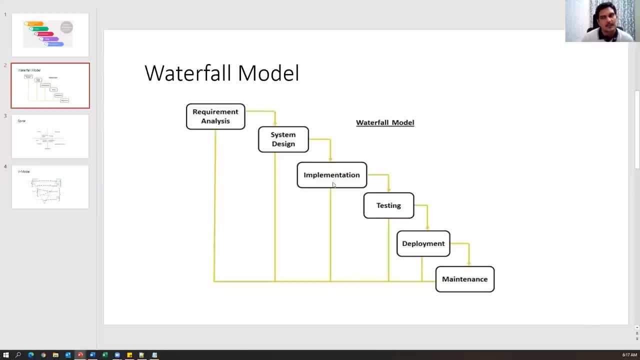 to develop the software. so the next phase is implementation or coding phase. so, based on the design document, coding or implementation will start after completion of implementation, implementation in the sense of development. so after completion of implementation or development, now the testing phase will start. so in the testing phase, what you will do is the tester. 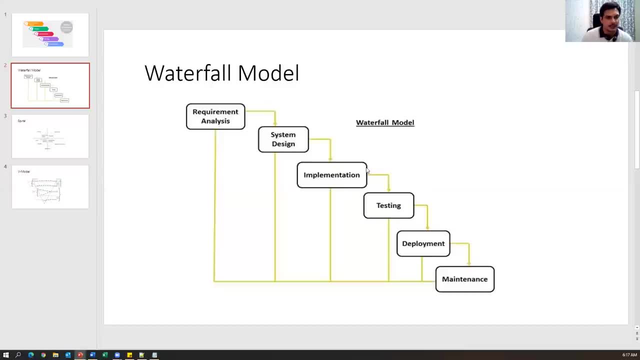 will test the software after completion of development and once the testing is completed, then we will deploy the software on the customer environment. so deployment is nothing, but will install the software in the customer environment and then they'll start using the software. so that is a maintenance phase. so this is all about waterfall model. now, if i just look, 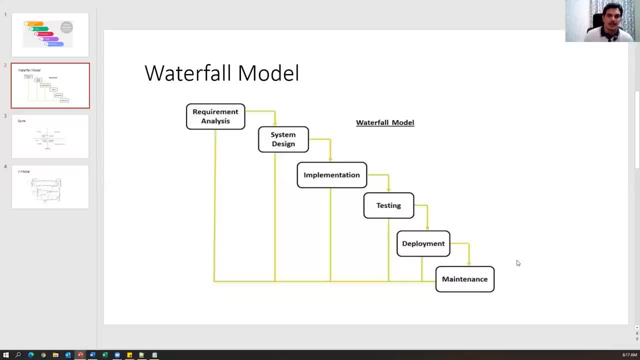 at this waterfall model. just understand the behavior of it. okay, so one of the four will be the demosged or the nonvanished. so as soon as it finishes, we'll do the proofreading. okay, so you can see that we ultimately got three. we're going to send that and then each 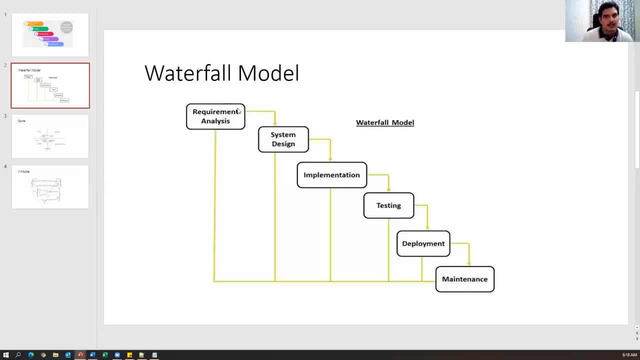 of the vêrts printed out, the data which you can purchase by suitable developer and then. so this死 rated is basically the time frame of every time frame, time something starts and goes out. so, for instance, here you look at the software which is being produced, the 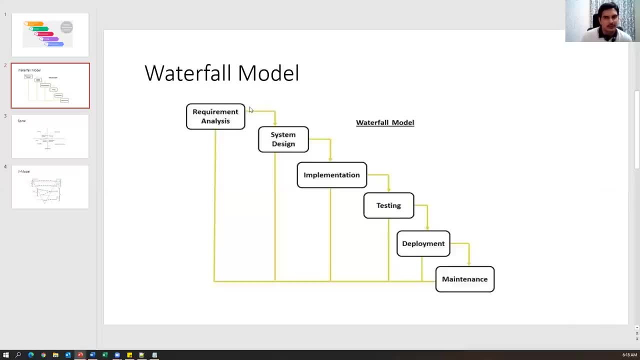 For example, when I take a requirement analysis phase, what is the input for this- The customer requirements- And what is the outcome of this phase? Requirement specification document And the requirement specification document will be the input for the system design phase, And what is the outcome of system design. 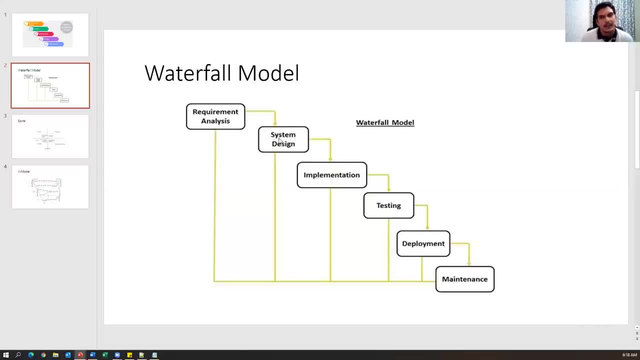 Design documents. They will prepare some design documents And based on the design documents- so design documents- will be the input for the implementation phase And what is the outcome of implementation phase Code. So, based on the design, the developers will implement the code or programs or software. 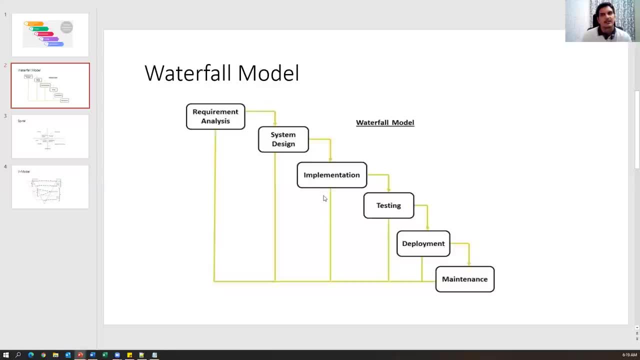 And once the outcome is software and once they deliver the software and testing will start. what is the input for testing The software itself? Once the developer is provided the software for the testing team, testing will conduct. After completion of testing, what is the outcome? 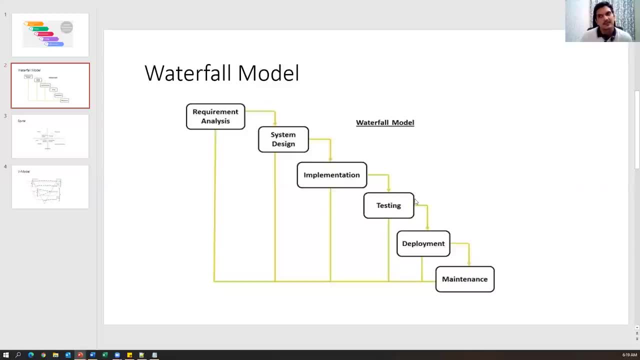 Like test cases, test plan, test results. These are the outcome of the testing phase. These are the documents which we have to prepare as a tester And the deployment will happen. So in the deployment phase we will prepare some documentation like installation documentation. 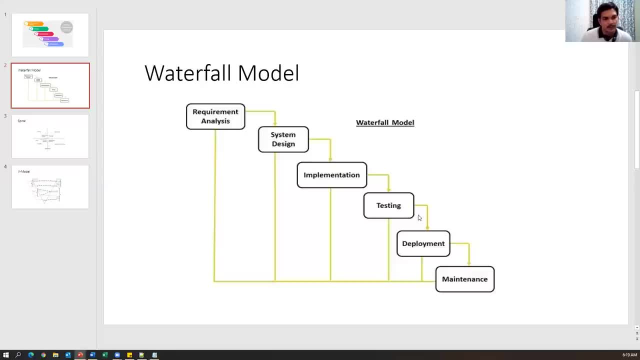 and functional flows, how the software will work like user manual. So these things will be provided to the customer And based on that, the customer will start using the software. So each and every phase is having certain input or it will give some outcome. 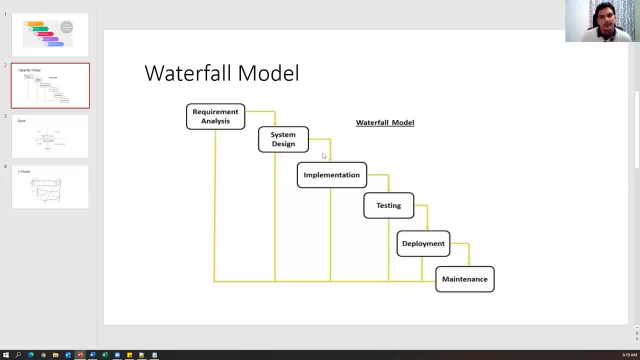 That is the first point. The second point is suppose if I want to start a design, right until unless the requirement analysis is completed, I cannot start the design. What does that mean? Every phase is depends on the previous phase of the model. 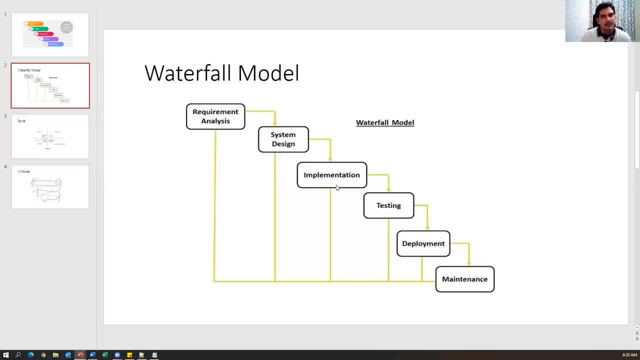 For example, design is depend on the requirements, Implementation is depends on the design. Testing is depends on the implementation. Deployment is depends on the testing. So each phase is depends on the previous phase. Until, unless we completed this phase, we cannot go to the next phase. 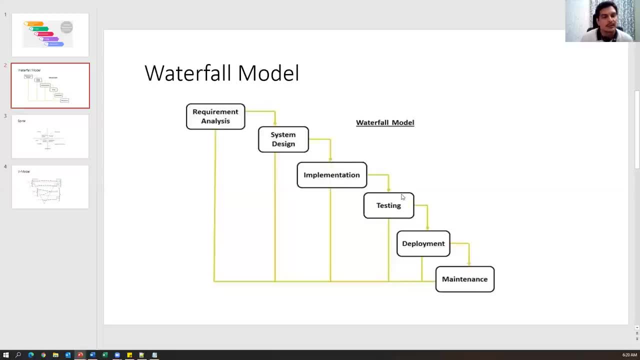 Until. unless we completed that implementation, we cannot go with the testing part. So every phase is depend on previous phase. Okay, so this is a behavior of the waterfall model. So this is very old and traditional model. The companies were following the olden days. 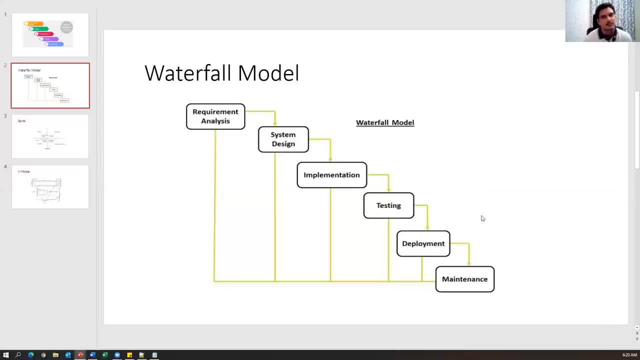 But now, what is the advantage and drawback? So, because there are so many other models also came in the market, but why we move to the another model? So that we need to understand. So what are the advantages and disadvantages of water model that we will discuss now? 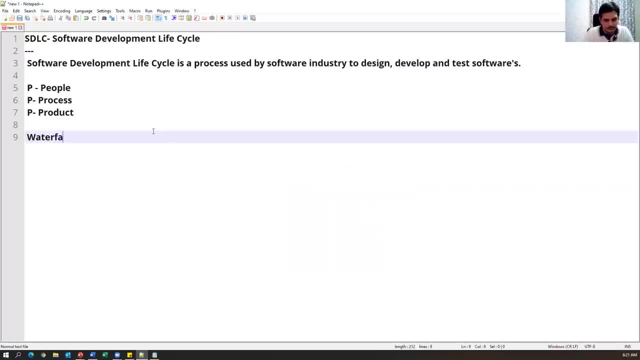 Now come back to the notes, Waterfall model. So if you have any queries, guys, please put me in the chat window. I'll answer this. Okay, so waterfall model, Just a moment. Yeah, so waterfall model advantages. What are the advantages and disadvantages of waterfall model? 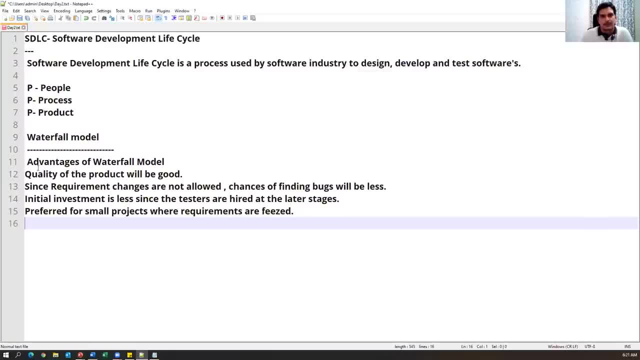 So let me just write some advantages here. So waterfall advantages, the first advantage, one, two and this is three and four. So let us start discussing what are the advantages of waterfall model. If I just look at this, the quality of the product will be good. 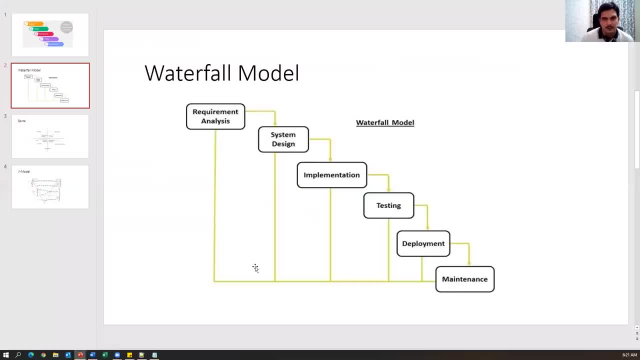 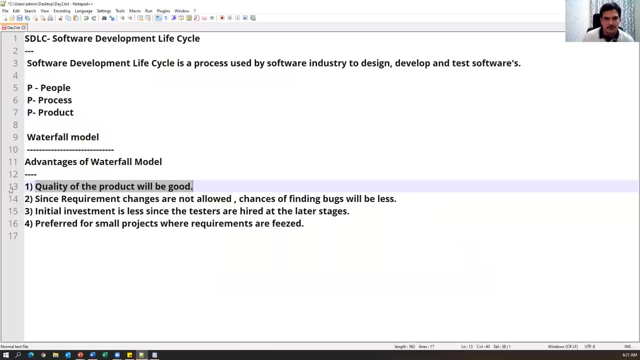 So because in waterfall model- if I just look at this waterfall model- normally this model will be prepared for long term projects. Okay, So here the first point is. the first point is quality of the product will be good. So why the quality of the product will be good? 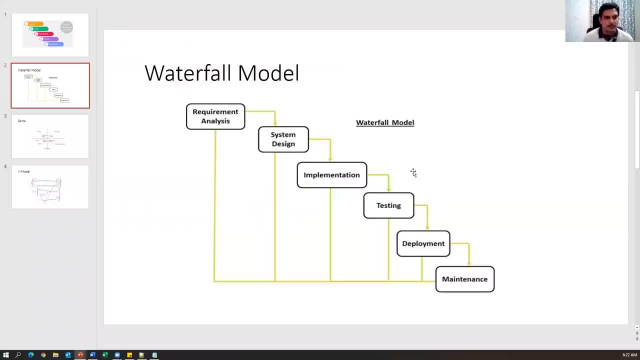 Because every phase we have a detailed documentation. So whatever activity we do, we will document it, So that will be very, very clear for the people who are involved in the design phase, development phase and testing phase. So, finally, which will lead to the quality product, because every, each and every phase we have a clear documentation, so that 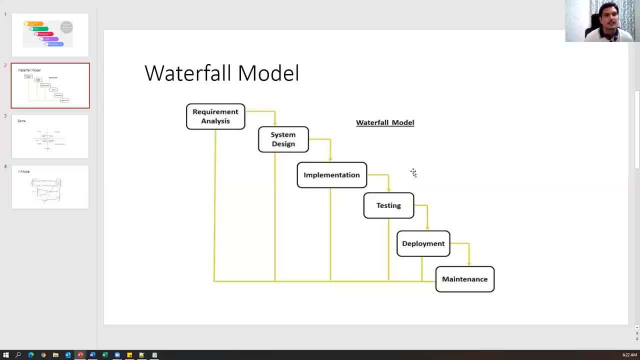 we can also develop and test the software And finally we will be able to release a quality product to the customer. Okay, So that is the first point of waterfall model. The advantage of waterfall model is quality of the product will be very, very good. 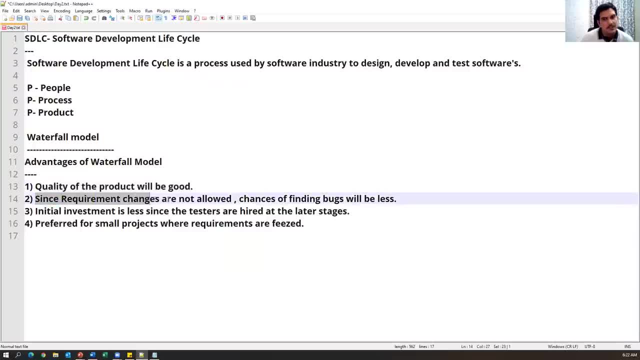 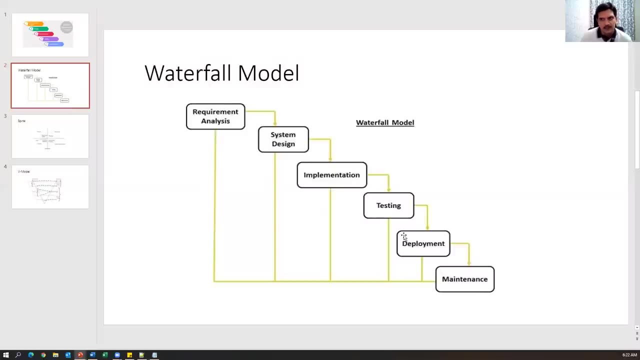 The next advantage is, since the requirement changes are not allowed, chances of finding bugs will be less. And one more important point: guys, suppose we got some requirement from the customer and we have started design and we have started coding somewhere. we are in this particular phases. 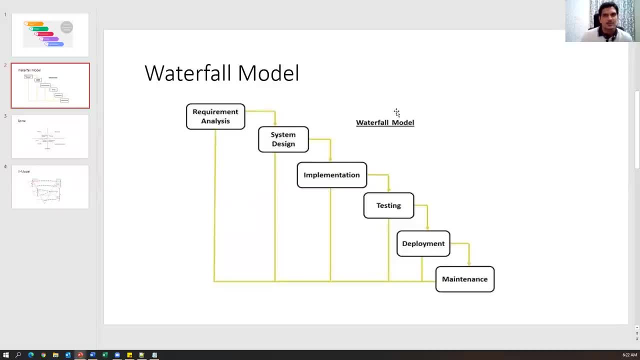 But again customers came back and asked us to change something, asked us to change some requirement. Okay, That is not possible in waterfall model. So frequently changing the requirements we cannot accommodate in waterfall model. This is a fixed model. So once you've completed requirement analysis and design, then coding testing, deployment will go on like this: 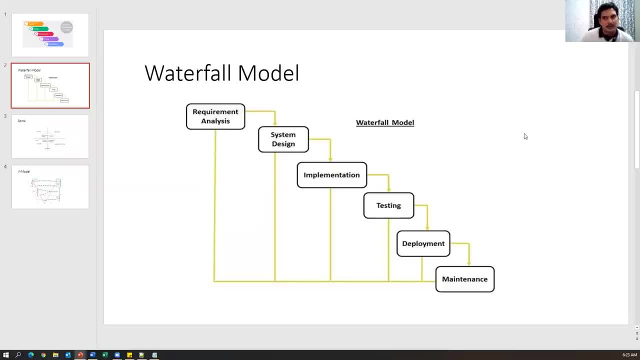 We cannot allow the new design, We cannot allow the new design, We cannot allow the new design, We cannot allow the new requirements or we cannot change the requirement in the middle of this phase, because everything will be phased, Everything will be clear, cut documentation. 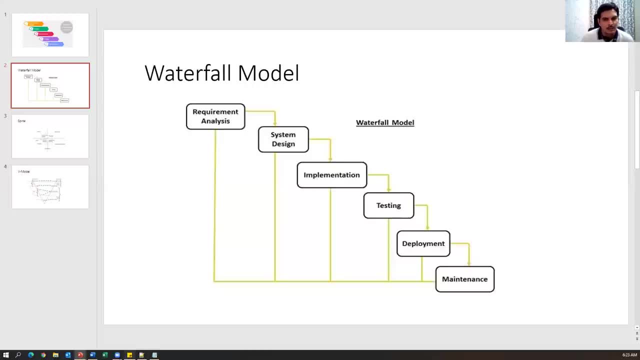 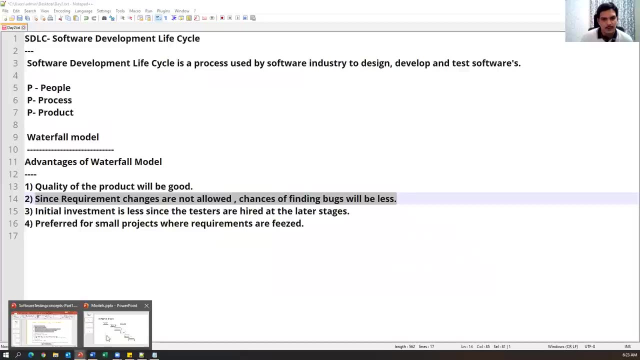 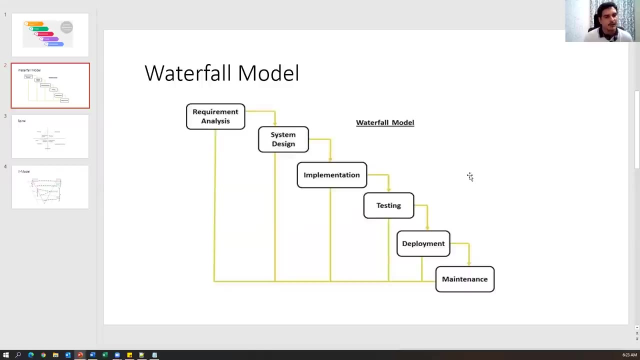 So the new requirements we cannot accommodate in this model. So because of that reason chances of finding bugs will be very less. And if you keep on changing the requirement, so if you're keeping on, if you keep on changing the design or coding, definitely there will be chances to get a number of bugs. 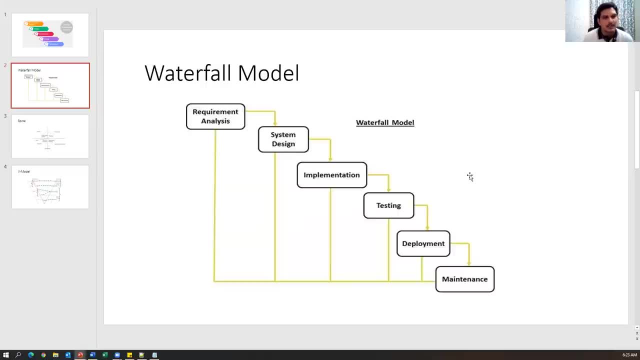 But here everything will be clear. The document, The documentation will be clear and we are not allowing to implement the new requirements in the middle of the process. So there are less chances of bugs we have in this model. That is another advantage. 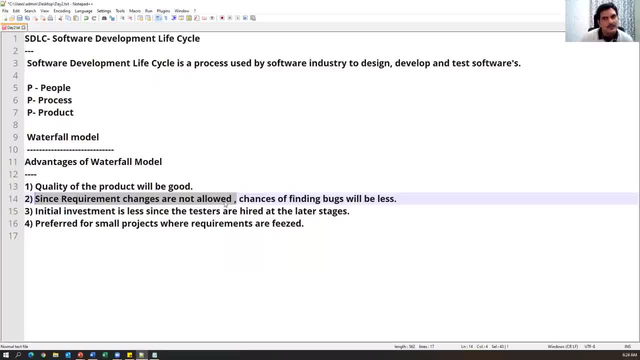 Since the requirement changes are not allowed, chances of finding bugs will be very, very less. So that is one of the advantages of waterfall model. So the next advantage is initial investment is less, since the testers are high at the latest Stages. 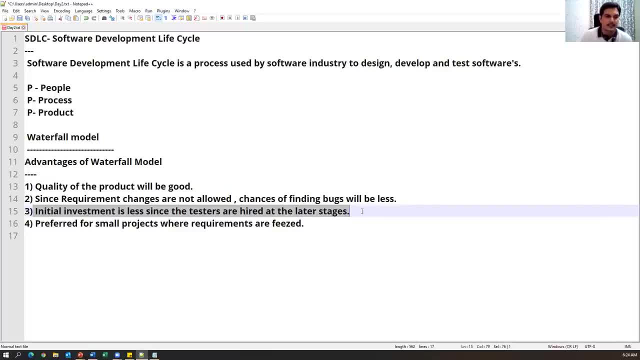 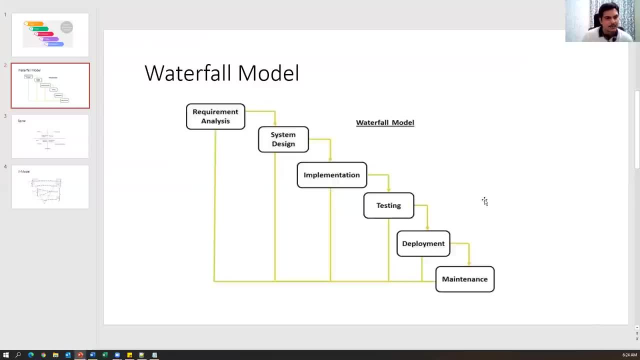 Initial investment is less, since the testers are hiding the latest stages. What does that mean? If I just look at this model once again, each and every phase is having different teams, like: requirement analysis will be different team I'm in. different team. design will be different team coding or development is a different team. 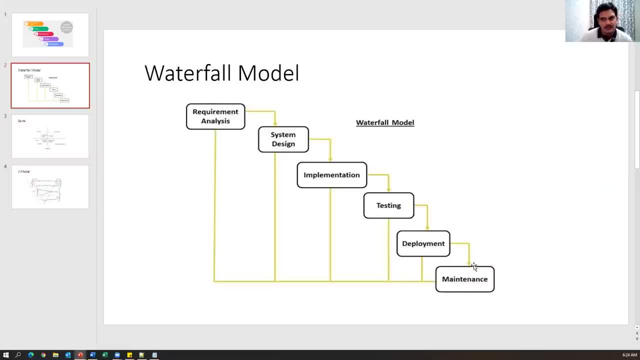 Testing is a different team And at the initial stage of software development process we don't need all the team members right Initial stage. We need only business people or like Providers, product managers and project managers. then the designers we need after completion of this phase. 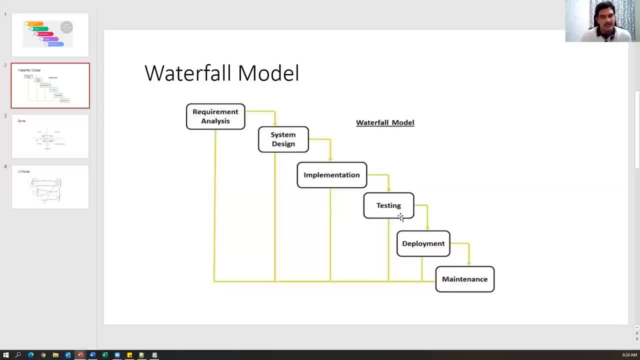 the programmers or developers are needed, and then testers we can recruit. until unless we completed these phases, we don't need testers, right? so investment is very less. that is the point we need to discuss here. initial investment is less because we no need to hire the people at the 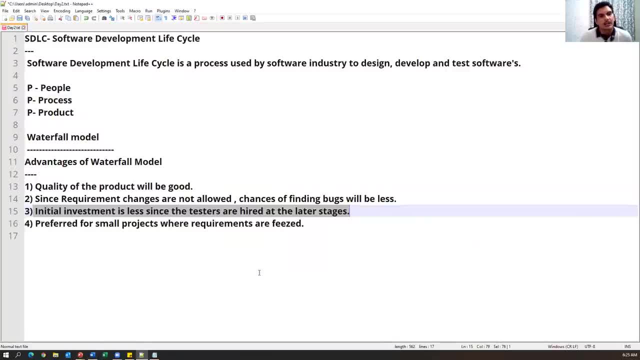 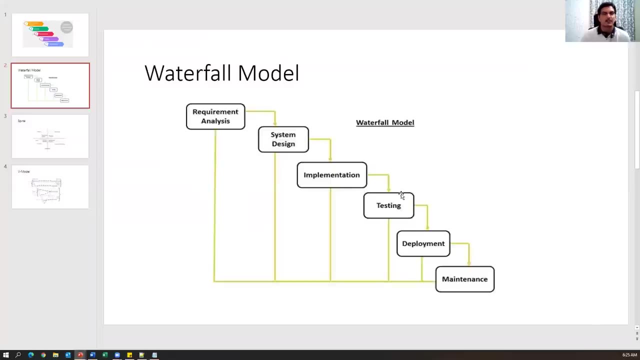 beginning stage. so whenever we need those people, we can recruit them, we can hire them. so that is the reason initial requirement is less, since the testers are hired at the later stages, after completion of requirement analysis, design, implementation. then testers come into picture. so in this particular time we can hire the tester. so initial investment is very, very less. that is. 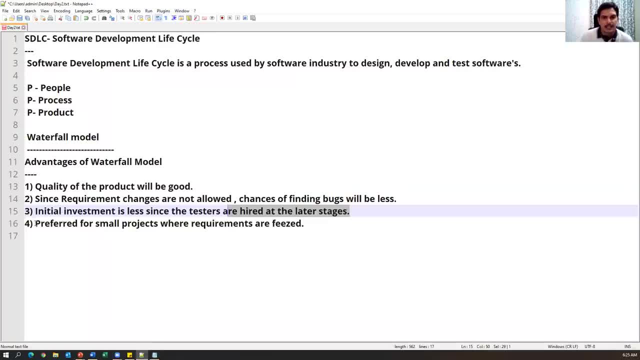 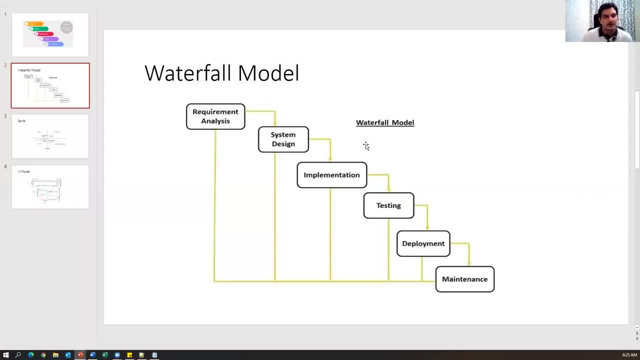 one more advantage of waterfall model, and the last advantage- is preferred for small projects where requirements are freezed. especially, this model will be preferred for small projects where the requirements are freezed, because every uh, every phase, we have a static documentation and everything. every phase that documents will be freezed. we cannot modify the. 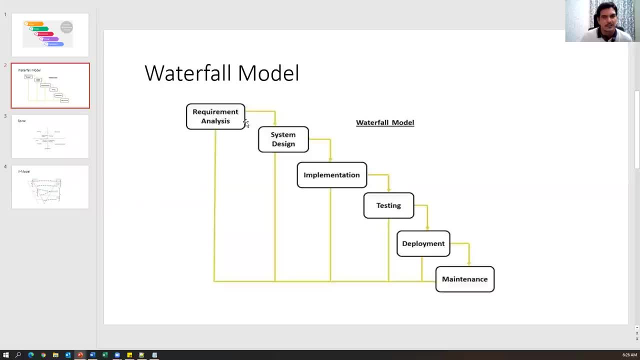 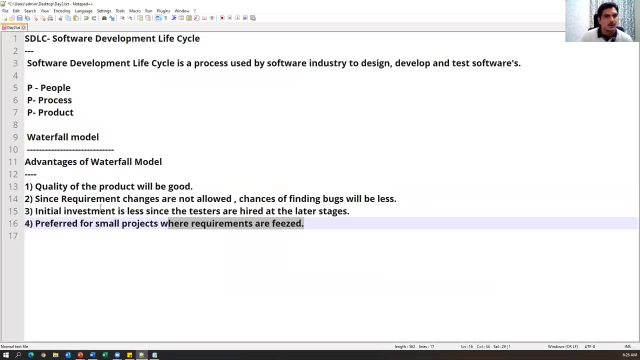 document. again, we cannot go back and modify the documents. so if there is any requirement which are very static, which are not dynamic requirement or which are not changing very frequently, in those cases we can go and prefer this model. okay, so these are the few advantages of waterfall model. 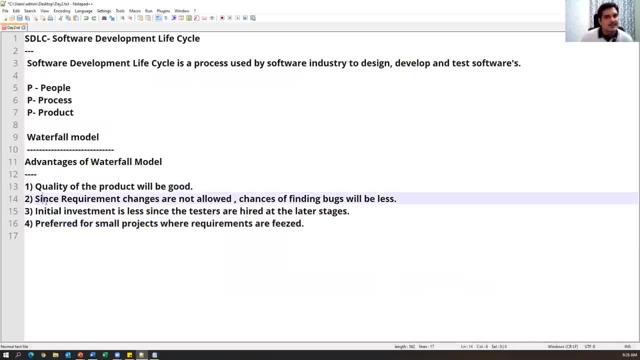 quality of the product will be very good and since the requirement changes are not allowed, so chances of finding bugs will be very less. initial requirement is less, since the testers are hired at the larger later stages and preferred for small projects where requirements are freezed. so these are the few advantages of waterfall model. now let us discuss drawbacks or disadvantages of. 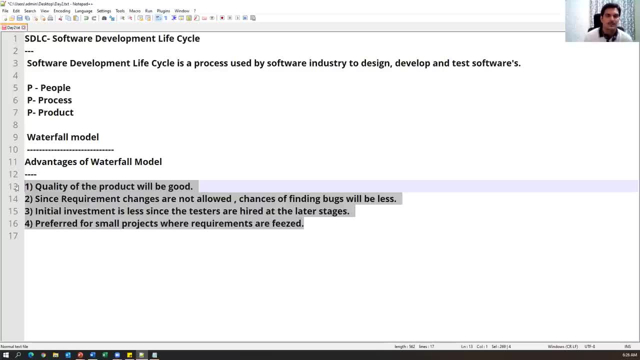 waterfall model because, based on the drop drawbacks or disadvantages, the drawbacks of waterfall model, new models are coming into market because so every, every model, they are having their own disadvantages and then people are using a different type of models, so even waterfall model also having disadvantages or drawbacks. so now we will see what are the drawbacks of waterfall model, or 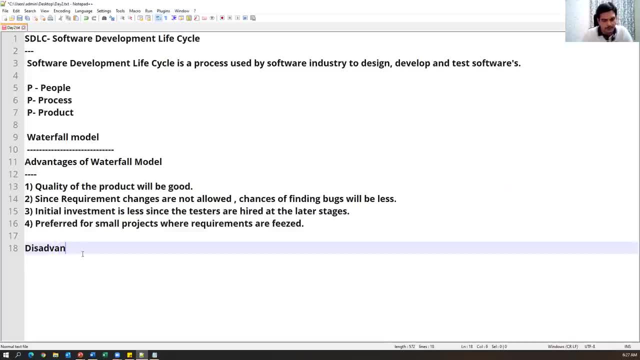 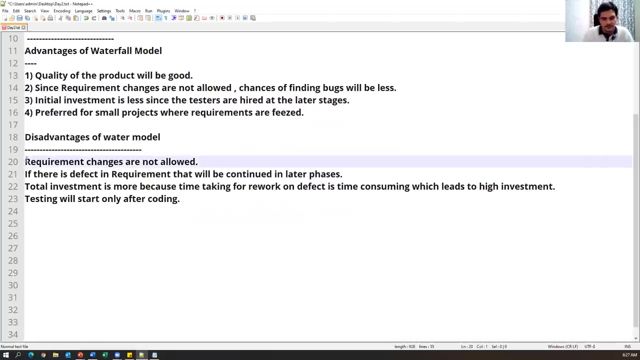 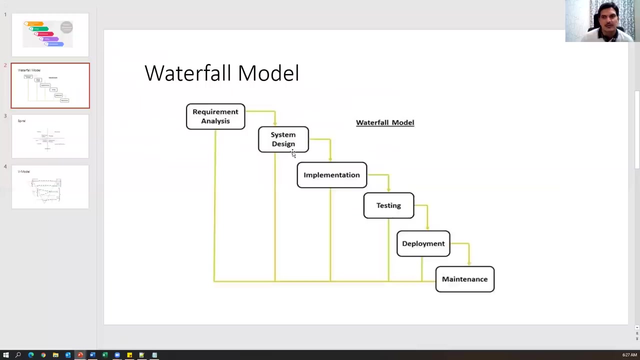 we can say disadvantages of a waterfall model, disadvantages of waterfall model. okay, so what are the disadvantages of waterfall model? so let me write some notes here, okay. so let us look at this. the first point: requirement changes are not allowed. suppose the customer is given some initial requirement here and we have started design and implementation. 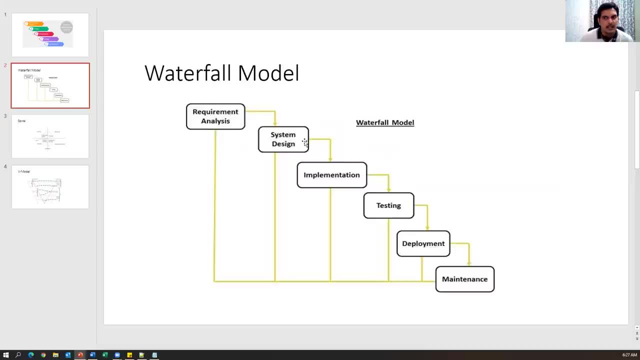 we are in implementation or testing phase. at that time again customer came back and asked us to change some requirement or asked us to implement some new requirement. so that kind of requirements we cannot accommodate in the middle of the development process. okay, we cannot accommodate the frequent changes requirements we cannot accommodate in your software development process. so that is a one of 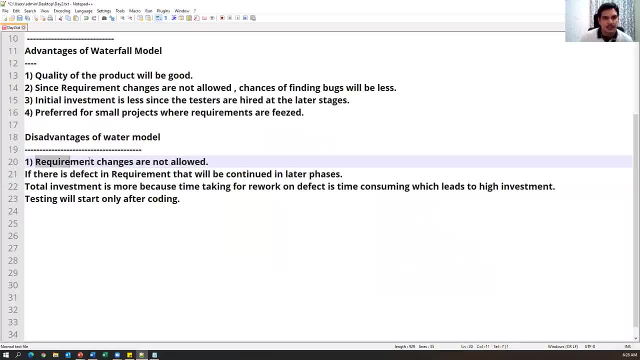 the disadvantage of waterfall model. so requirement changes are not allowed because this is a fixed model. once the phase is completed, once we move on to the next phase, we cannot go back to the previous phases. okay, and the requirement changes are not allowed in the middle of software development process. 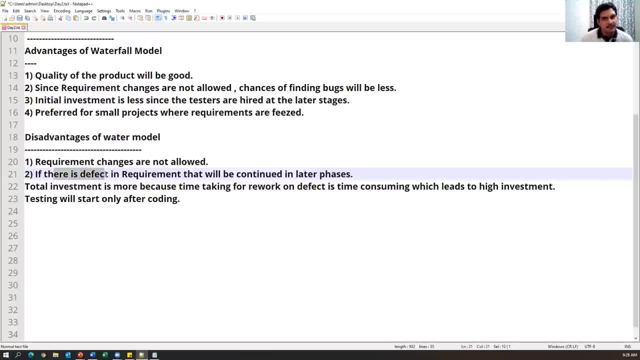 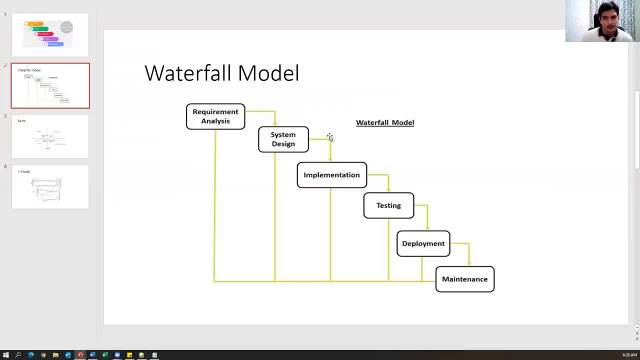 and the next drawback is, if there is a defect in requirement, that will be continued in the later phases. so this is one of the important point, guys: if there is a defect in the requirement, that will be continued in the later phases. so what does it mean, suppose? 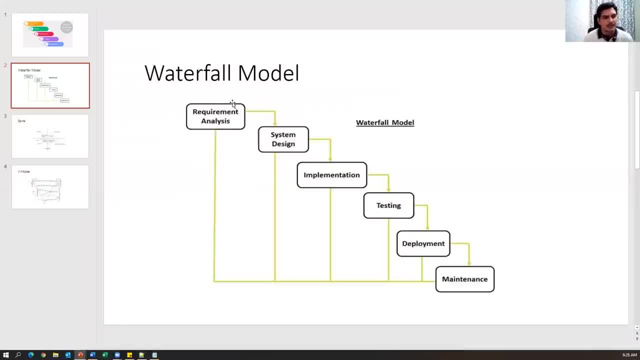 in the requirement analysis phase we have collected some requirements. suppose if there is any problem or any mistake in the requirement right, that will be again continued in the next phases, because requirement based on the requirement document design will happen and the same mistake will be continued in the design. if the design is wrong, coding will be wrong if the coding is wrong. 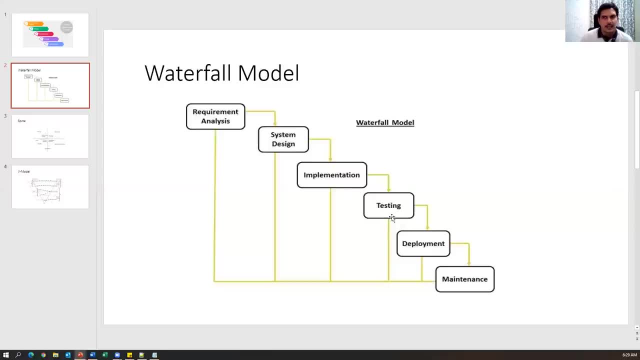 testing will be wrong and we cannot find those bugs. and if the testing is again, we will miss the bug again. that bug will come under meaning again. that bug will be faced by the customer. so if there is any mistake in one phase, that will continue to the next phases. okay, so that is one. 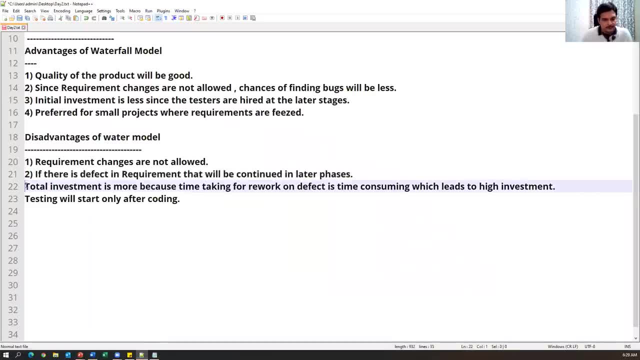 of the drawback. and the next point is: total investment is more, because time taking for rework on defect is time consuming, which leads to higher investment. so what does that mean? total investment is more. total investment is more why? because, suppose, if you find any defect in the 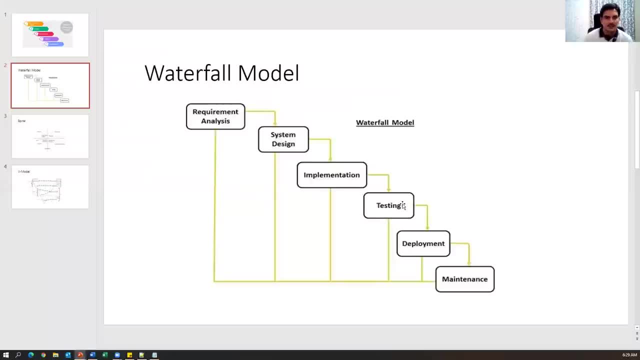 middle of some phase, like suppose in the testing phase we found some defect. and when i found defect in the testing phase, what we have to do? we have to correct the defect in the coding level and again the same defect we have to correct at the design level. again we have to correct in the. 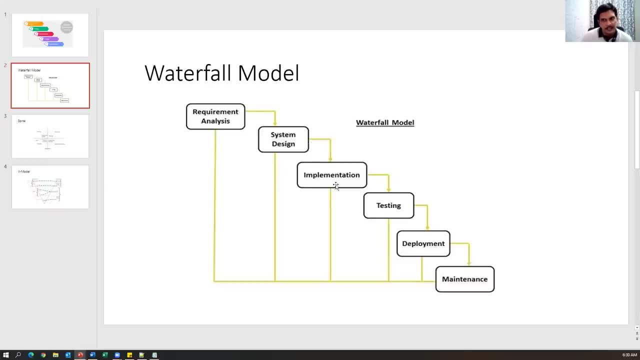 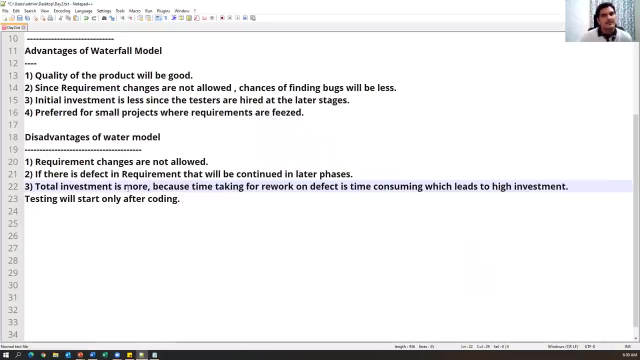 requirement level. so if you find any defect in any other, any of any of these phases, we have to go back to the previous phase and we need to modify the document accordingly. so that is again more cost, so that total investment will be more. we have to invest a lot if you want to do some. 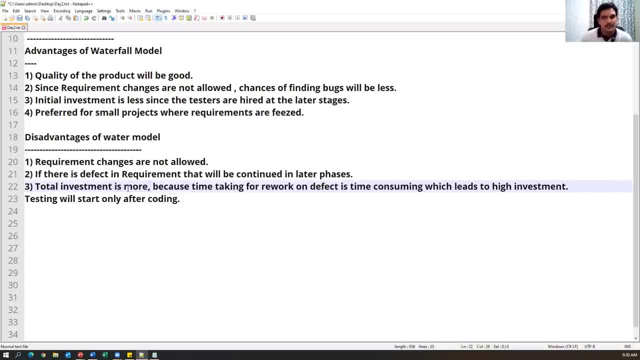 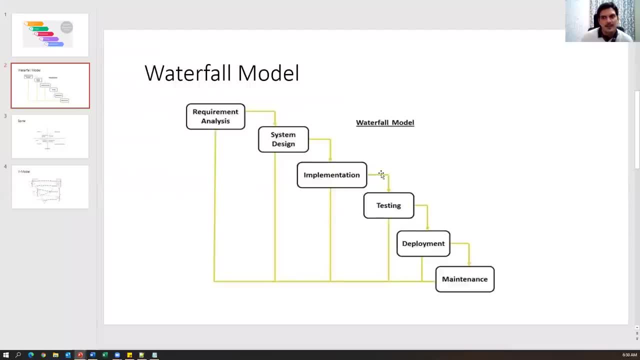 rework. we have to invest a lot, so that will cause the rework. right, if you find any defect in some phase, we need to change. suppose in the testing phase we found some defects, accordingly, we have to change the code. the developer should work on that. that is again rework and again the designers. 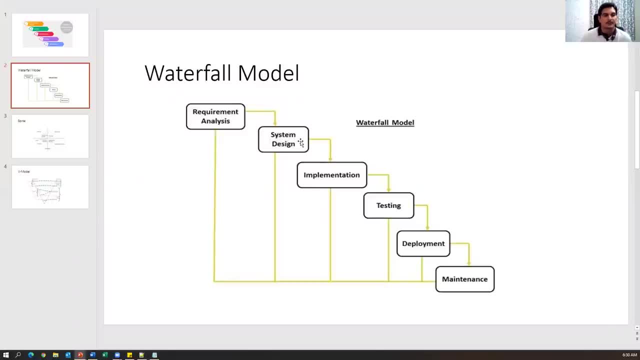 will change the document accordingly. so that is, that is also a rework and we have to change the requirement. we have to correct the requirement that is also reworked. so whenever you do some rework, the cost will be more okay. so that is a another disadvantage of 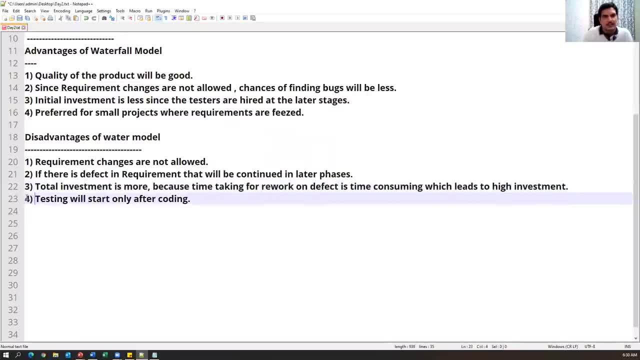 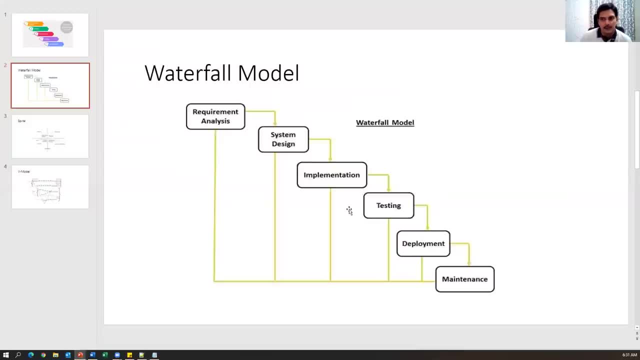 waterfall model. and the last one is: testing will start only after coding. testing will start only after coding. what does that mean? we have only one phase of testing. so after completion of three phases, here we have a testing. so if we find any defects in the testing phase, accordingly, we have to change the code or implementation, we have to change the. 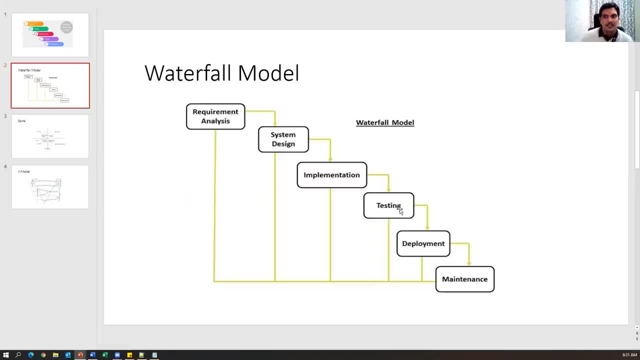 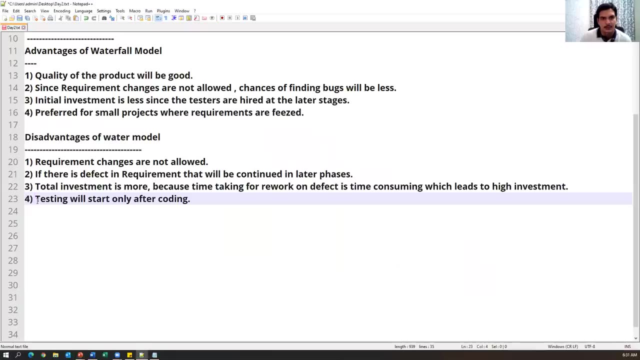 to change the requirements. so we have only one phase of testing here. we don't have a different phases of testing. so the chances of bugs will be more. so that is another topic. so testing will start only after coding. so testing team will not be involved from the beginning of the software. 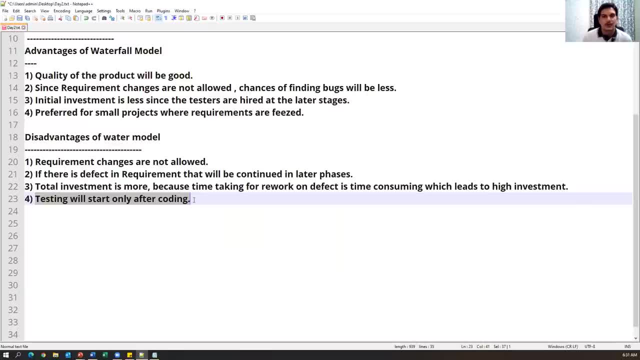 development process. so the testers will be involved only in one phase: after completion, after completion of the coding part. okay, so these are the disadvantages of waterfall model. so advantages and disadvantages. okay, so this is very old and traditional model. the companies are falling, so initial days of it industry started long back. okay, so now, based on these drawbacks, 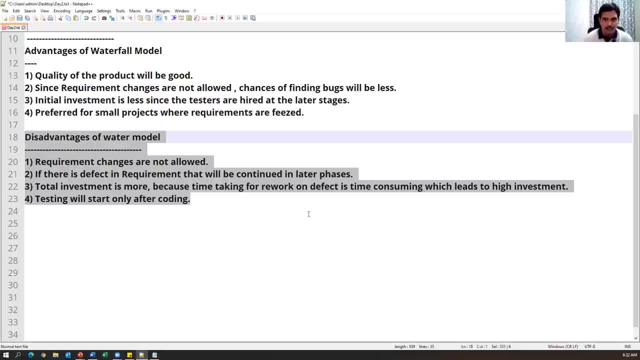 the new models are coming up in the market. okay, so because the drawback series, requirement changes are not allowed, because this is a common right. if the customer is given some requirement in the middle of software development process, again customer come back and ask the changes, some requirement, or they may give some new requirement. 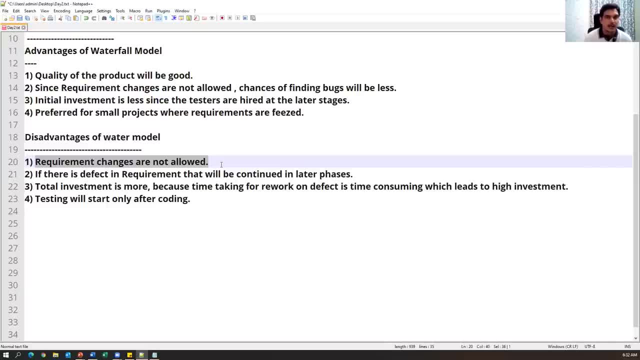 so these changes are commonly there. so we should able to accommodate those changes in our software, right. and here we have only one phase of testing. if you find any defects in the previous phases, that will continue to the next phases. so that is also another biggest problem, right so to overcome. 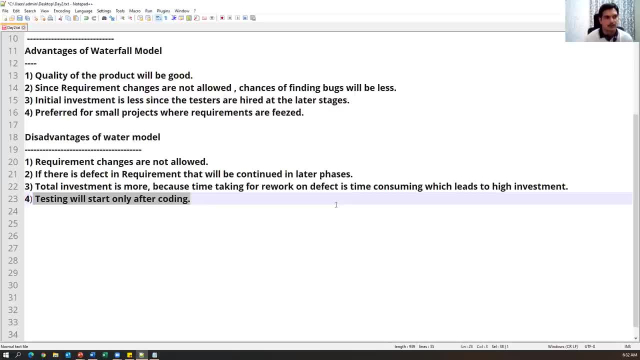 these particular problems. we have another model called. they have come to the another model called, which is also called iterative model. okay, so now let us start with spiral model. this is another sdlc model. this is another type of sdac model. so are you guys able to follow? 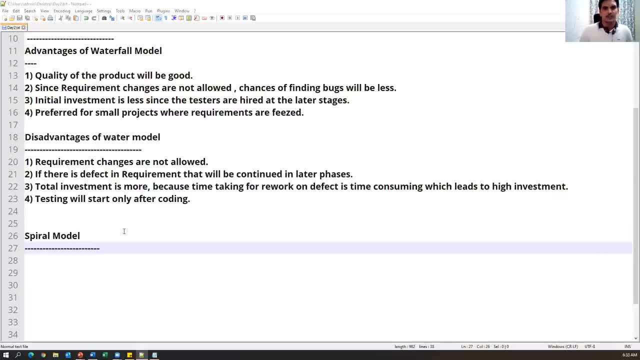 please confirm in the chart window everyone. so this is a spiral model. so next we are going to discuss about spiral model. great, so spiral model. so what is spiral model look like? so let me just show the picture first. so let me just show the picture first. so let me just show the picture first. 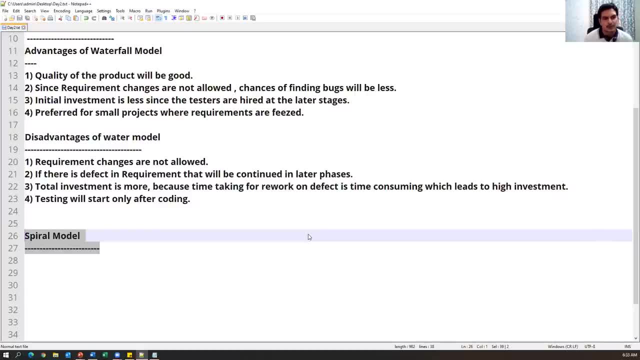 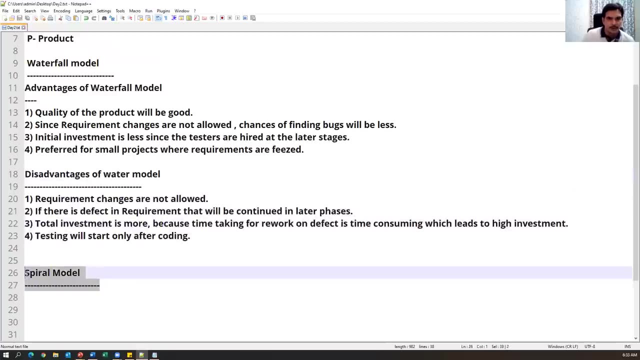 and then let us try to understand so how spiral model works. and again, the spiral model is also having some number of advantages and disadvantages. okay, so to overcome the problems from, or overcome the drawbacks from, waterfall model, spiral model is implemented. now let us see how the spiral model looks like and what are the advantages and disadvantages. now let us. 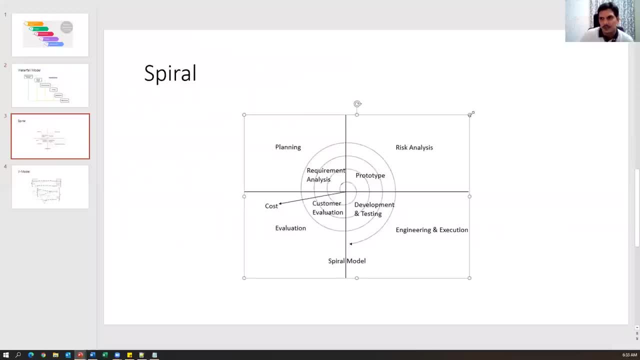 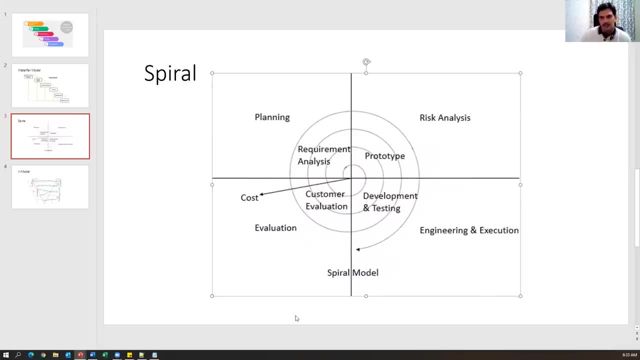 start about spiral model. so if we just look at this picture, this is a picture of spiral. it seems very similar to the spiral shape. okay, if you see the diagram, it is a spiral. so this is a picture of spiral models. okay, now let us understand how this spiral model works and then we will discuss. 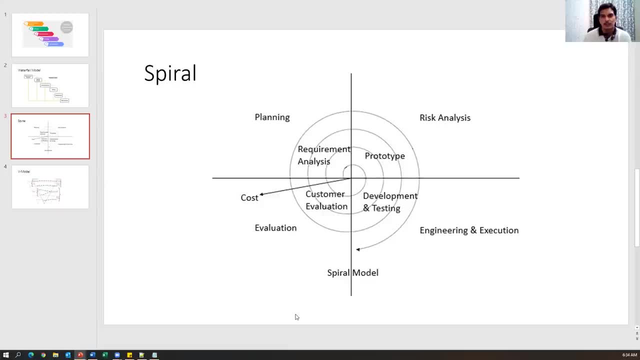 advantages and disadvantages. so here, if i just look at here some terminology like risk analysis, engineering and execution evaluation, planning, so these are all normal terms like requirement analysis, design, coding, testing, it is the same, okay. so here, uh, planning, planning in the sense, requirement analysis. okay, planning in the sense is a simpler requirement analysis. let me just write the notes. 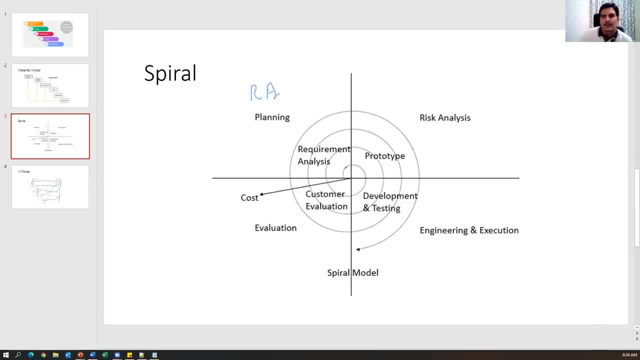 so here, planning in the sense requirement analysis, and after planning, after requirement analysis, we will design the code. so again, risk analysis comes under like after completion of requirement analysis. in the risk analysis we will plan like uh, how much risk is involved, like how many developers required, how. 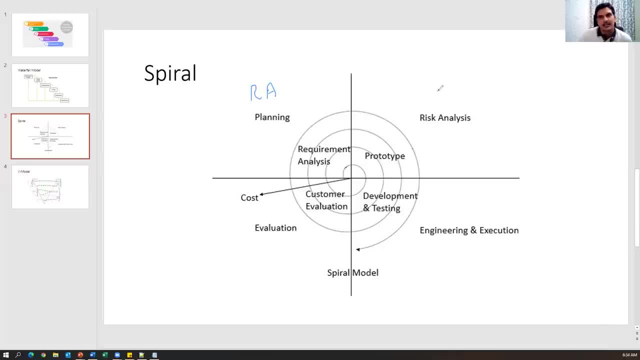 How many testers are required, we will analyze in detail. So that is comes under risk analysis. So these two basically comes under requirement analysis and everything. And engineering and execution means what it is basically design and development phase. So this particular area which is talking about design and development, 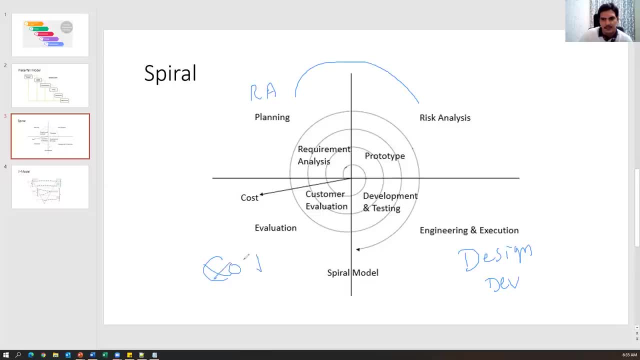 And this particular area is talking about the sorry testing, okay, testing phase. This is the four parts we have. The first part is a requirement analysis phase, So these two and the design and testing requirement, design and testing. So design and development comes under one phase here. 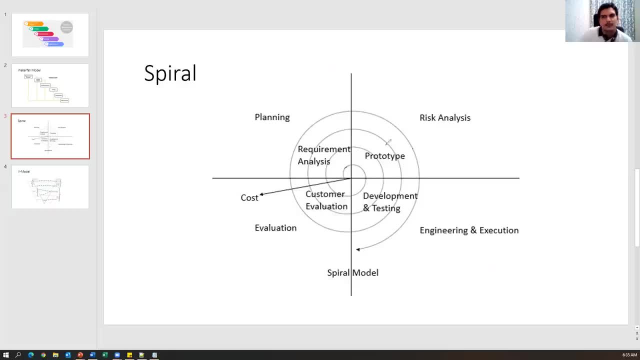 So let us try to understand this, how this spiral model works. So the first part- again same SDLC process- will be there. So first, requirement analysis, or collect the requirements and the design, coding, testing, maintenance. So these phases are common. 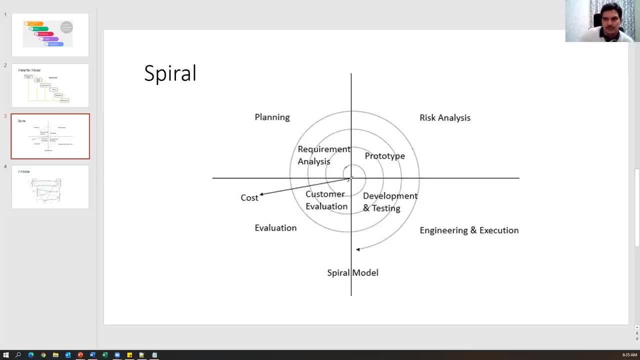 So here the terminology is different, the process is same. So initial level, first we will estimate some cost and we'll do some planning. So this particular part, whatever you can see here, this part is a planning- means requirement analysis and understanding the risk analysis and budget cost. everything we will think. 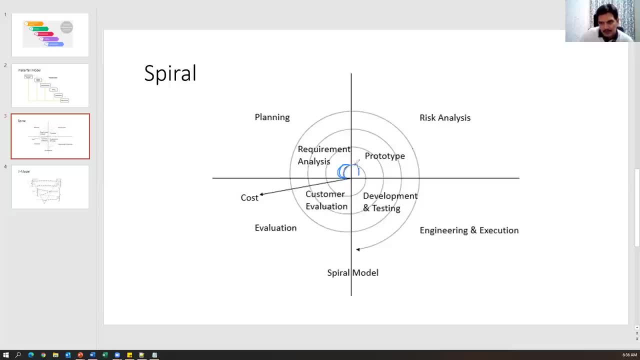 about. So that is the first phase. After completion of this, development and coding will start. So development and testing. So here, development and testing, And then we will release the software to the customer customer evaluation. So one cycle is completed like this. 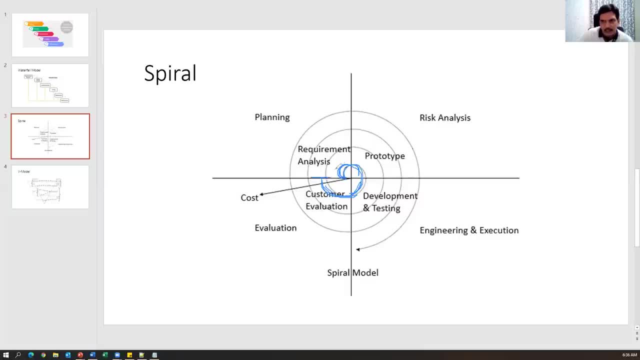 Once you reach here in one cycle, requirement analysis, design, coding, testing and maintenance. So one cycle will be having all five phases And once we reach it here, we deliver one software to the customer. one version of the software we will deliver to the customer. 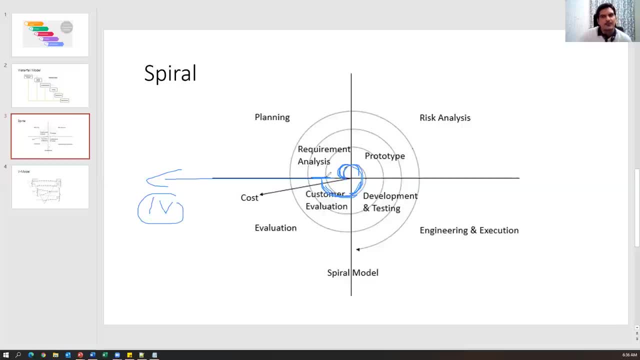 Again, on top of this, the customer will give you a few more requirements. So the customer will give you a few more requirements. So here we will deliver one software to the customer. Then, on top of this software again, we do requirement analysis, design, testing and 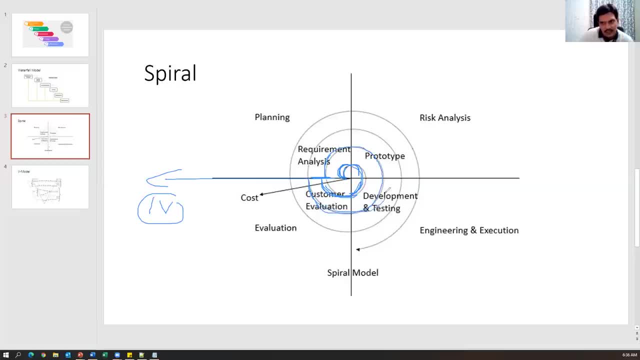 coding in the second cycle. And again in the second cycle we will release another software to the customer, let us say version number two, And again we will take the new requirements. Again we will implement the new requirements on top of existing software. again, requirement: 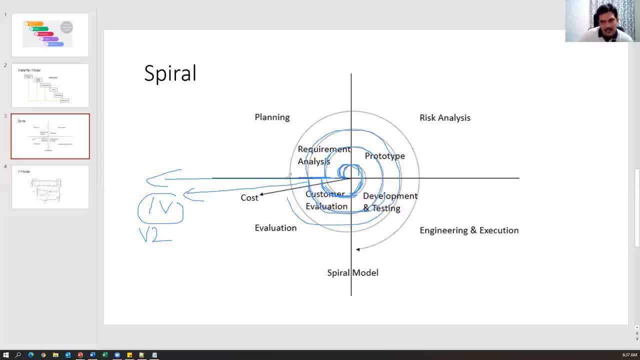 design, coding testing will start and we will release another version of software in the next cycle. that is version number three. So in every cycle we will follow the SDLC process. in every cycle we will follow we do requirement analysis, design, coding, testing and maintenance. 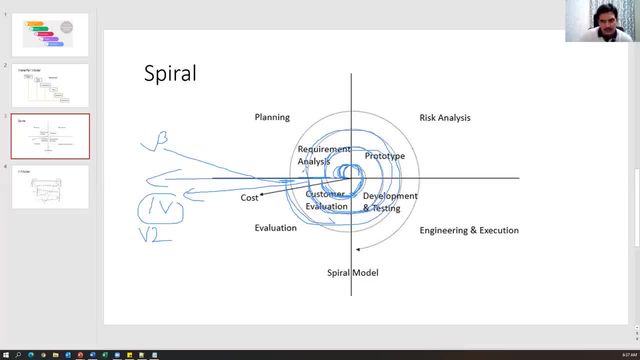 So each and every cycle will follow the same kind of process, But the process will be followed in the different cycles. Okay, so this is a behavior of the spiral model And if I just look at this, We are able to accommodate the customer requirements, some new requirements, suppose the customer 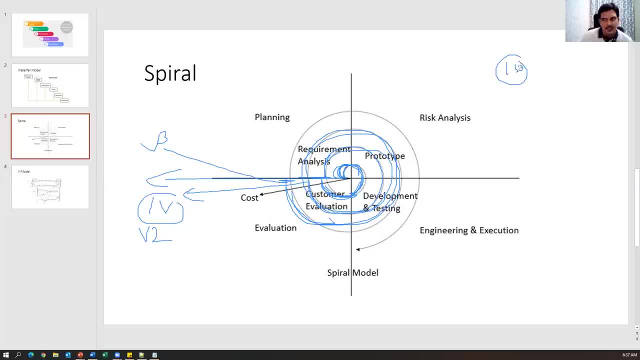 is given initially 10 requirements And for these 10 requirements we will complete one cycle And then we will deliver one software to the customer And he will keep on working on these 10 features. the first version is released And again customer came back and introduced five new requirements. 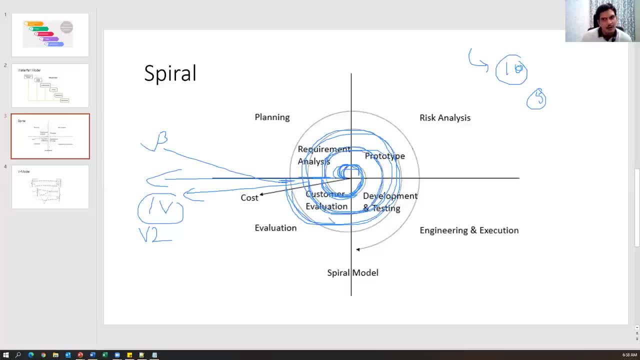 And then second cycle. we will implement the five new requirements on top of existing software. That's the second cycle. And similarly that even the customer is having some changes. suppose he's come back and introduce some new changes in the old requirement, then he can also change the requirement in the 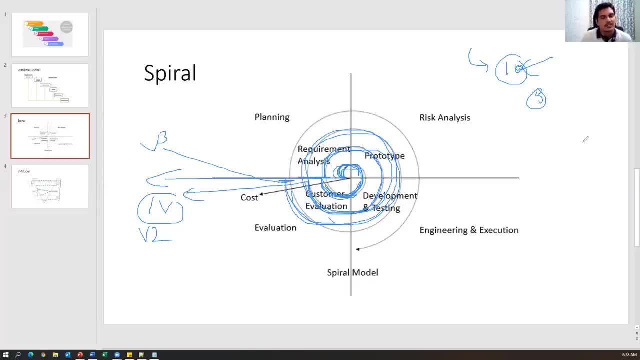 second cycle. So what is an advantage of this model? here is, the main intention of introducing this model is to accommodate the new requirements and also accommodate the frequently changing requirements. Okay, So in each and every cycle, after completion of every cycle, we will release a new software. 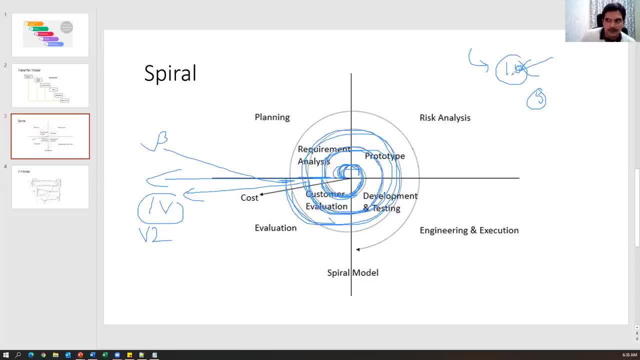 to the customer And we can also accommodate the new requirements or changing changes of requirements after completion of every cycle. And this cycle will be continued endlessly still. as soon as we have completed requirement from the customer, then we can still continue this spiral model. especially this model is: 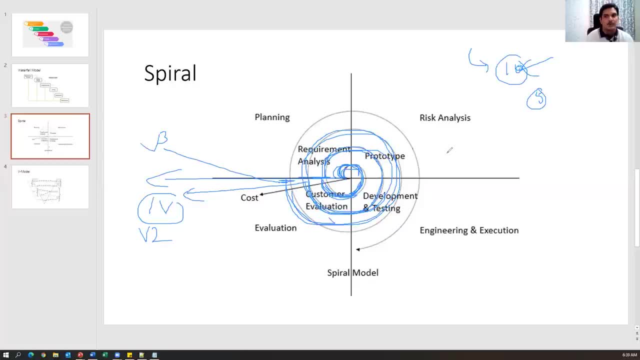 preferred for product based, Because what is product? product is a software which is developed based on the market requirements. So every time the market requirements will be changed And accordingly we have to implement the new features in the software also. So this model is especially suitable for products like product based. companies will follow this. 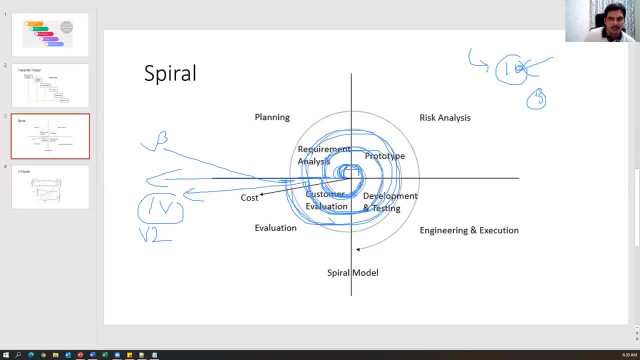 model And each and every cycle of iteration, the new software will be released to the market. And, for example, guys, Suppose, if you take it, If you take any software in the market, if you take any product, let's say WhatsApp, 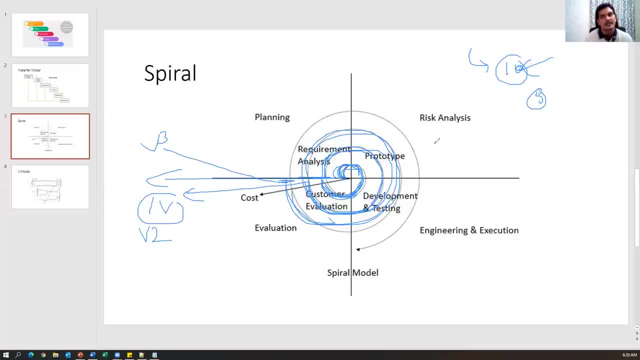 this is our application in our mobile right, WhatsApp. So initial days, WhatsApp is having very less number of features. After that, what happened? Every time we are getting some upgrade upgrades. So what is upgrade means the new features. So, based on the customer requirement, they'll implement the new features on top of existing. 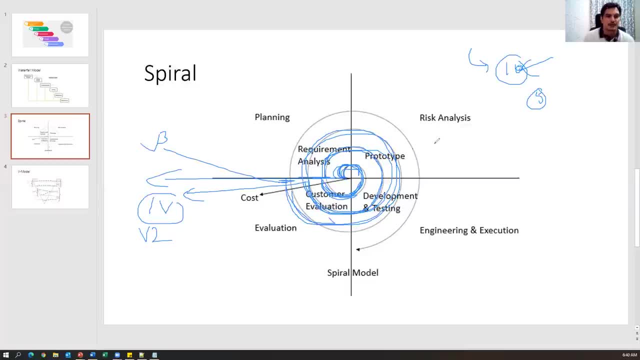 functionality or existing software, then they'll release a new software to the customer, So in iterator model. so this is comes under iterator model. You can say iterator means it is repeating again and again. the same number of phases will be repeating again and again with the new requirements. 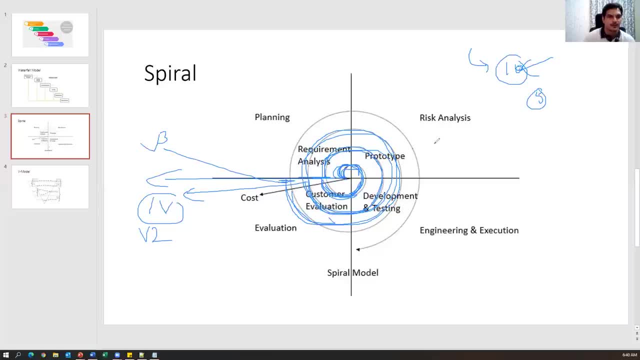 Okay, so especially this is suitable for products. So suppose Microsoft products. So we have Windows, Windows operating system. So in the olden days we have Windows 98,, Windows 2000,, Windows 2005,, Windows 10.. 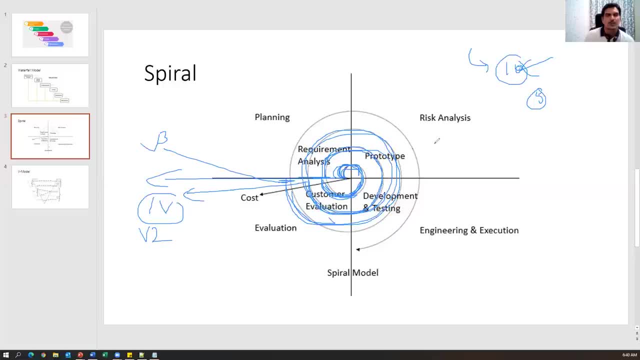 So there are different versions are there, And that is possible only through iterations based on the customer requirements. we collected the market requirements and we have implemented those features on top of the software. So this is the spiral model. So each and every cycle we will release a piece of software to the customer, not a piece. 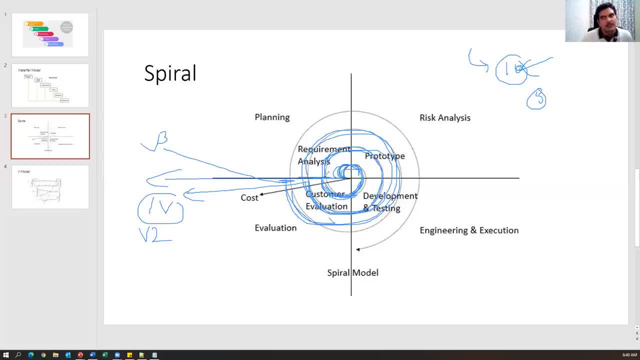 of software, But at that particular time, whatever the number of requirements we have from the customer, all the requirements we will deliver to the customer. After that we will take the new requirement from the customer. Okay, so this is modeled. actually, whatever the software we have implemented, 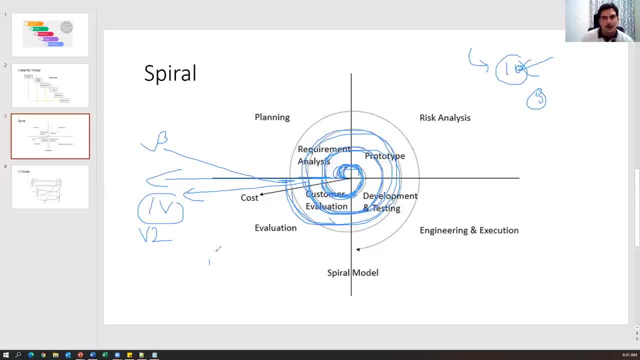 Okay, Whatever the requirement we have implemented in the first cycle, that is one model. And whatever the requirement we have implemented in the second cycle, that is a second model. third model. So in every cycle we will release a new model. 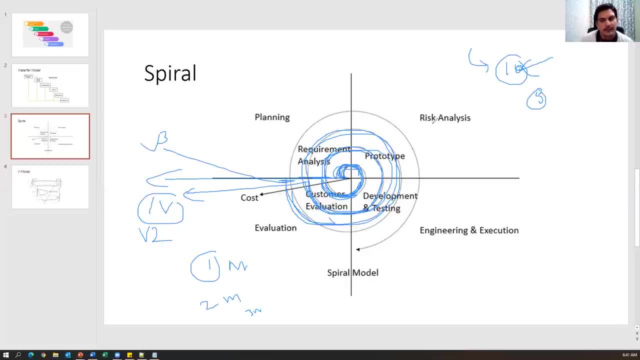 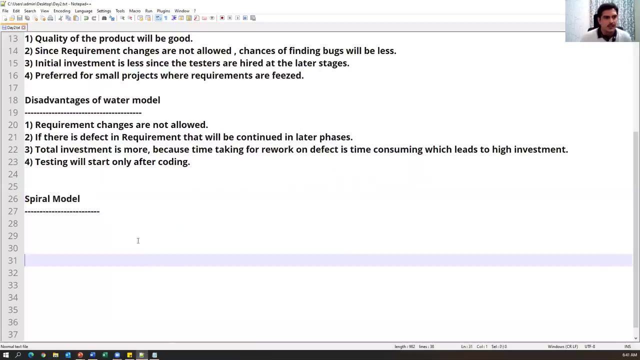 Okay, so this is a spiral model, So software development will happen in the cycles. Okay, so now let us understand. what are the advantages and disadvantages of this particular model? Now come back to the nodes. So what are the advantages, The advantages and disadvantages of the spiral model? 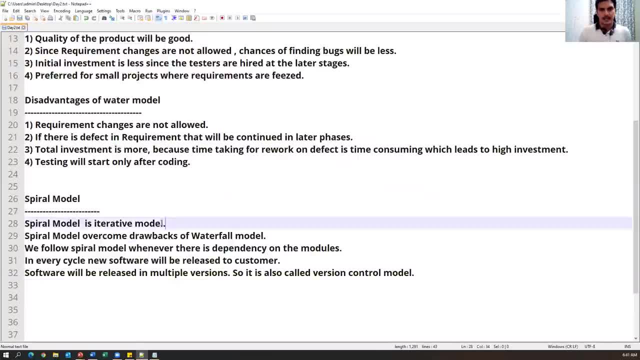 So I already told you a few points here. Let me just put here: the spiral model is an iterative model, As I said, every cycle cycle is nothing but iterative iteration. So repeated multiple times is called iteration. So spiral model is iterative model, where we are calling iterative model because all the 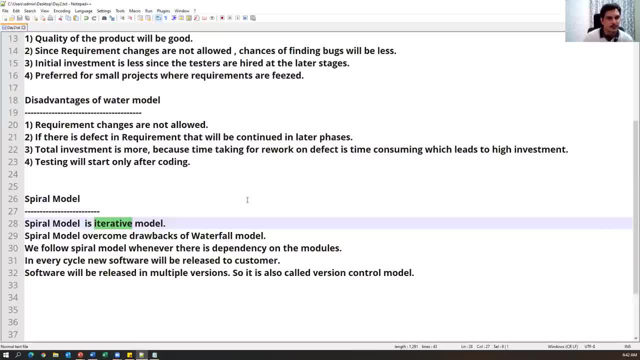 software development activities will happen in the repetition model, So we say iterative model, And which is also called version control model, because in each and every cycle we are releasing one version of the software to the customer, So which is also called as a version control models. 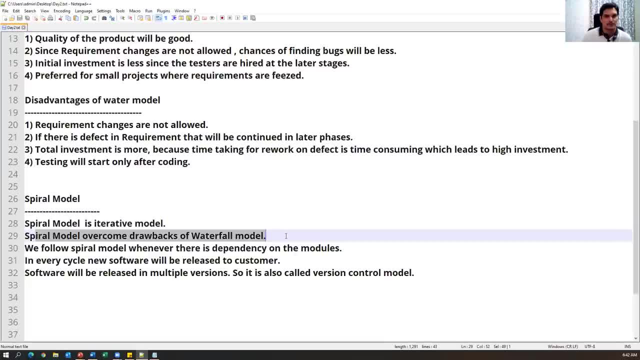 Okay, so spiral model overcomes the drawbacks of waterfall model. So what are the drawbacks we discussed in the waterfall model? Requirement changes are not allowed, But here the requirement changes are allowed. Okay, so spiral model is overcome drawbacks of waterfall model. And we found that in the first cycle we are releasing one version of the software to the. 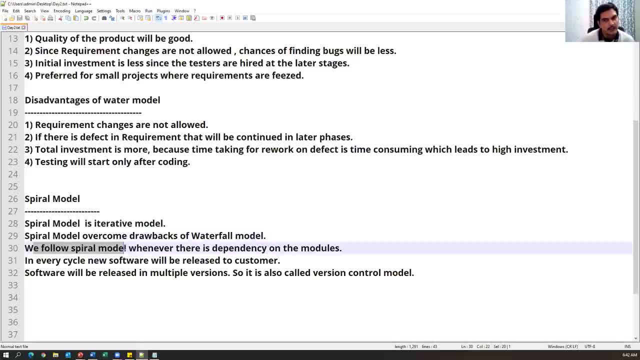 customer. Okay. So we follow spiral model whenever there is a dependency on the models. This is one of the important points, guys. So when we have to go for spiral model, So we follow the spiral model whenever there is a dependency on the model. 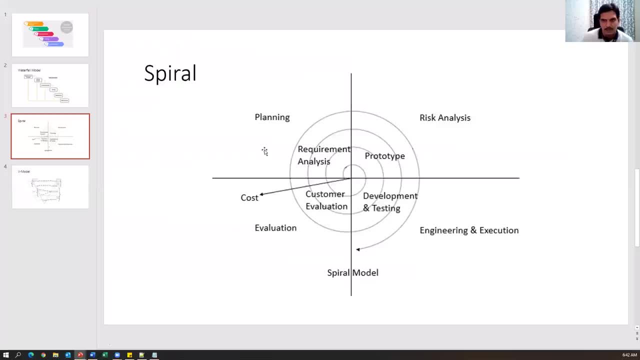 What does that mean If I just look at the spiral again? So whatever software we have developed in the first cycle, that is one model And whatever the new requirements we have taken from the customer- Okay, That is a depend on the previous model. 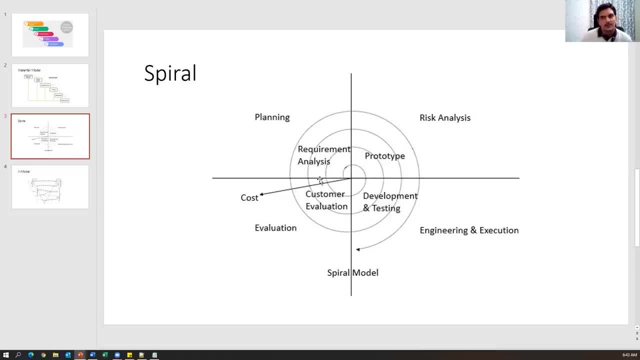 So whatever we have already implemented, the new requirements should be depend on the previous one, Because on top of this software, we are developing the new requirement. Understood, guys, right. So whatever we have implemented already, the new requirements should be implemented on. 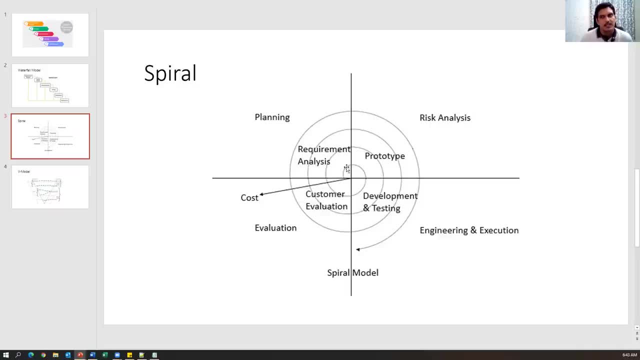 top of the existing software. So there should be some dependency. Okay, So suppose the customer is given 10 requirements, We have implemented all 10 requirements. We have implemented all 10 requirements here And again, customer gave another requirement that should be on top of the existing requirement. 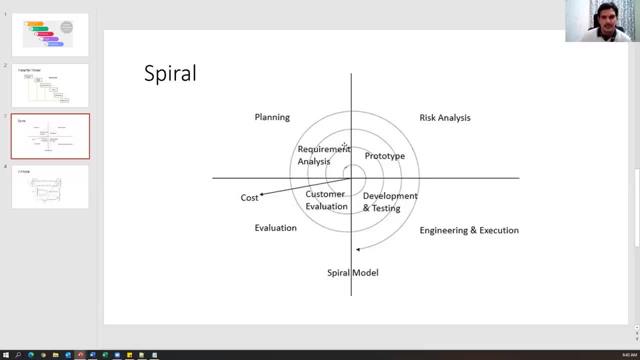 That means there is a dependency. There is a dependency. I'll just say simple example, guys, Suppose just look at the Gmail. So in the Gmail application I have one feature called compose email. So I have a feature called compose email. So open the compose email. I have put all the email subject. I have entered somebody. 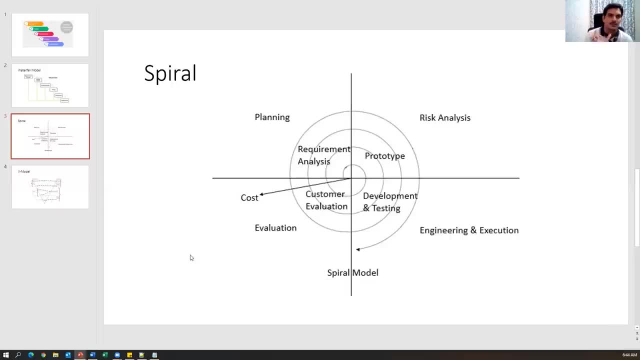 and sent Mail is sent. So till that That is one module. Let us assume that is one module. After sending the email, that mail should come to the out box. Okay, There is one more box, out box, whatever emails, or we can say send box. 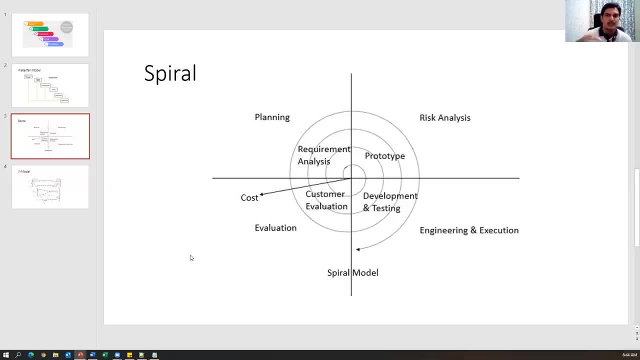 So whatever emails you have sent, that should be stored in the another, another box that is called, we can say, send mail box. Okay, And that is a different module. So the first module is a compose email, The second module is a send email box. 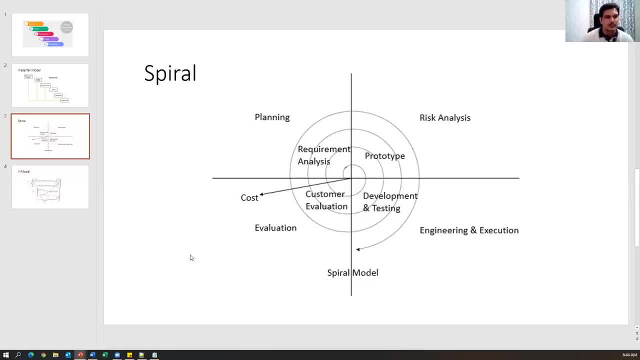 So whatever means you already sent That should be stored in the another box. So this is called as a dependency. until, unless you send an email, that cannot be saved in another folder, right? So that is called as a dependency. So first to the customers, given some requirements we have implemented and whatever requirement, 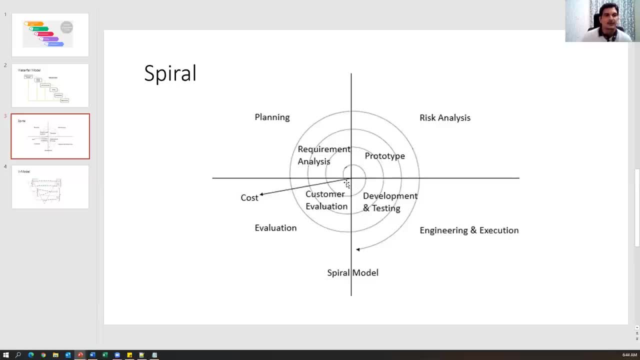 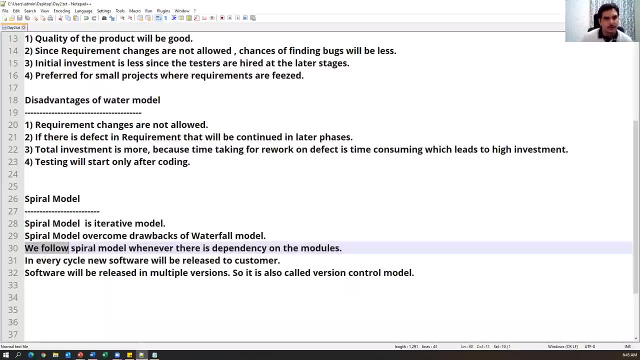 in newly, given that should be depending on the existing requirement. So in that case we can use spiral model. So that is a one of the points. So we follow spiral model Whenever there is a dependency on the model. Okay, And the next point is: in every cycle new software will be released to the customer. 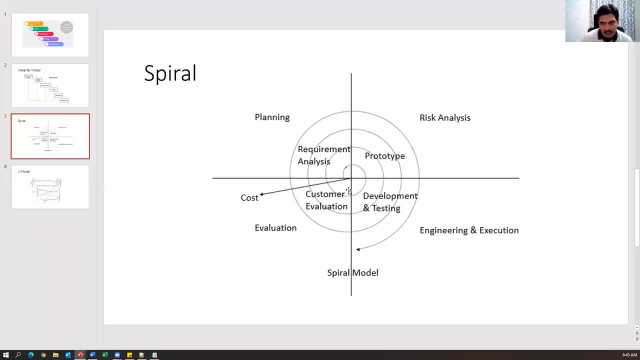 As I said, as soon as we completed one cycle like requirement analysis, design, coding, testing, but internally, every cycle, in every cycle, we follow SDLC process. again same waterfall model: we are falling, But the same waterfall model we are following in different cycles. 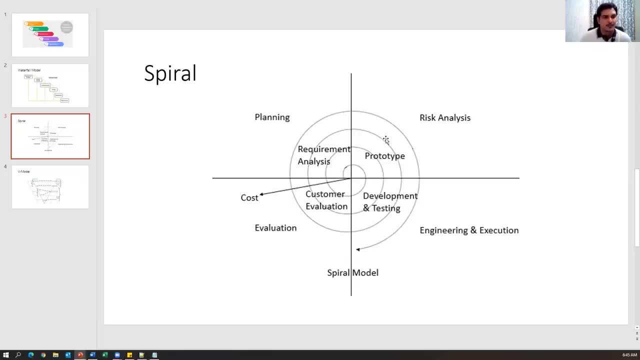 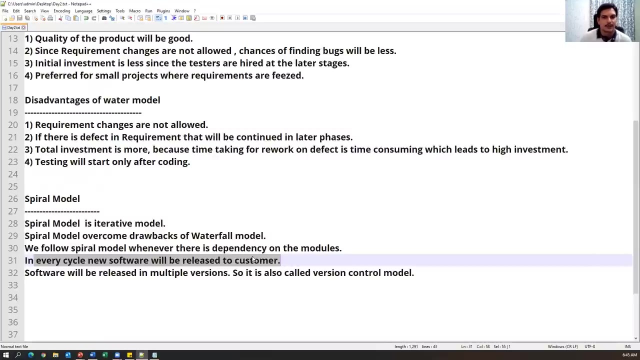 So that is a small difference between waterfall model and spiral model, And in waterfall model we don't have different cycles, But here, in each and every cycle, we are following the waterfall model. Okay, So in every cycle new software will be released to the market or released to the customer. 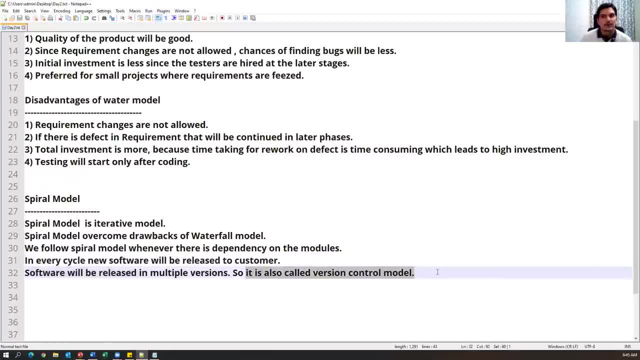 So software will be released in multiple versions. So it is also called version control model. As I said, once we get the requirements, we conduct the. we do all the process, requirement analysis, We do the coding testing and deliver the one software to the one version of software to. 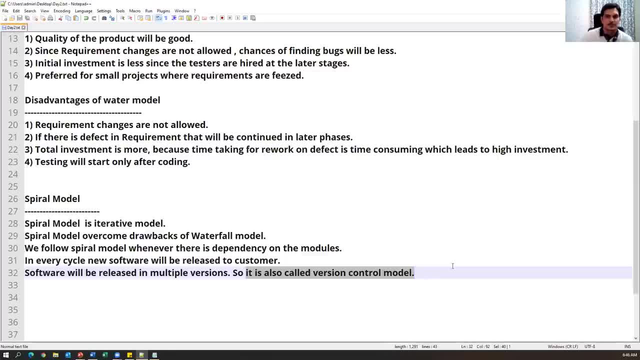 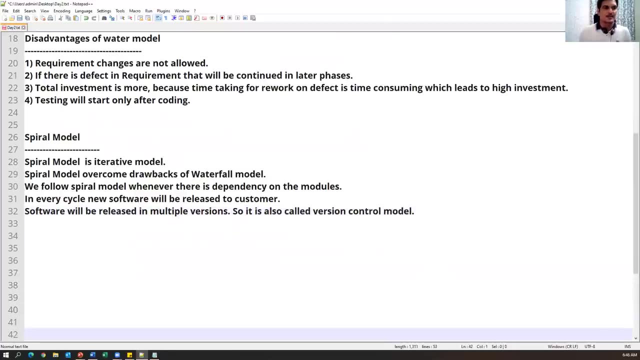 the customer, And then we will start with the new requirements. So software will be released in multiple versions. So it is also called as version control model. Okay, so these are the few important points which you have to remember for spiral model. So now let us discuss the advantages and disadvantages. 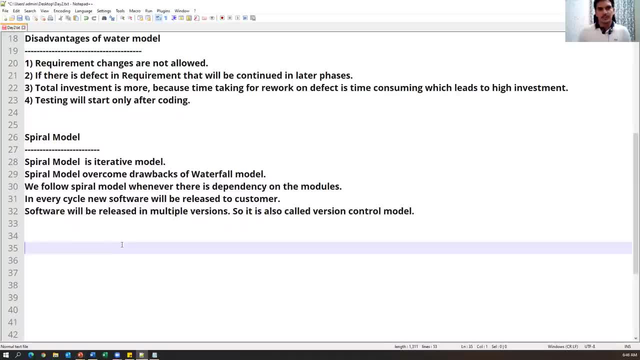 So first let us discuss the advantages. So what are the advantages? In interior perspective? these are very important guys. So, even though we are not working on these models nowadays, but if you go for an interview, people will ask some questions on this- you have to remember a few important points, okay. 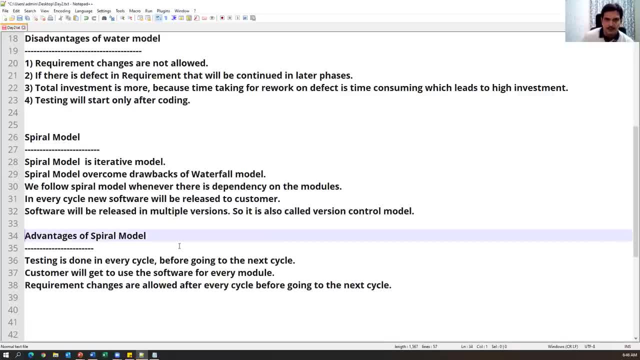 So advantage of spiral model. So what are the advantages? So, as I said before, testing is done in every cycle before going to the next cycle. So here, testing is done in every cycle before going to the next cycle. What does that mean? 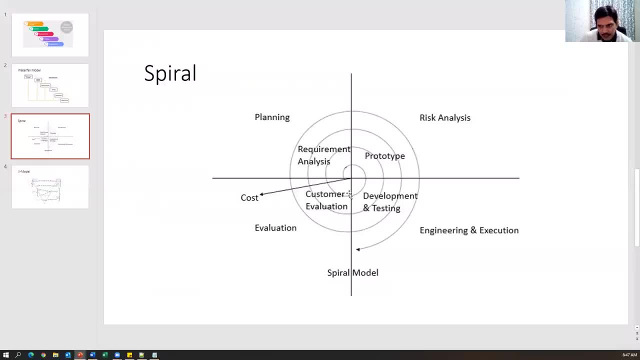 Again, Let us look at the picture. In every cycle we have all the phases. like in every cycle we are following waterfall. again, requirement design coding testing. that is one cycle. again requirement design coding testing. second cycle and again requirement design coding testing. fourth, 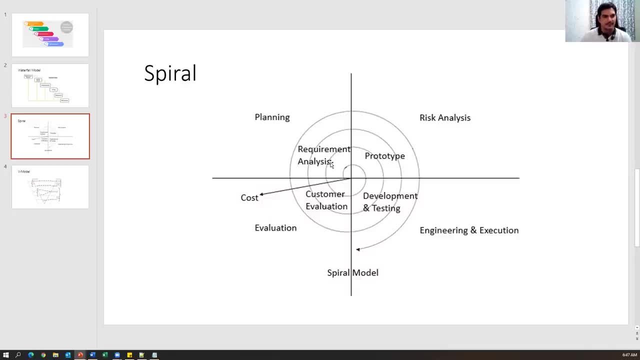 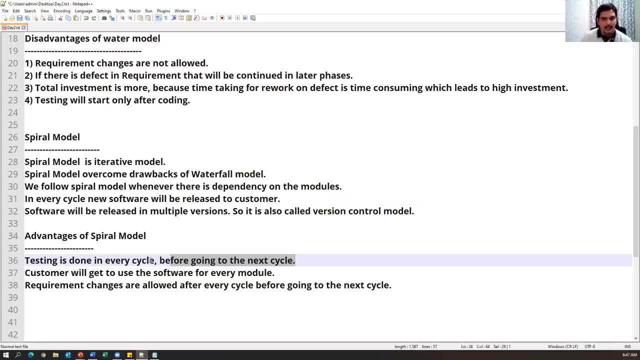 cycle. So in every cycle we have a testing. In every cycle we have a testing. That is one of the advantages. So testing is done in every cycle Before going to the next cycle, After complete, in each and every cycle we conduct testing once. 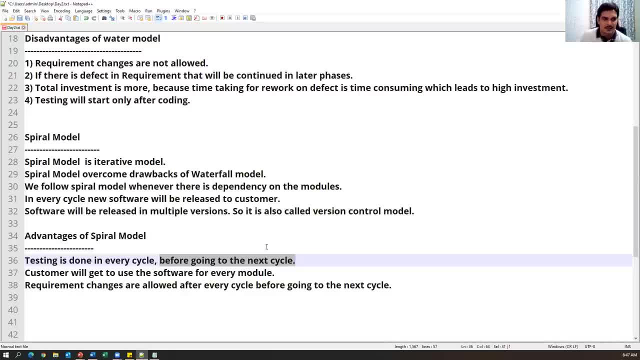 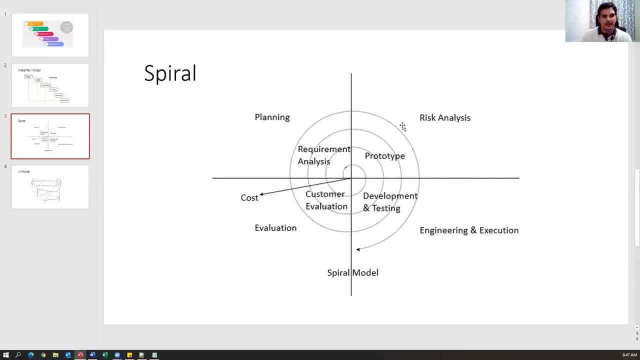 So testing is done in every cycle before going to the next cycle. The next one is: customer will get to use the software for every module. What does that mean? Customer? no need to wait for the full fledged software and whatever the initial requirements they have given. 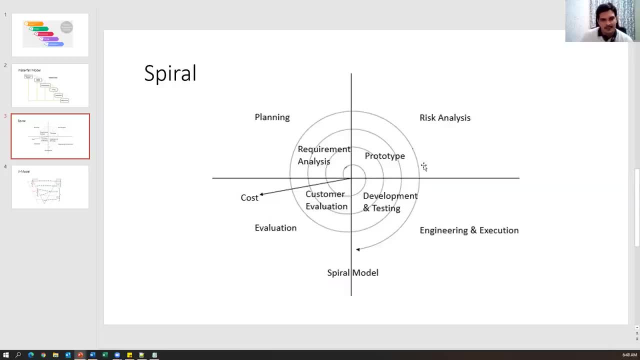 We can develop the requirements and test it. So that is one of the advantages. Okay, So we will give the software to the customer And he will work on the software parallely. we'll get another requirement from the customer. new requirement from the customer. 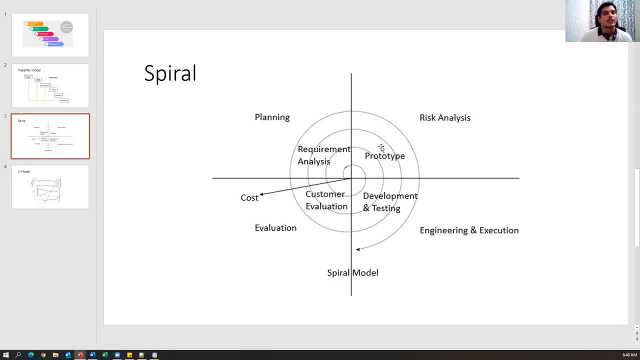 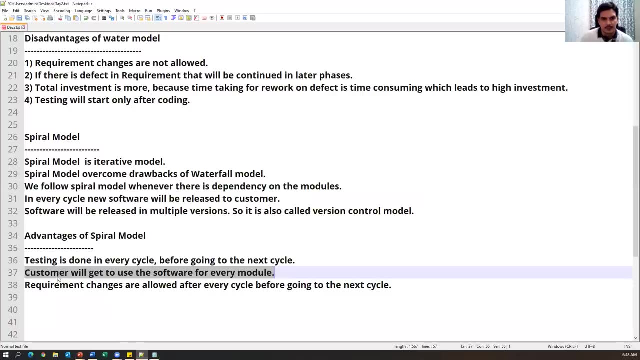 And again we can start another cycle. So customer is no need to wait till we complete the entire process or entire software. Okay, that is another point. So customer will get to use the software for every module. After completion of every cycle we are releasing the software to the customer. 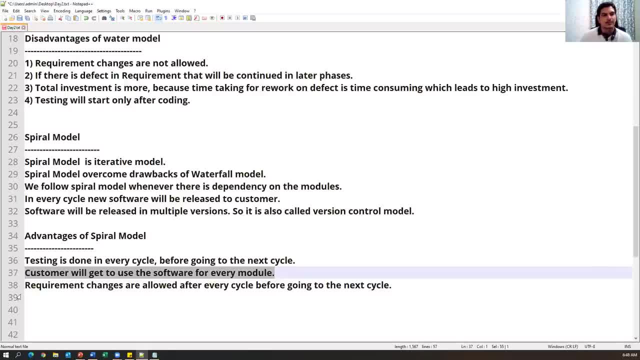 So he can start using the software. Customer: No need to wait till end. And the last advantage is requirement changes are allowed. This is a one of the important point in the waterfall model. the requirements changes are not allowed in the middle of development process. 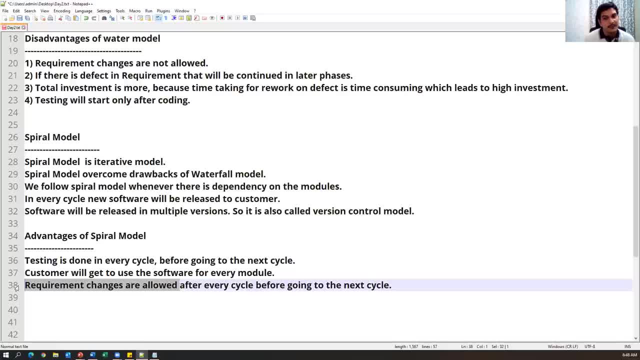 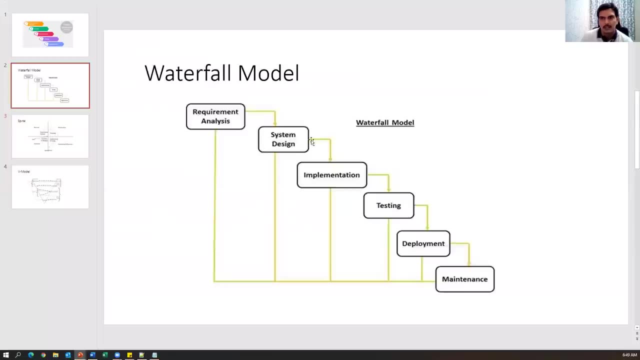 But here requirement changes are allowed after every cycle and requirements changes are allowed, but when after completion of the cycle, not in between the cycle Understood. So in the waterfall model Also, we do the same thing in waterfall model. 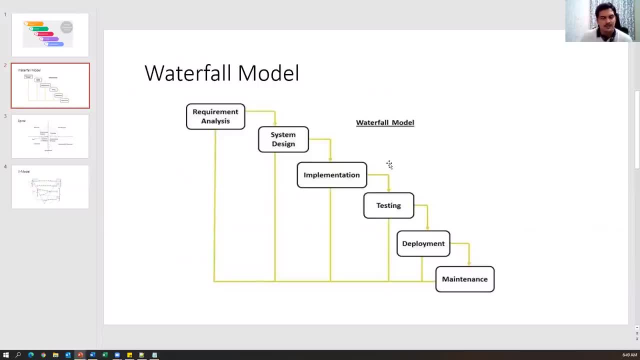 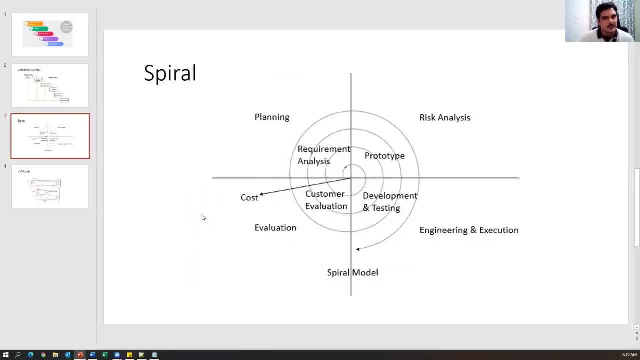 Suppose we are in the testing phase, Can we allow the changes in requirements? we cannot allow here, But in the spiral model we can accommodate the changes. But when we can accommodate after completion of the entire cycle or before starting the next cycle, we can accommodate the new requirement. 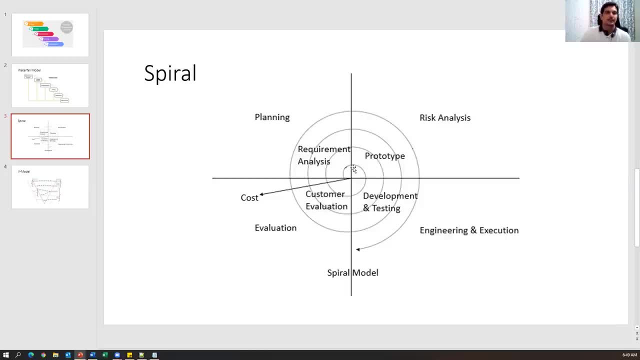 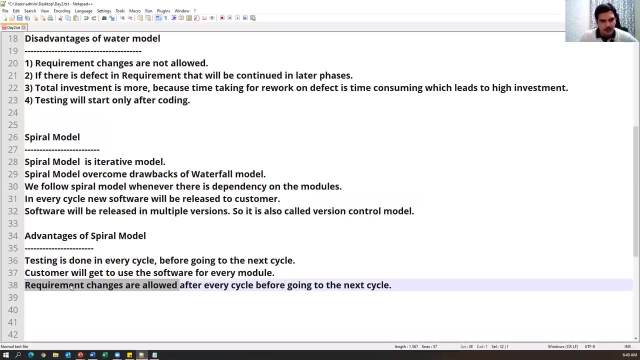 But in the middle of the cycle we cannot accommodate. Okay, We can accommodate the new changes, We can implement the new changes or new requirement, But in the middle of the phases, in the middle of the cycle, we cannot accommodate. So requirement changes are allowed after every cycle before going to the next cycle. 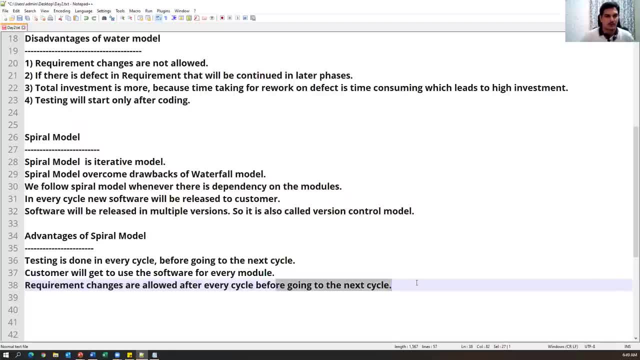 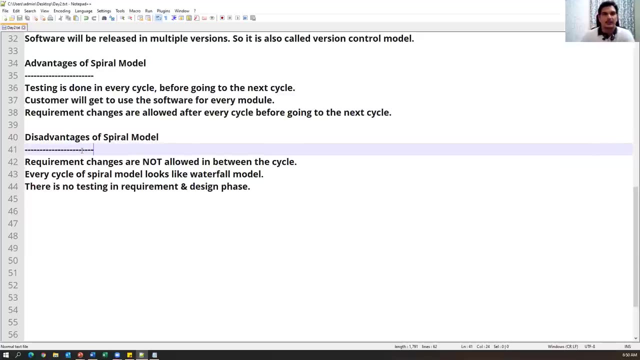 But in the middle of the cycle we cannot accommodate the new requirements. So these are the advantages of spiral model. Now we'll see the disadvantages of spiral model. Disadvantages, Okay, Disadvantages: Requirement changes are not allowed in between the cycle. 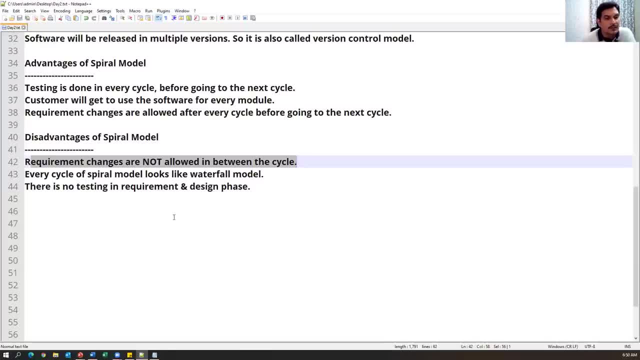 So requirement changes are allowed when we have to allow the requirement changes after completion of the cycle, But in the middle of the cycle or in between the cycle we cannot allow the new requirements. So that is one disadvantage. Every cycle of spiral model looks like a waterfall model. 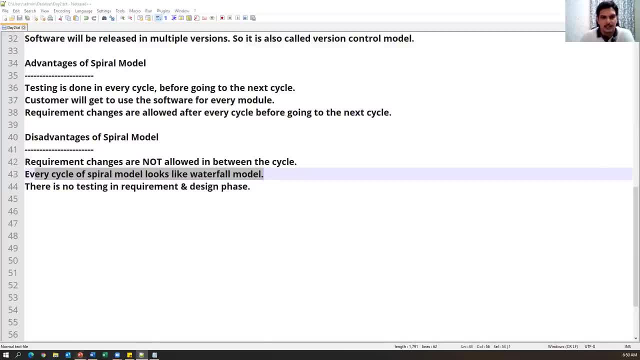 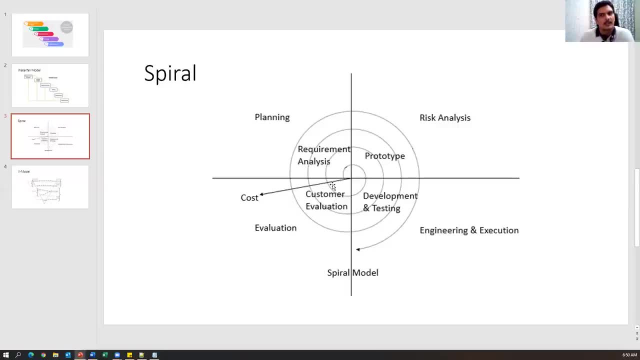 Again, the waterfall model is involved here. As I said before, every cycle we are doing requirement analysis, design, testing, design, coding and testing. So the same activities are going on in every cycle. So internally, in each and every cycle again we follow the waterfall model. 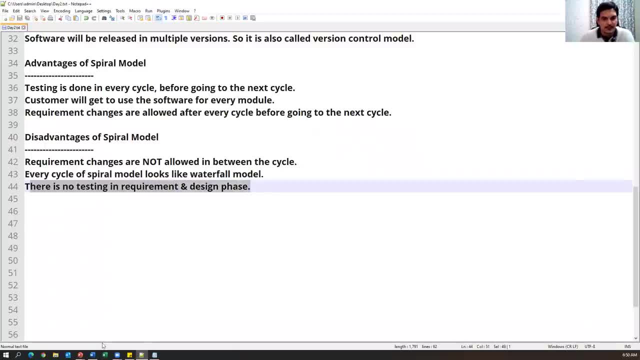 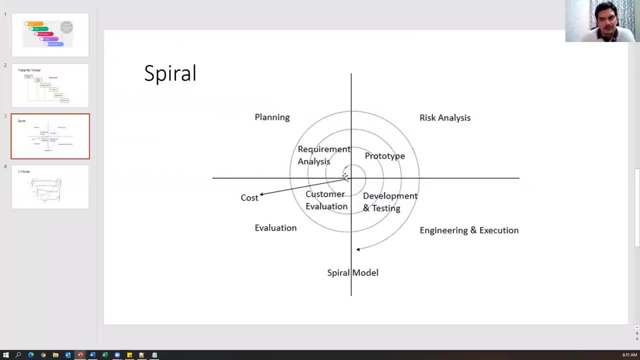 And there is no testing in requirement and design phase. but just look at this cycle. Here also, we have only one phase of testing in every phase, in every cycle. So if I just look at waterfall model, Okay, We have only one cycle, we have only one phase of testing, but we don't have any testing. 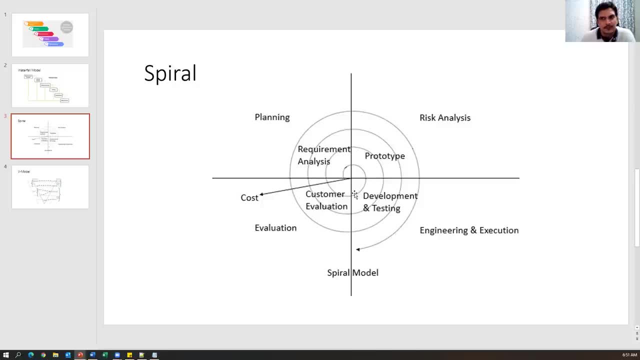 in the design phase or requirement phase And there are chances are there to get the more number of bucks in the testing phase. So because in the previous phases we don't have testing only we have one phase of testing in one cycle. So that is one of the another drawback. 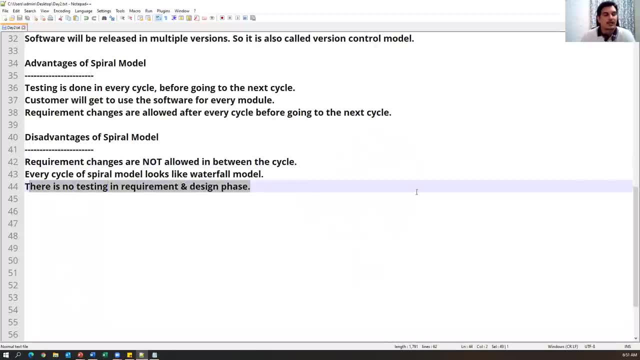 So, based on these two drawbacks, again another models are coming into market, because every model is having pros and cons. So spiral model: This model can overcome some of the drawbacks from waterfall model. Similarly, some other models can overcome the drawbacks from spiral model. 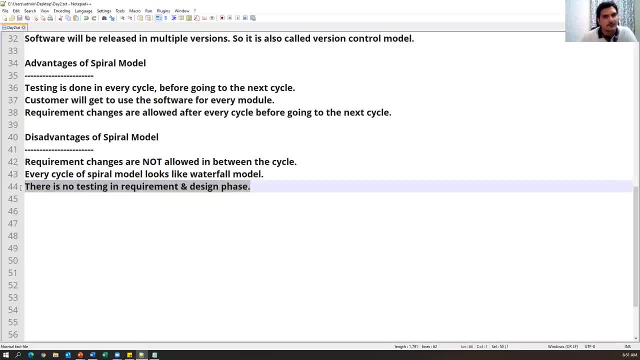 So there is no testing in the requirement and design phase. So these are the disadvantages in spiral model and requirement changes are not allowed in between the cycle. After completion of the cycle it is allowed, but in between the cycle it is not allowed. 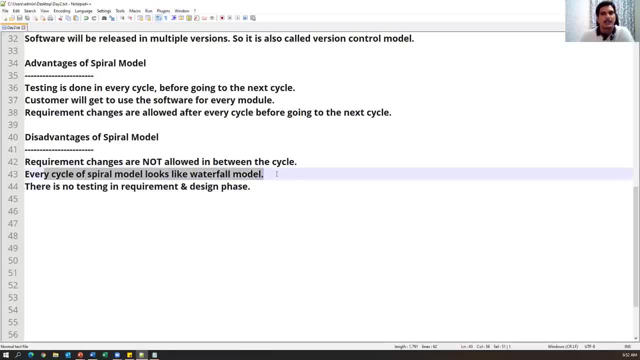 Every cycle of spiral model looks like a waterfall model, Because we have only one cycle, One phase of testing in every cycle, And we don't have testing in every phase. That is a drawback. So these are the advantages and disadvantages of spiral model. 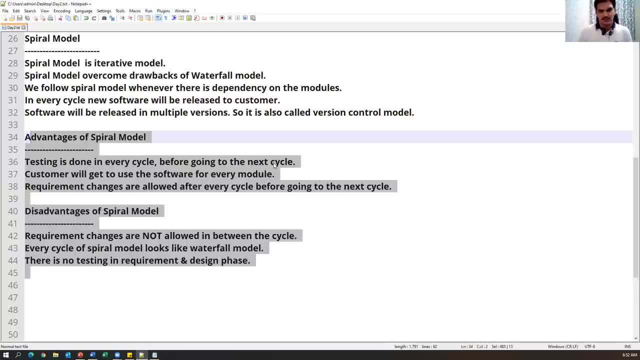 So these two are very old and traditional models. So nowadays most of the companies are not following these models, but still we need to understand what exactly these models and what are the advantages and disadvantages. Okay, now I'm talking about a new model, which is V model. 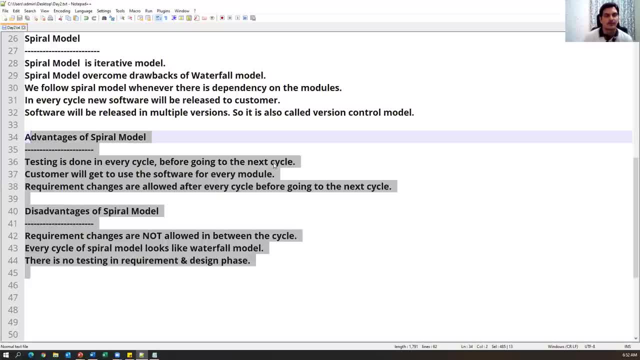 So in that particular model We can Overcome all the drawbacks from waterfall model and spiral model. Okay, so prototype is one of the model which is also available and which comes between waterfall and spiral model. So prototype is also one of the SDLC model which is there which comes between waterfall. 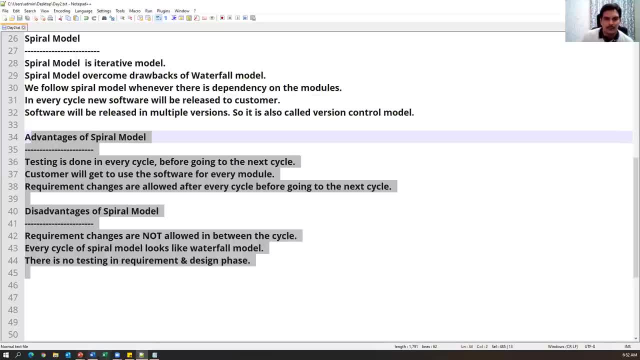 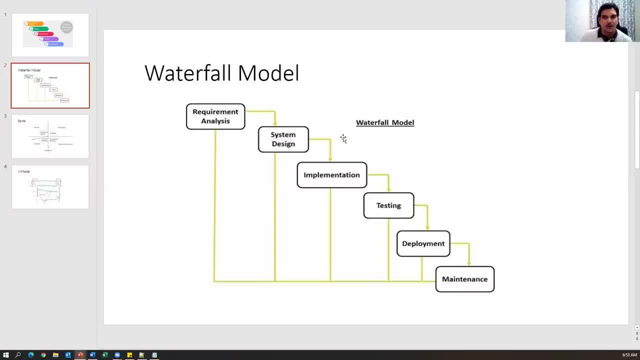 model and spiral model. But in waterfall model we cannot accommodate frequently changes requirement right. Suppose, if you are there in the testing phase, We cannot accommodate The new requirement. but in the prototype model we can accommodate the new requirement in the middle or in somewhere in the development process but there is no iteration in the prototype. 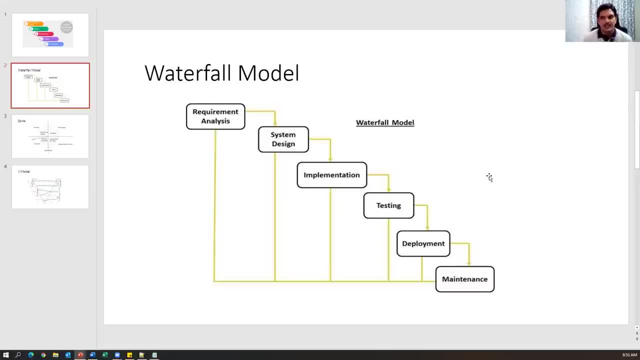 model. There is no iteration. Okay, so we can just get a small requirement from the customer. We don't need to get the complete requirement from the customer And as soon as you know few requirements, we can do requirement analysis on those requirements. 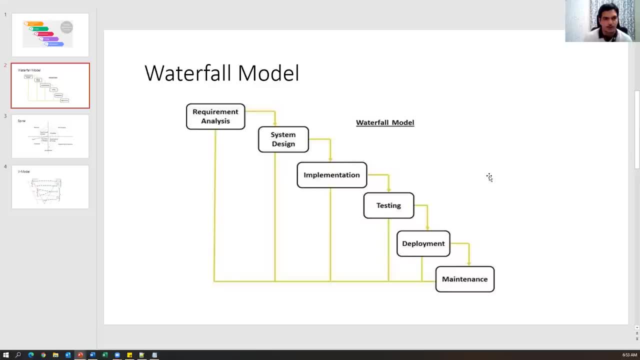 and design, coding, testing and deliver the software to the customer. One prototype, Okay, and after that again, customer will look at that prototype. prototype is a sample, Okay, let me just give you some points here. So prototype, I think Rahman, somebody asked what is prototype. 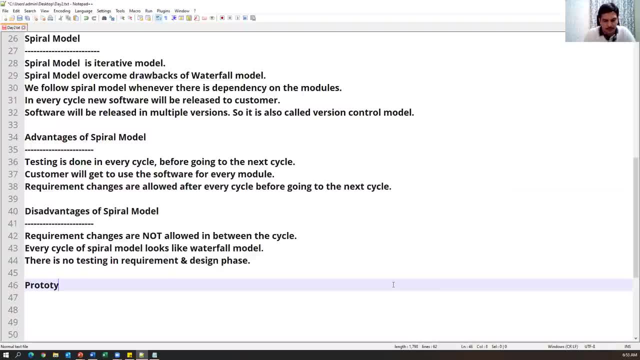 So maybe you can hear this term. So prototype model. Let me just explain what it is. a prototype is a- we can say- blueprint, blueprint of the software, Blueprint of the software is called as a prototype, Okay. So prototype, Okay, What you will do is in prototype model. normally what you will do is so: first we will get the 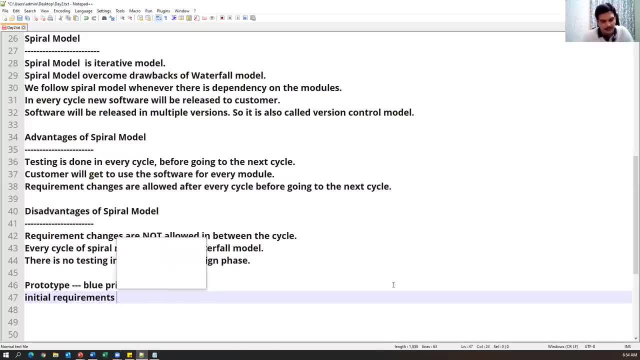 initial requirements, initial requirements from the customer. First we will get the initial requirements from the customer. Customer can have a number of requirements, but initial requirements we will get from the customer And after that we don't develop the complete software, we will develop the prototype. 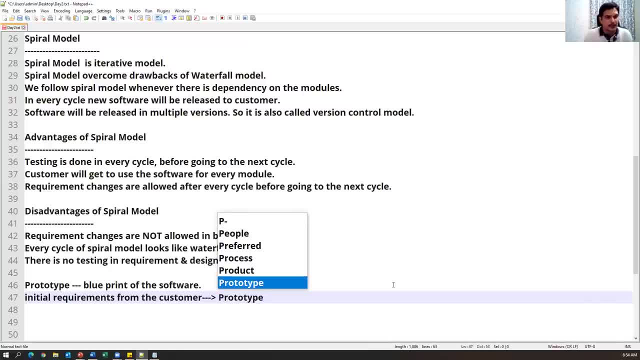 Prototype is nothing but a sample, a blueprint of the software And we will show this prototype to the customer, will explain this prototype to the customer. Okay, if the customer is satisfied with this prototype, then we will start design, coding, testing and different phases. 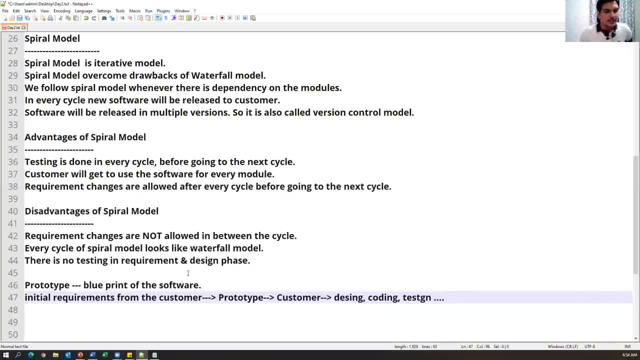 So prototype model is a prototype is nothing but a blueprint of the software And we will take initial requirement from the customer And we will just prepare some prototype model, suppose let me just give you some example of what is prototype Suppose before constructing the house. so we will have some plan in the paper. we will 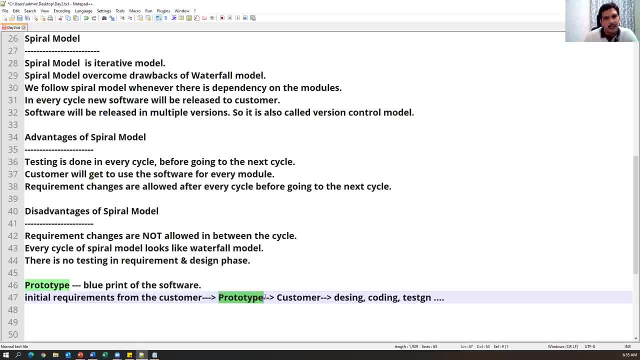 design the plan. That is a just a blueprint, And what is another? blueprint means? So, just like a toys, we will construct the house, right? So if I see some movies and everywhere, so before constructing the actual house we will see some kind of model house. 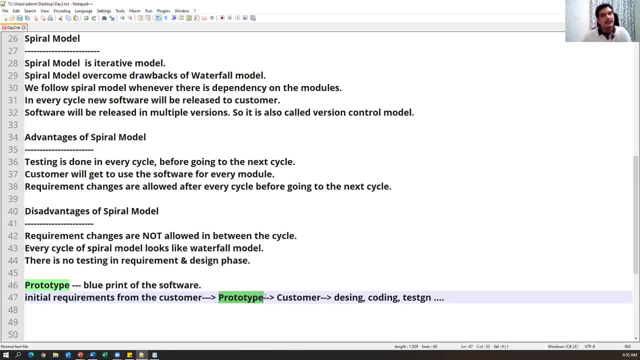 So that is a simply prototype. So here we will get the initial requirement from the customer, we will develop a small prototype and we will demonstrate that to the customer. If the customer is satisfied with that prototype, then we will start design, coding, testing. 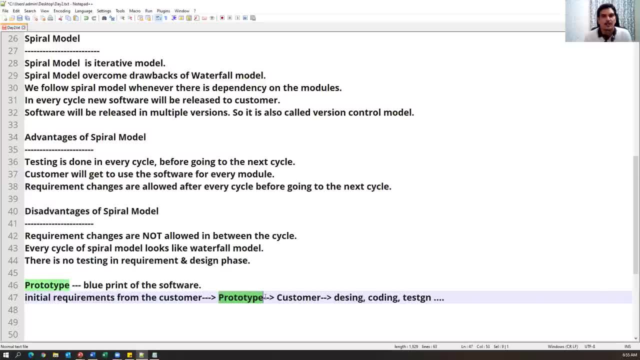 Okay, so here the chances are there. like the customer, involvement will be more here, Because every phase, or any, every step, the customer will give you the inputs And based on that, we will design the prototype and continue the rest of the process. 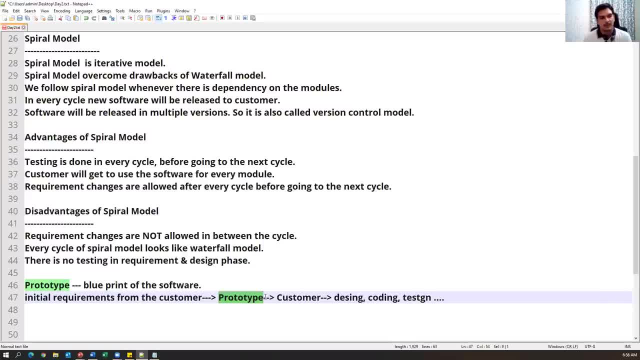 Okay, this, this, this particular model, comes between a waterfall and spiral model, So which is spiral is an advanced than prototype model. Okay, because even prototype is also having some different drawbacks. So, and we are just skipping the prototype model because it is also having some drawbacks. 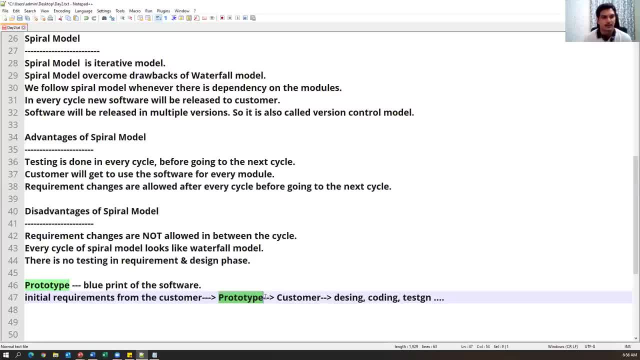 which we can also overcome by using spiral model, because if you have a number of features if you want to accommodate in prototype, it is not possible. Okay, so that is a prototype. So what is model? Okay, So model means a simple component of the software. for example, if I take email. okay, let me. 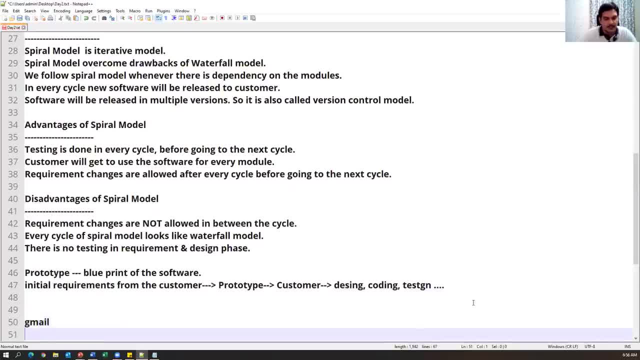 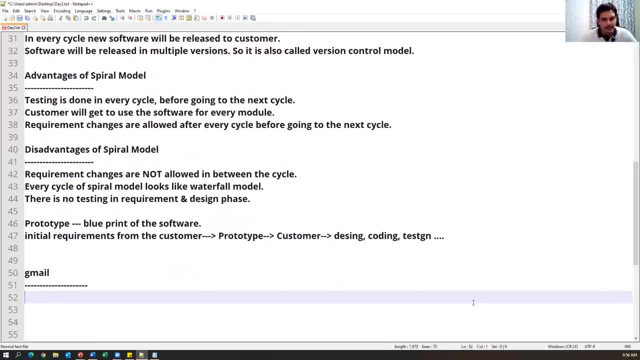 just take with some example: it's a Gmail. I have taken Gmail application. okay, everyone know about Gmail, right? So what do we can do in the Gmail? In the Gmail, what we can do, we can do the first login. 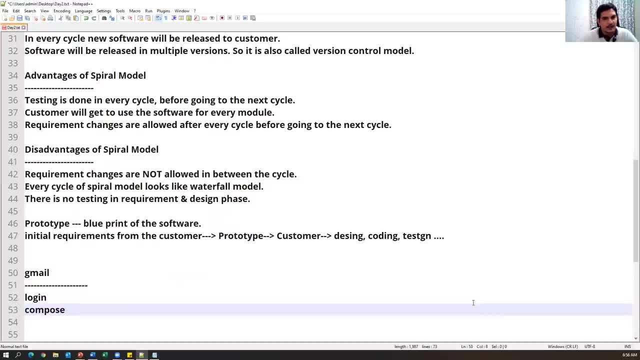 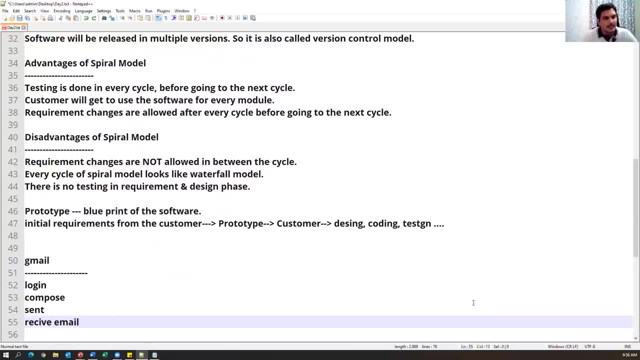 After login, we can compose email. After composing, we can send an email or what we can do: we can receive an email, We can receive an email and a lot of features we have, so we can do a lot of things. 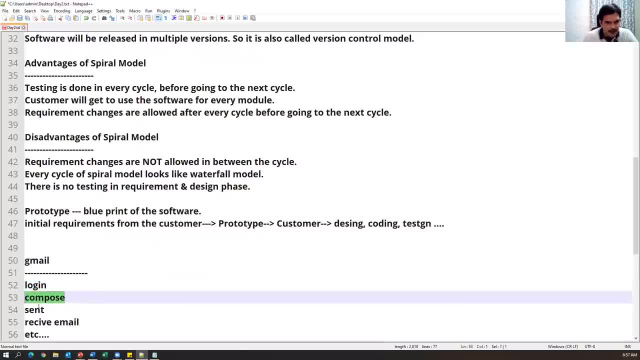 And if I just look at this, every feature, every functionality is a model. okay, login After login, we can compose a mail and we can check the inbox, we can check the mails which we have got, And this is one model and we can compose a mail. that is one model sending a mail. 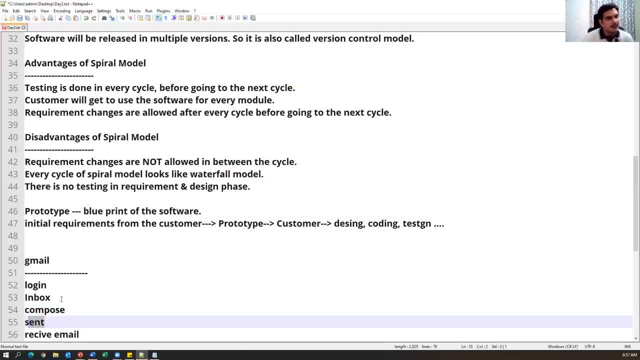 that is another model. So every application features a model, Okay, Okay. So, first of all, if the model is aaitan, they need to be user-friendly. right, They need to be a, because most of the objects that we buy in the store that we purchase. 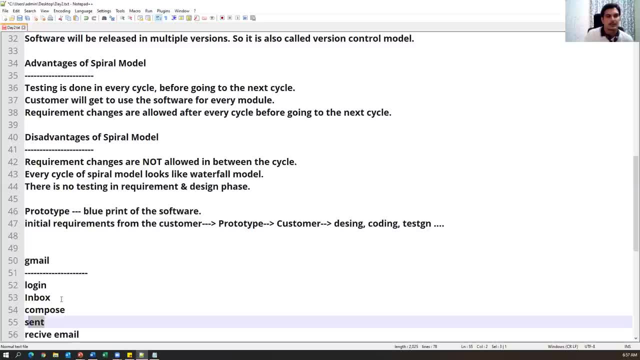 in our store are user-friendly right. So most of the documents which we buy in our store are user-friendly. Alright, Right, That would begreat. Okay, work on one module and another module. some other group of people will work, so module is nothing. 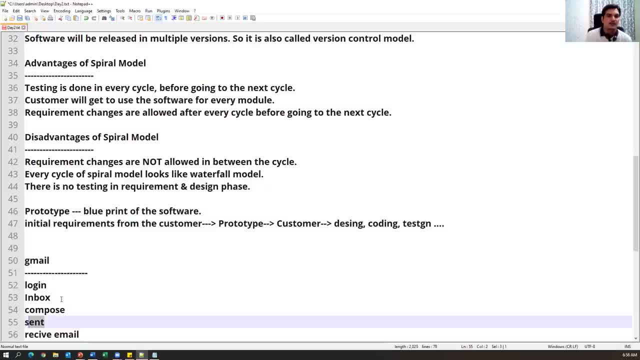 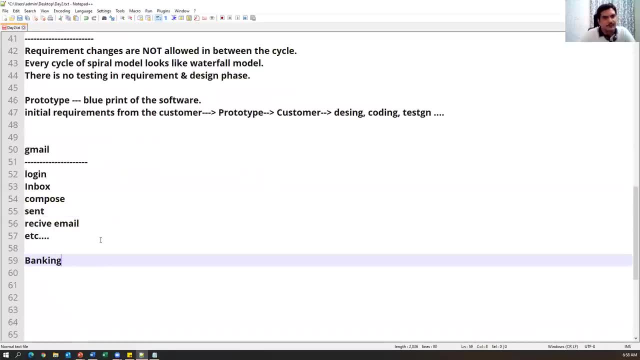 but a piece of software which contains a few number of functionalities from the application. okay, similarly, if i take some banking application. so what are the different modules we have in the banking? again, we'll start with the login part. login is a one module. we can say: and after login, 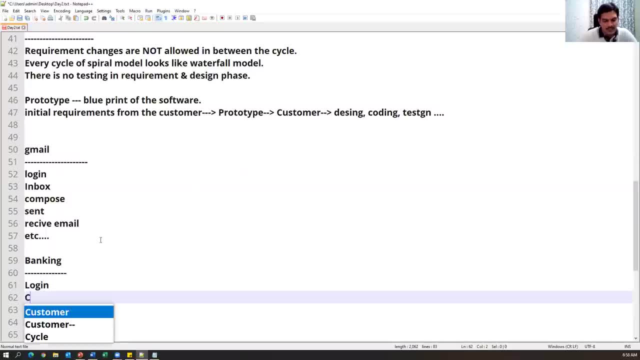 what are all things we can do in the banking application so we can check the balance right? this is one module, this is one piece of functionality, and we can do some fund transfer. this is one module and then we can. we can do fund transfer, balance sick and what else we can do. 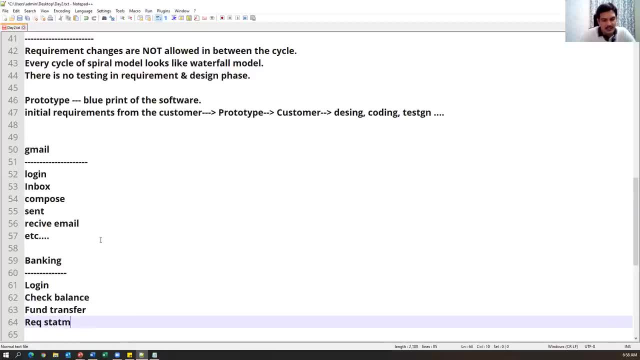 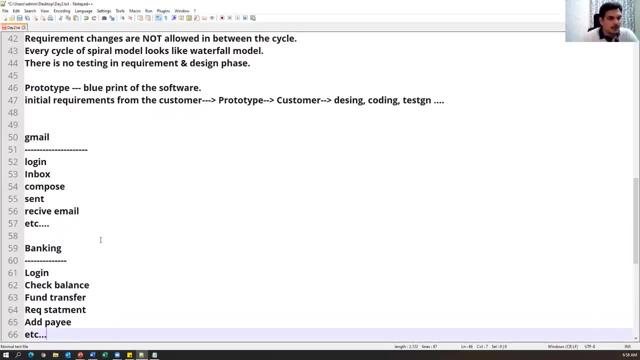 we can request the statement. we can request the statement. we can add p, e. so these are all different modules in our application. so different module is nothing but some piece of software which contains some number of features, or we can say each feature is one module. okay, understood everyone. so what is that module? so module is a part of the software, entire software. 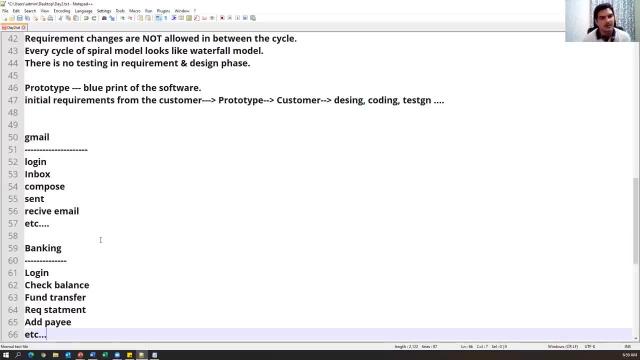 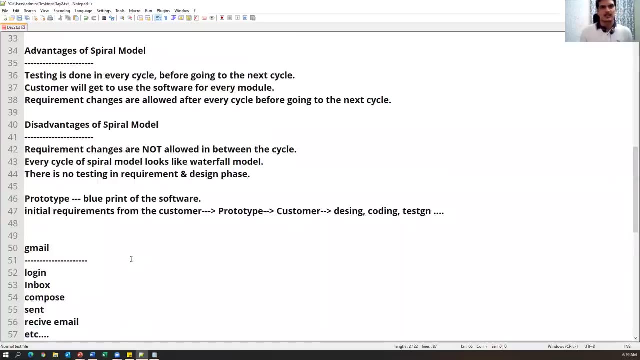 will be divided into multiple parts. so each module is called, each part is called as a model. okay, so whatever functionality you can see in your application, we can consider that as a module. okay, all right, so now let us move on to the next model. okay, so we have discussed about. 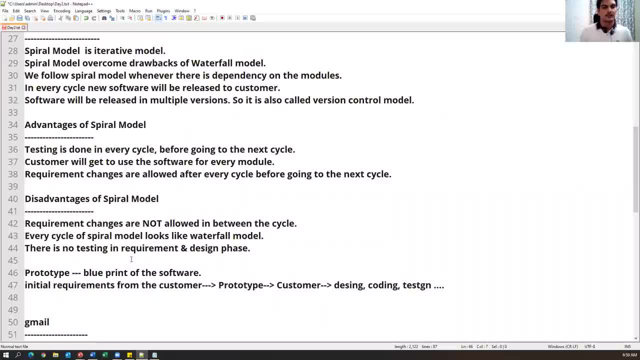 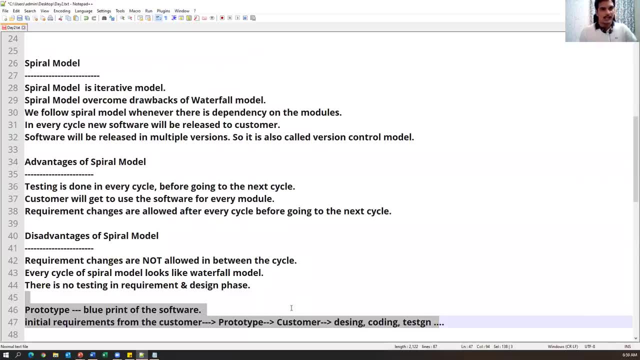 waterfall model, spiral model. then we are moving to another model called v model. so prototype model is not that much important because this comes between waterfall and spiral. so first waterfall model and then prototype and to overcome the problems from spiral and what us prototype, then spiral model come into. 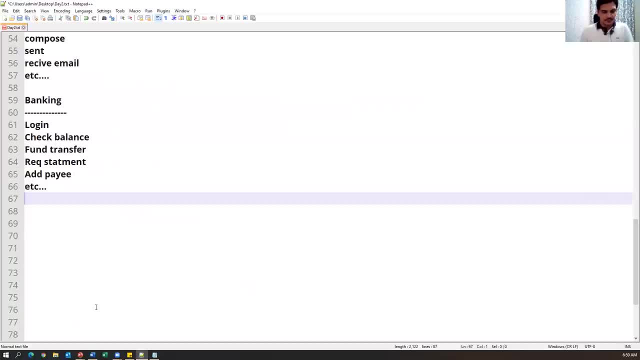 picture. okay, now let us move on to the v model directly. so now i'm introducing one of the important model called v model. this is also called as vv model. vb model means verification and validation model, vb model, v model or vv model. okay, so yvt is called as a v model. 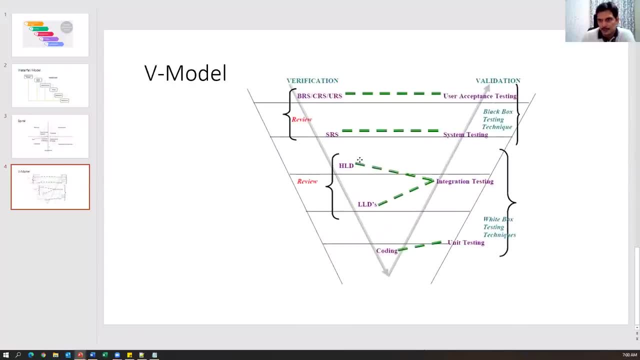 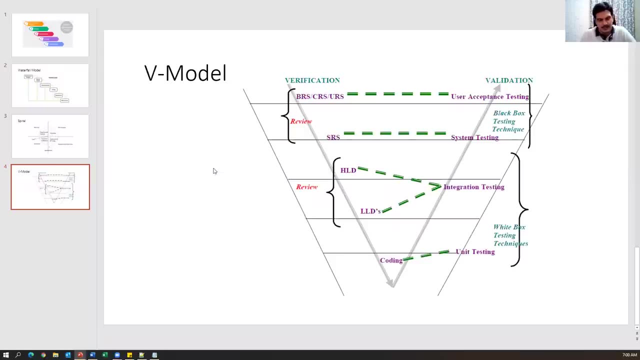 v model. so this is most important. guys, please look at this. lot of things we have to know here, lot of things are there. so first let us understand this model and then, uh, we will discuss advantages and disadvantages. okay, all right, so v model. v model is also one of the software development. 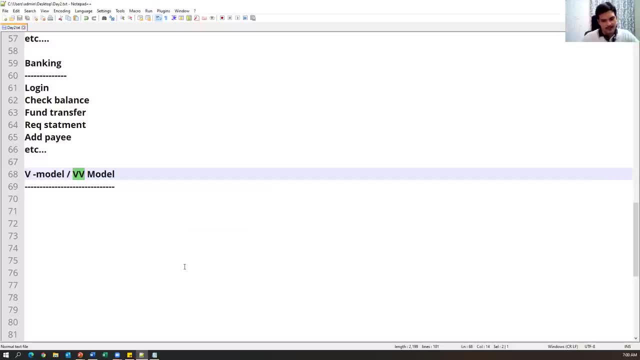 process model, sdlc model- like what fun model. spinal model. v model is also one of the software development process model, so let us try to understand. so what is this v model and how the activities will go on. let us carefully listen in the v model. if i just look at this picture, 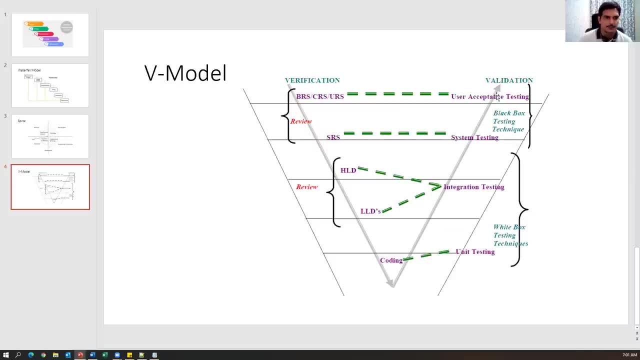 it seems very similar to the v shape right. this is one part which is comes under verification. the other part is comes under the validation. so one side is completely verification part, the other side is completely validation part. okay, that is the one thing. so let us try to understand what exactly it is. 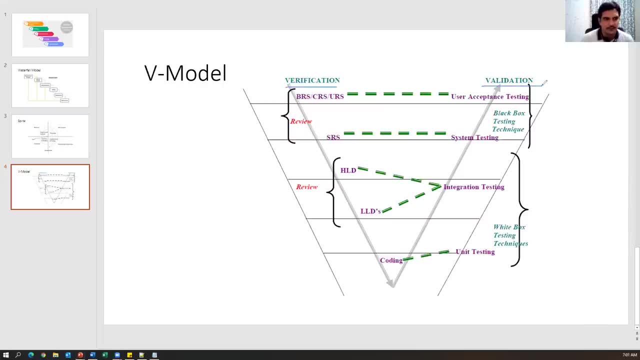 so this is a verification and validation. i'll tell you what is verification and validation. just let us discuss this. so in the main specialty of the v model, the main specialty of the v model is: in every phase we will conduct the testing. so, in every phase we conduct the testing. what does? 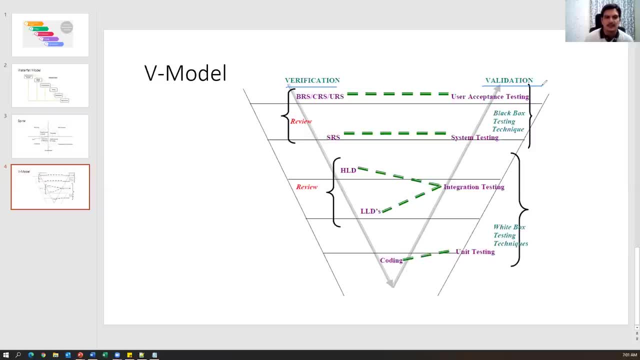 that mean in the requirement analysis phase we do testing. in the design phase. we do testing. in development phase also we do testing in the testing phase also we do testing. so in every phase of software development process we do testing. so that is a specialty of the v model. so in every part of development process we will conduct 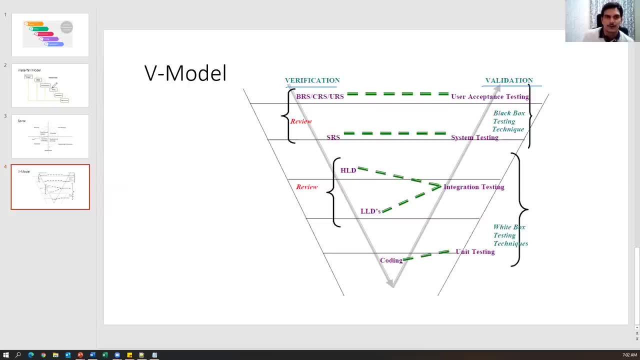 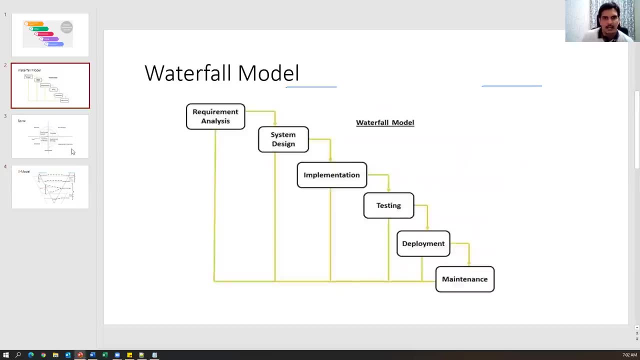 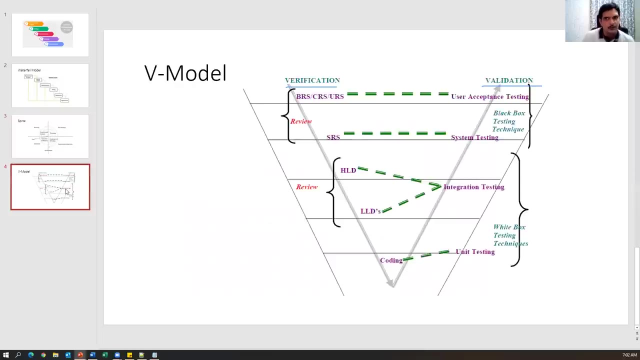 testing. but previously it was not there in the waterfall model, if you look at here. so in the waterfall model, if i look at here, we have only phase of testing and even in the spiral model we have only one phase of testing in every cycle. but now in v model every phase we have testing in requirement phase, we have a testing in design. 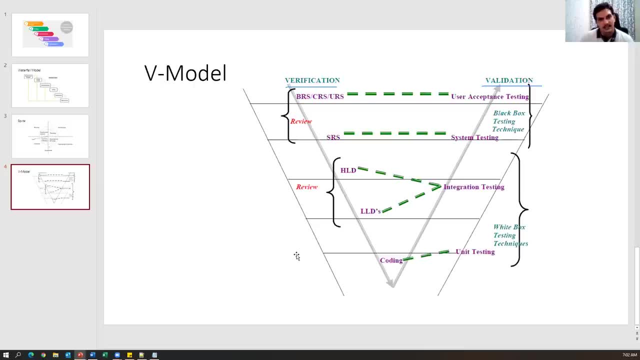 phase, we will conduct testing. in the coding phase we will conduct testing. in the testing phase also, we will do some testing and every phase we have testing. so that is a specialty of the v model. so now, if i just look at this, one part is verification, the other part is validation. 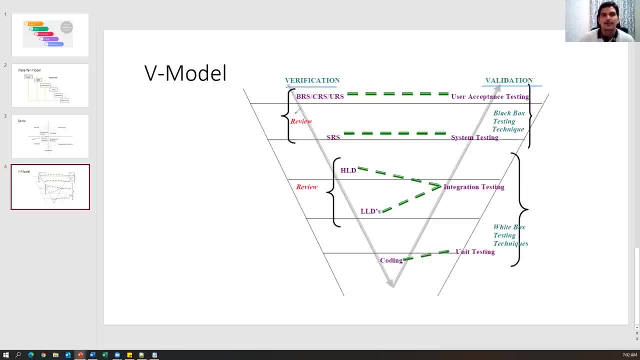 now, what is the first phase in the software development process? what is the first phase? collecting the requirement from the customer. so here we have something called brs, crs, urs. what does that mean? business requirement specification or customer requirement specification or users requirement specification? so the 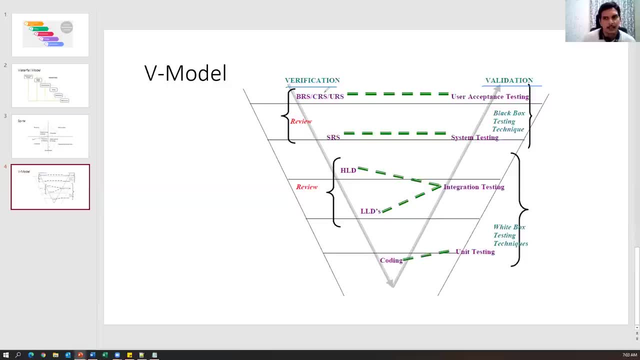 the. the is different, but the context is same. they are talking about one document, that is, business requirement specification document. what exactly it is? what it contains? so, basically, this document contains the business requirements. what is business requirement means? whatever the requirements are given by the customer or client will be noted in this brs document. 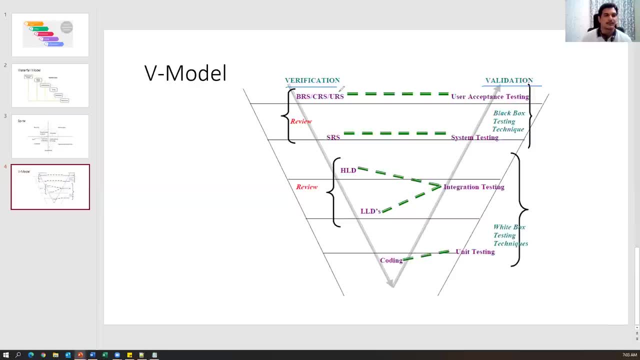 so who will prepare this document? business unit, so in our company means there will be a team called business unit and those people will interact with the customer and they will collect the requirements and they will prepare the document. and this document more can be understandable by the business people, not from the technical people. so, technical people- 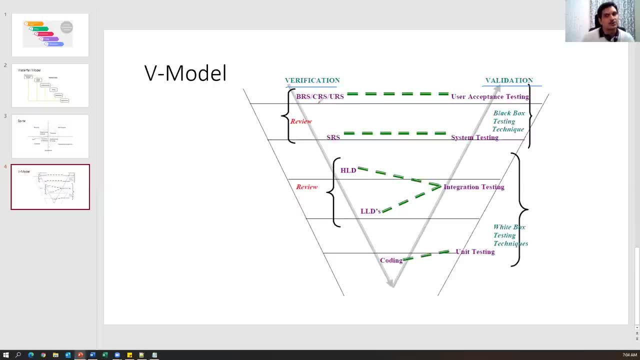 cannot understand this document. it is very huge document and customer and business unit. so these people involved in this document, so they will collect all the documents and there is a lot of the requirements and note down in one document that is brs, crs or urs is the first phase of. 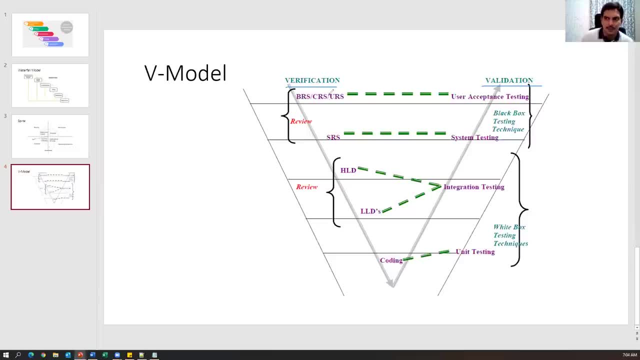 software development process now observe this. so this particular document, based on this document, we conduct one testing called user acceptance testing. okay, i'll talk about this in detail, so for now just understand: this document is going to be input for user acceptance testing. we can call it as a uat testing. u80 means user acceptance testing will be conduct based on this document. 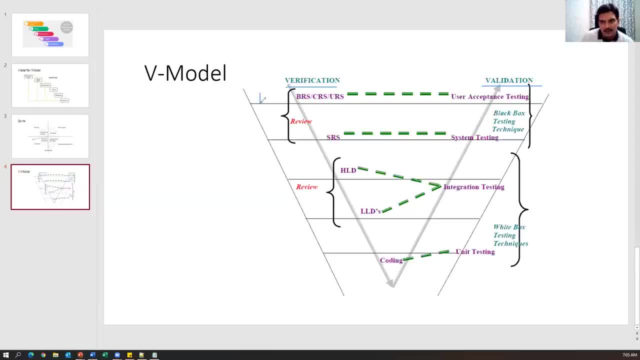 remember this. now the next phase is the first phase. now the second phase, but this is a document cannot be understandable by the developers or testers. okay, so we need a document which contains some more technical details. so, based on this document, there will be another document will be prepared. 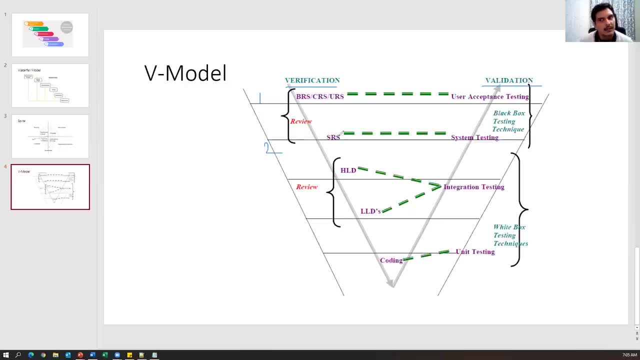 that is srs document, software requirement specification document. okay, so in the coming sessions i will show you all this document, how these documents will be prepared, how these documents look like. okay, so brs, crs or urs- this document cannot be understandable by the technical people. only business people can understand. but if you want to understand, 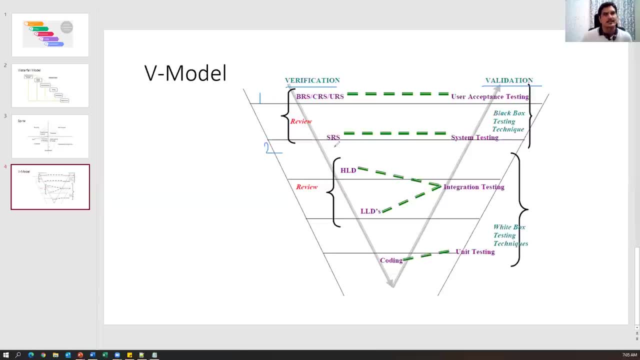 the requirement. you have to convert that into srs. so srs contains more technical details, the same requirement, but it will be present in the technical format by using like data flow diagrams or van diagrams. so we use certain diagrams in the srs and technical people, especially developers and testers. 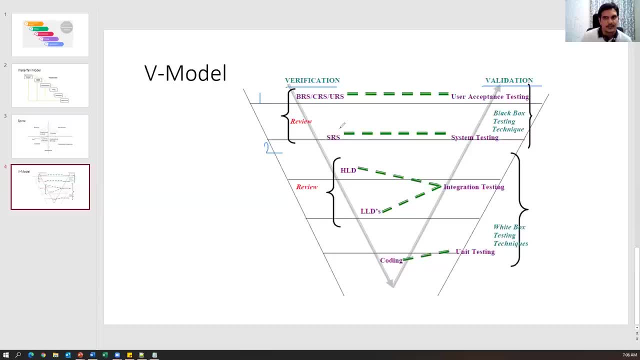 can understand. so that is the next document and they are based on the srs document. the designers will prepare hld and lld document. high level design documents, low level design. these are third section hld and lld. hld means what high level design document which contains the main modules of the 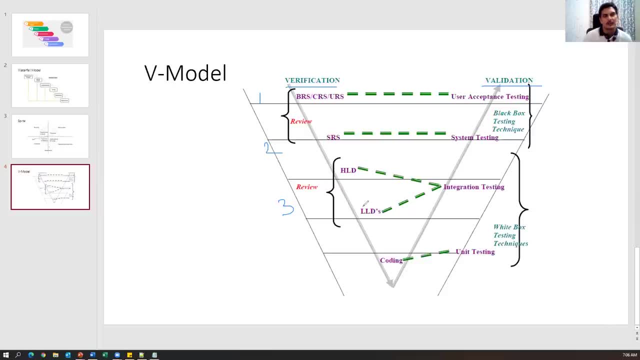 application. lld means low level modules of application. so as we discussed, what is module means? model means is piece of functionality in the application. so here the entire application will be divided into main modules. again each module is divided into some sub modules. so those sub modules, a low level design. so in hld document we will have main modules, in lld we have low level. 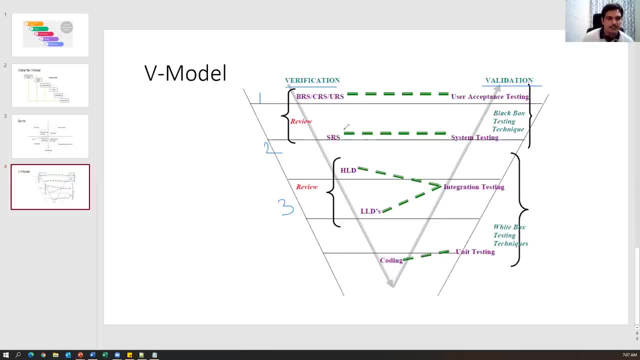 modules. so srs is also prepared by the project managers or product managers. so normally this first phase business unit people will be involved, bu people and srs document will be prepared by product manager or we can say project manager, pm. we can say pm. okay, they will write these. 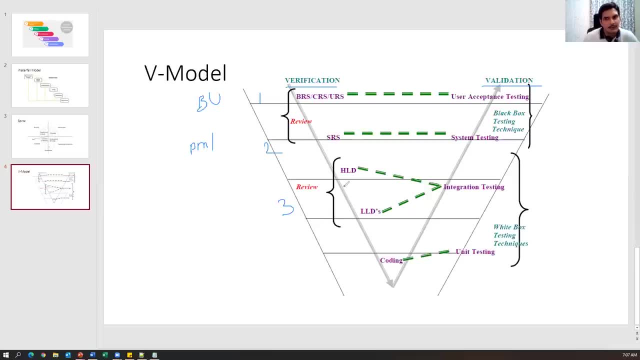 requirements and hld and lld documents will be prepared by the designers. hld and lld documents will prepare by the designers. right, this is just a documentation which contains a different pictures and diagrammatic picture. they will represent the software, so hld contains a main. 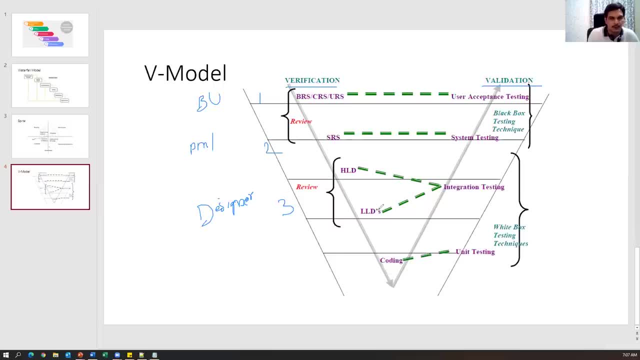 modules. lld contains a low level modules. the main modules will be divided into multiple sub models and then coding will start. so design requirement module. so first two phases: one, two comes under requirement phases and three comes under design phase and coding is a fourth stage. here the 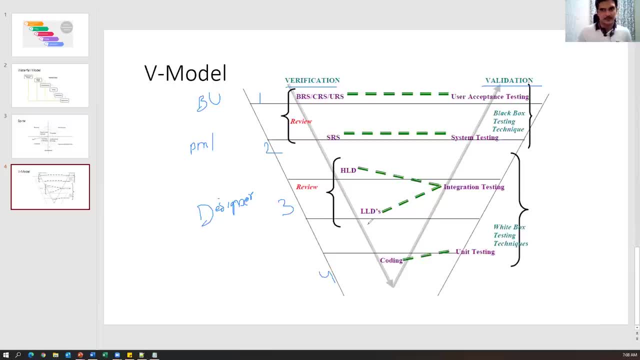 development will start, coding will start based on the documents. okay, this is one part. now come to the other side. this is all comes under verification. So, as i said, one important point here in the v model: in every phase, srs means what software requirement specification? okay, which is developed, which is written by the product managers, right? 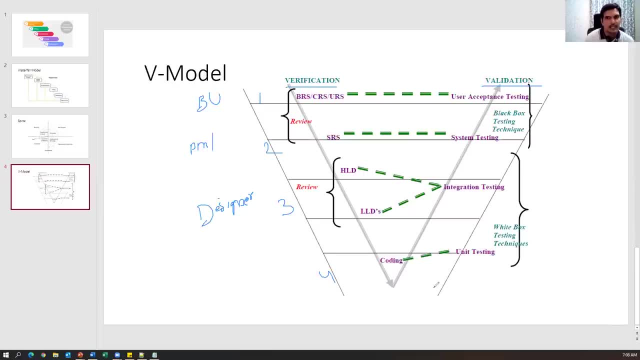 so, if i just look at this, as i said, one important point: every stage we have a testing in v model. in every stage we have a testing like requirement phase- we conduct testing. design phase- we conduct testing and coding phase- we conduct testing. Right, But where exactly we conduct testing? 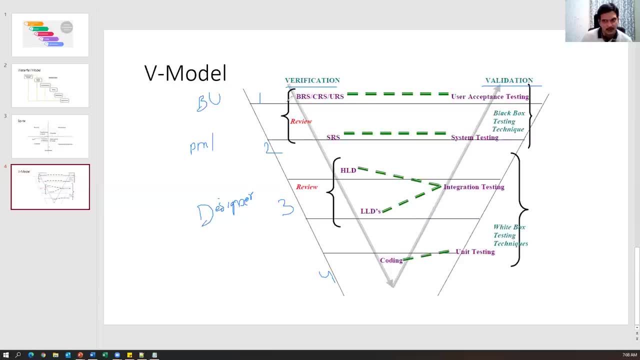 So in the first phase, as soon as we have done this document, business unit we conduct, or the same team is conducting, some reviews on the document. So here, in this particular stages, whatever testing we are going to conduct- and we will conduct this testing again- 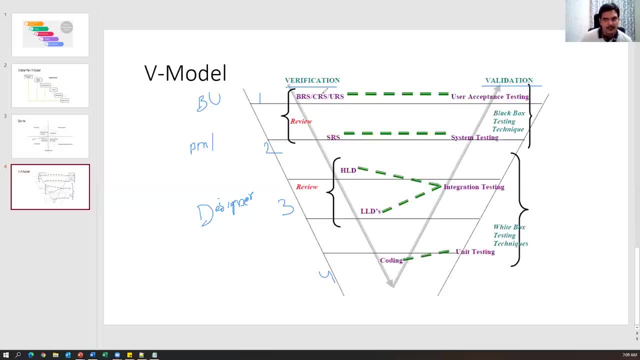 Not testers. OK, every team member, suppose in the BRS or in the first phase, Whoever is prepared these documents, and they are responsible for conducting the testing. So they review the document to ensure the correctness and completeness. So what they will review: the document is correct or not? 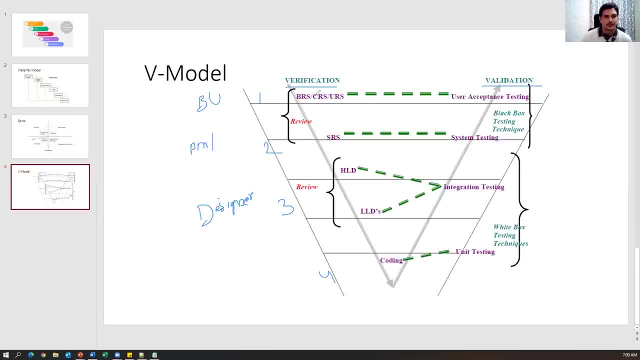 So whatever the content they have mentioned in the document which is correct or not, And if it is correct, then complete or not, all the requirements are mentioned in the document or not. So that will be verified. That is a kind of testing. 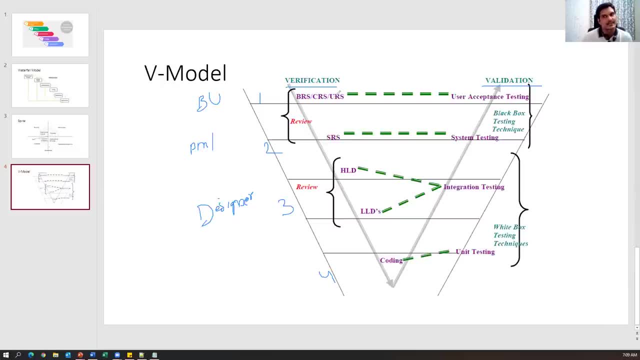 We are not exactly Testing the software. we are testing the documentation, because if the document is correct, the next phase will be easy or there are no chance. like next phase, We will not get any bugs or any issues because the next phase will follow, based on the previous phase. 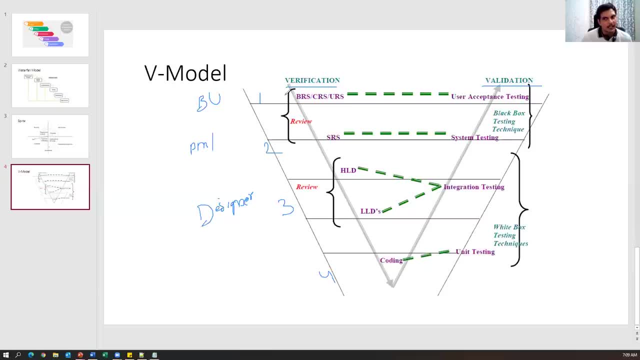 So if here the document is very clear, correct and complete, then rest of the phases will go on. So in the first phase, while preparing BRS or CRS, URS, the BU team, the people who are involved in the BU. 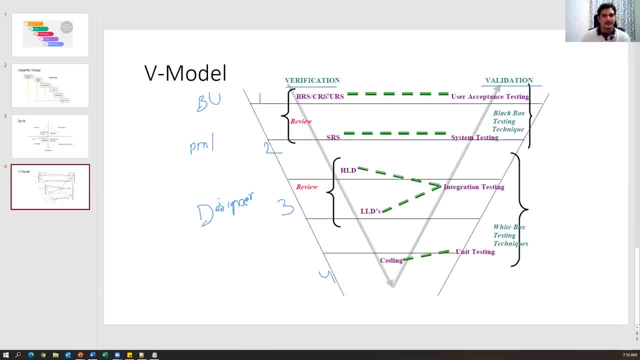 They will conduct some reviews on this document And that is a kind of testing review. And what is review means? Review means to ensure the document is correct and complete. Correctness and completeness of the document will be tested in the form of review. 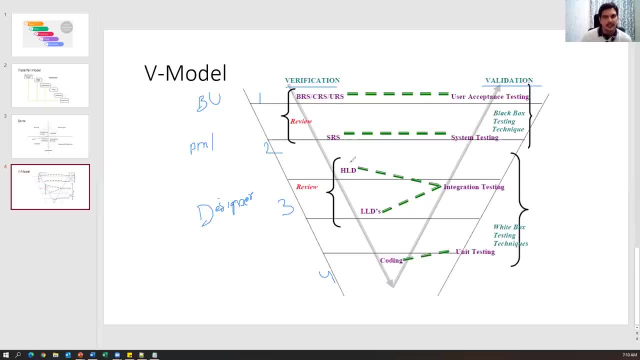 And the second stage: SRS document, LLD document, HLE- these are also documents, So we conduct some reviews on the documents to check whether they are correct or complete. So in that context these phases also include testing in the form of reviews. 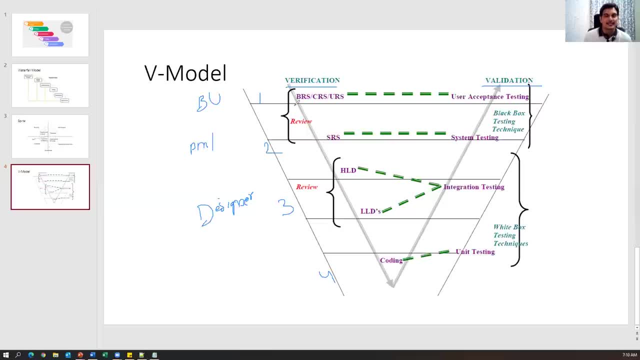 We are not exactly testing the software. We are testing the documentation part, We are testing the documents. OK, that is a review, not only review. There are three other things also there. We call as a. let me just write the notes. 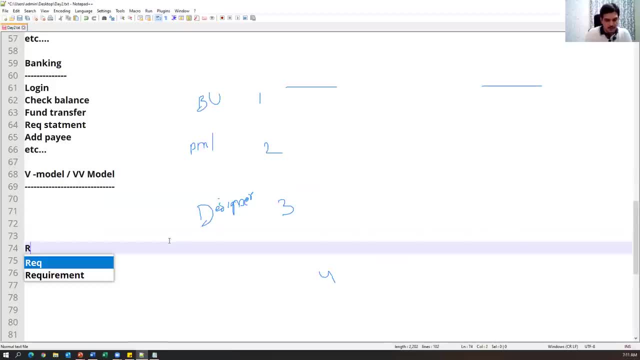 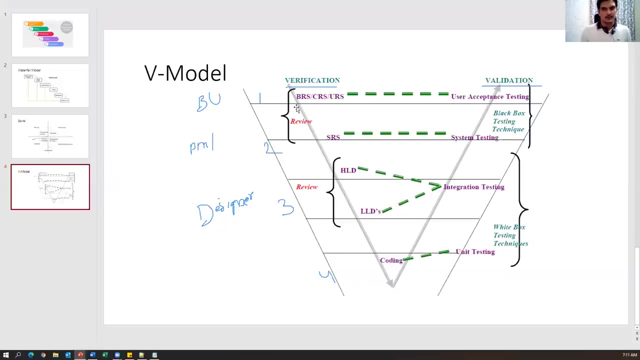 OK, so here there are a lot of points are included, guys. So I'm talking About review and also we have something called walk through. We also something called inspection, inspection. So actually these are the techniques for testing. So by using review or by using walk through, or we can, by using inspection, we conduct testing on this documents. 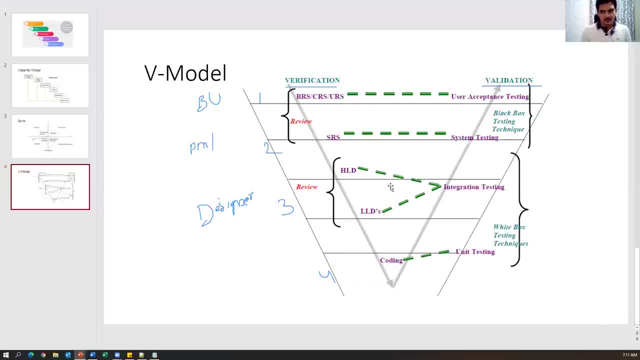 So we are as SRS, HLD, LLD. So if you want to test these documents, we use either reviews or we use some walk through Or we use some inspection. So these three are testing techniques To verify the documents. 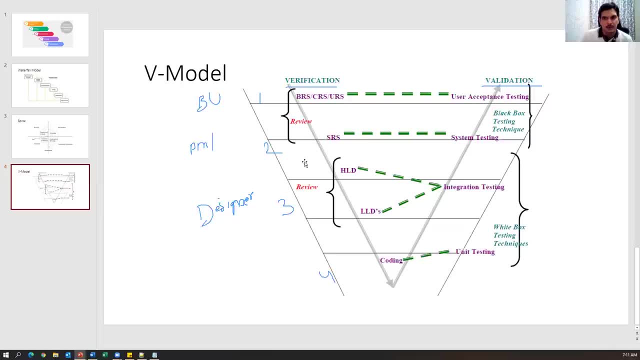 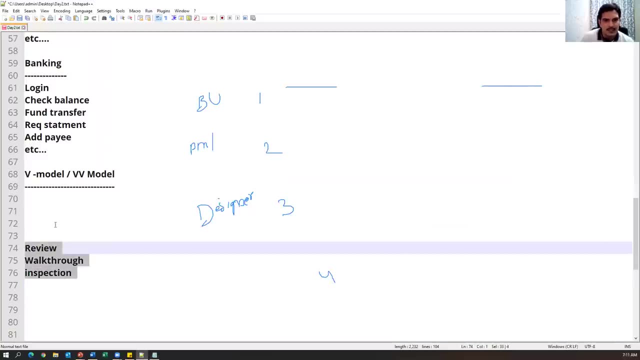 OK, I'll discuss in detail, Just hold on. So here I just mentioned only review, but actually there are three things we have. So review, walk through and inspection. So by using these three techniques we will verify the documents, not exactly the software. 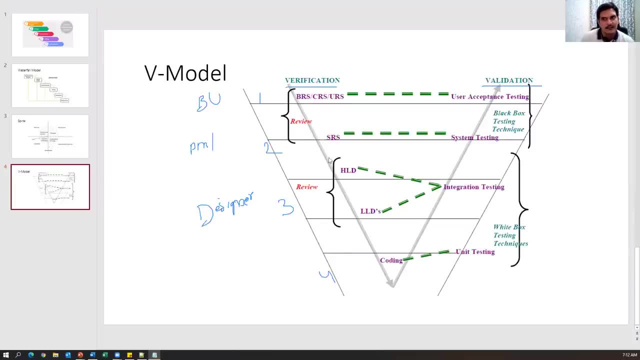 OK. so in that context, we have testing in every phase. We review the BRS document, we review the SRS, we review the HLD, we review the LLD And in the coding part, actual software will be ready. 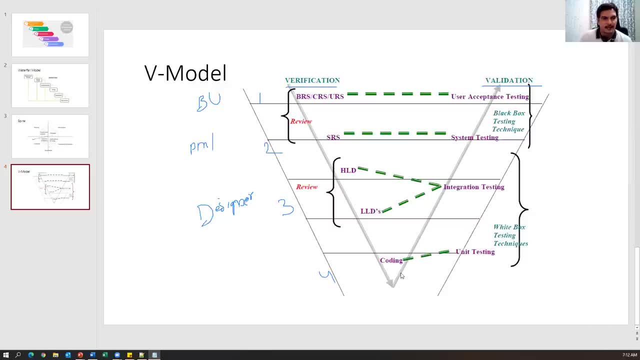 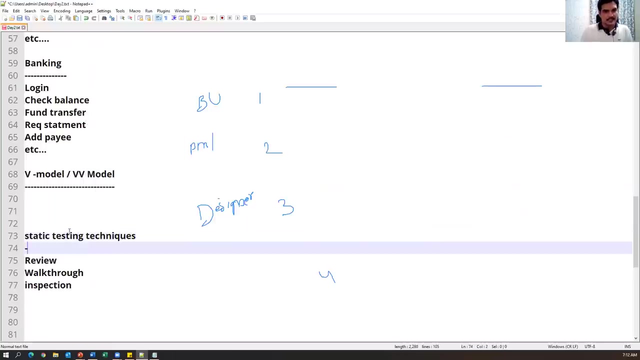 So where exactly software is developing in the coding phase. until and unless we enter into the coding phase, we just have only documents. So whatever testing we conduct on these documents, which is basically called as static testing techniques- So here understand this Static testing techniques we are calling as a static testing. 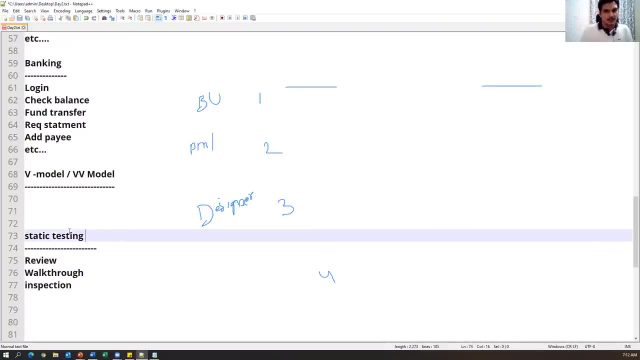 So what is static testing means testing the documents. testing the documents, testing the project related documents is called as static testing. Remember, it is very important. So testing the project related documents is called a static testing. So testing the project related documents in the form of reviews, walkthroughs, inspections is called as a static testing. 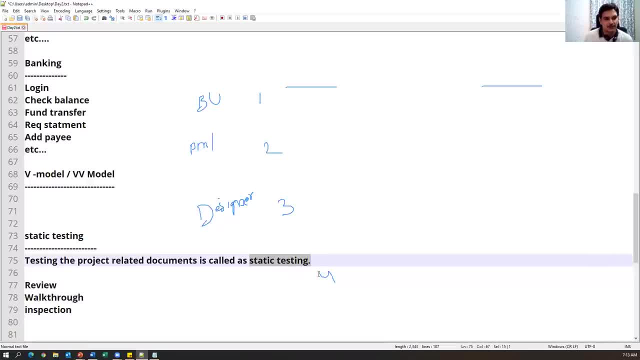 Static means what? we are not exactly testing the software, We are just testing the documents in the form of reviews, walkthroughs and inspections. in the form of reviews, walkthroughs and inspection, We are testing the documents, so which is called as a static testing, which is called as a static testing. 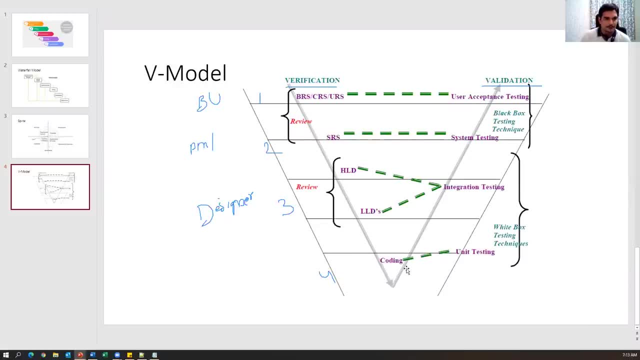 So remember, guys, now comes under coding. once the coding is started slowly, the software will be ready. so the coding will be done. first some modules will be developed and after developing multiple modules, they will integrate those modules. and after integration of the modules we will conduct one more testing. 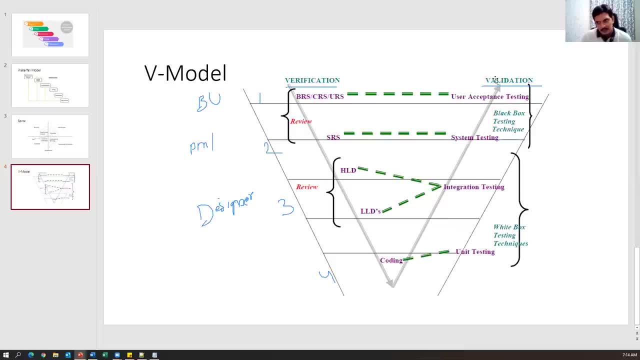 so here in this side, if i just look at another side of validation, we can see four levels again: unit testing, integration testing, system testing, user acceptance testing. okay, this part is called validation part. so what is unit testing means? whatever the module which is developed by the developer, as i said before, the entire software will not be developed at one shot. the software 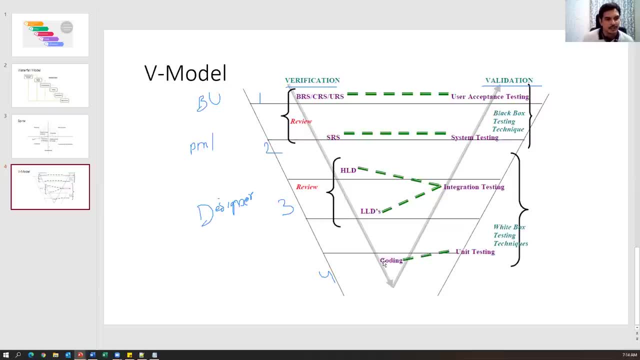 will be divided into main modules and sub modules. so first developer will start developing the software with single module, a small single module, so whatever module which is developed by the developer, if you test that particular module which is called as a unit testing, simply we can say unit testing in the sense testing the single module or single component. 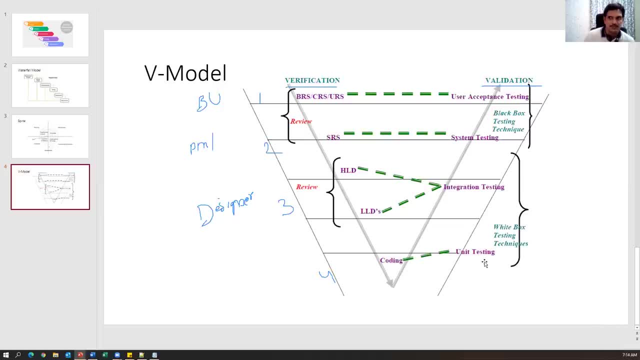 of your software, which is called as a unit testing. so who will conduct this unit testing? developer himself should conduct the unit testing because they know the coding part, they know how they have written the code, so they know exactly how the module is working. so the after completion of 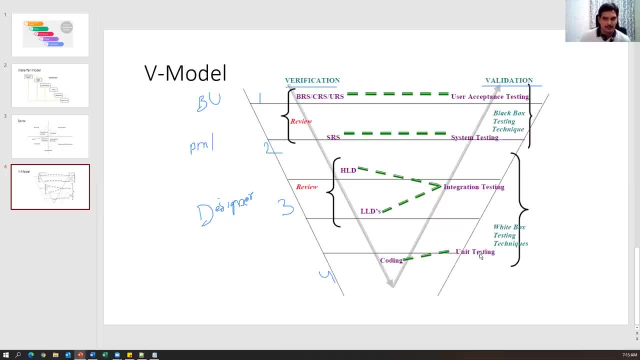 coding. first, unit testing will be conducted by the developers. after that they will integrate the modules. all the modules will be integrated and they will make one main module. then we'll test that module, which is called as integration testing. so after completion of all the modules, we will 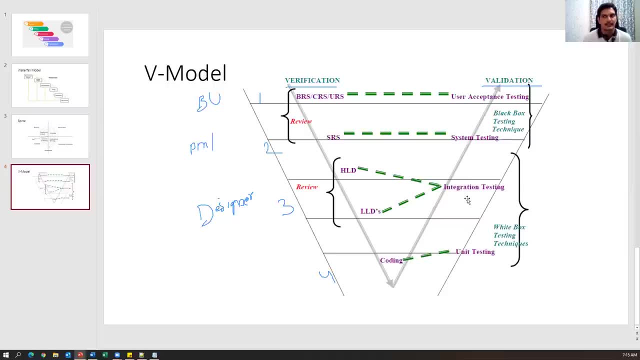 conduct one more testing called integration testing. after completion of integration, we will conduct the integration test and these two- unit testing and integration testing- conducted by the developers itself: developers itself because they know exactly how module works, because they are the developers, they are the, they are developed, the code. 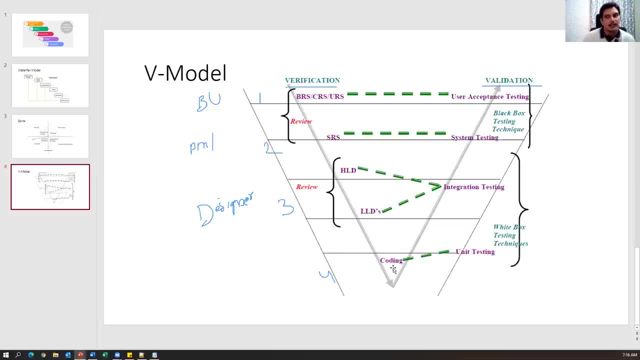 so coding. after completion of coding, the sub modules and main modules will be tested by the developers himself in the form of unit testing and integration test, and these two testings. if you want to conduct these two testings, you have to know the coding part. okay, you have to know the programming knowledge. 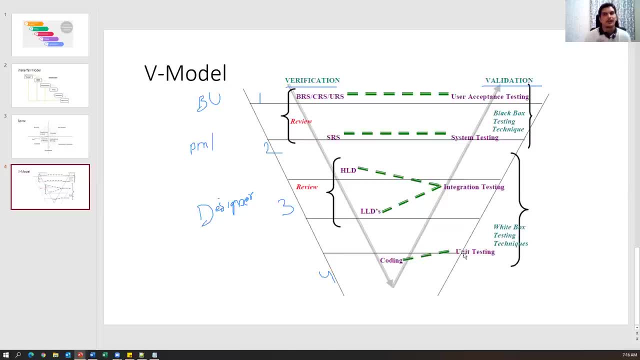 and what exactly developers are written inside the module. you have to understand that. but who can understand that testers doesn't have programming knowledge? so who is responsible for implementing the implementing or develop the module? i'll just highlight a few examples. so, for example, in our test session- but this was a test- 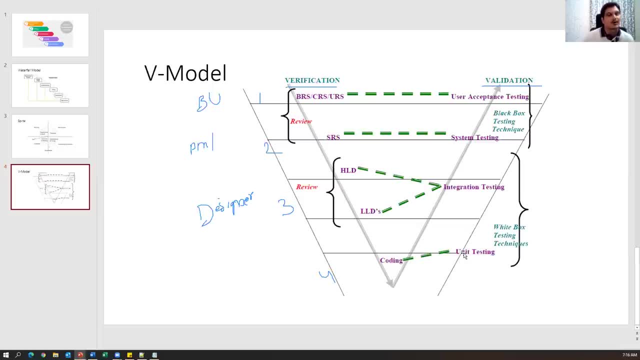 session that was called as virtual testing. okay, so first you have the test. you have to in develop the module. you have to know only the program definition, meaning you have to remember only the properties of the module. you have to know what's inside the module if it's computer. 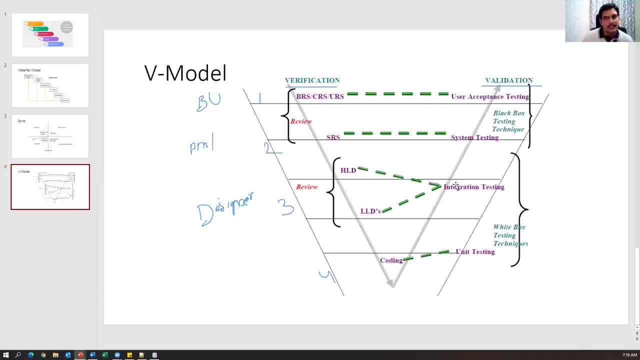 software user interactions. you have to ask your campus. its a separate source for all the modules. you have to understand that those modules are where the code is being embedded in what we need to efective, develop and use it. so it's up to you when you estos a test or get to know a module we were 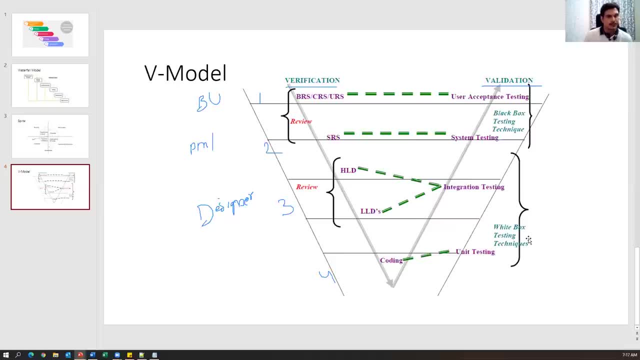 we have to know internal logic of the programs. if you want to test the module single module, we have to know what type of code the developers have written. so that's the reason these testings will not be conducted by the testers. these testings will be conducted by the developers. 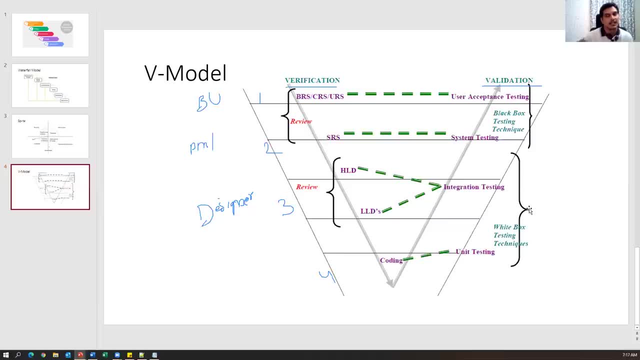 himself. that's the reason we can call them as a white box testing. so white box testing means what white box? if i just put white box, you know exactly what is there inside the box, right? so that is the reason. so white box testing means what we have to know: internal logic of the program and 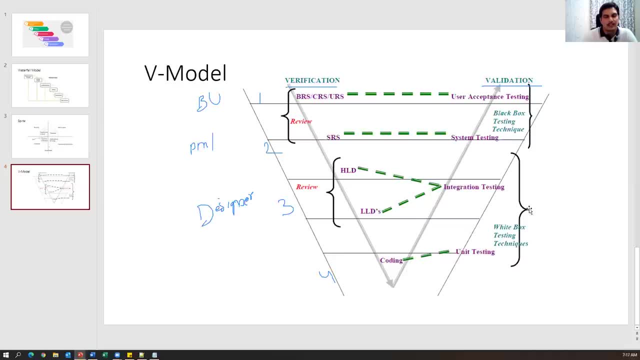 what is a program they have written for that model. so that will be known only by the by the developer, so they can conduct this testing. so after completion of the sub modules they conduct unit testing on single module and after integrating all the modules they conduct integration, integration testing, which is also done by the developers After completion of integration. 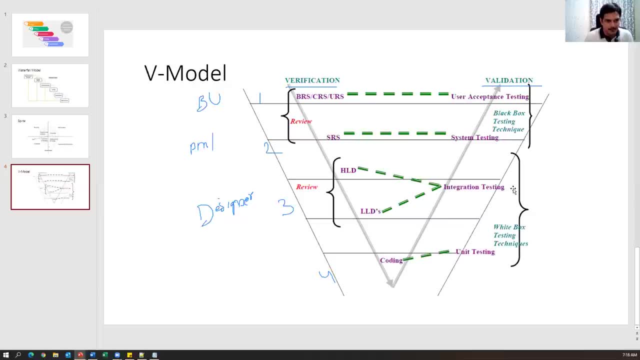 testing. the final software will be ready, The final integrated software will be ready, and that software will be given to the testing team. Then system testing will be conducted by the testers. So here system testing phase will come into picture. So here the testers. 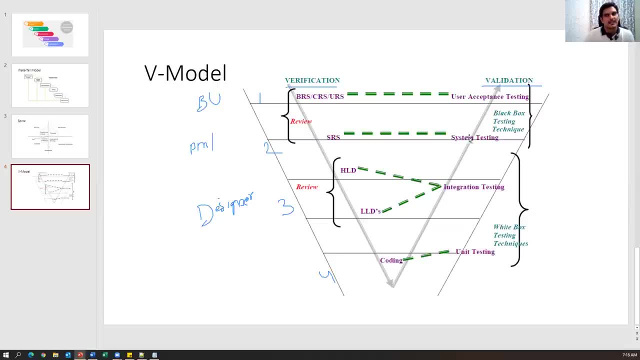 will involve to test the software. But what kind of testing they do? What is system testing here? Basically, they don't need to understand the code. They will just verify or test our software is working according to customer requirement or not. So what customer is expected? 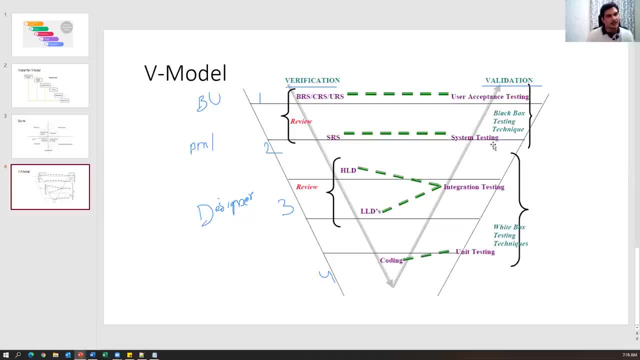 what are the flaws we have? what is the functionality? whether is working or not, That will be tested in the system testing phase. So here we don't need to understand the code, We don't need to have programming skill in the system testing phase and actual testers are involved in the 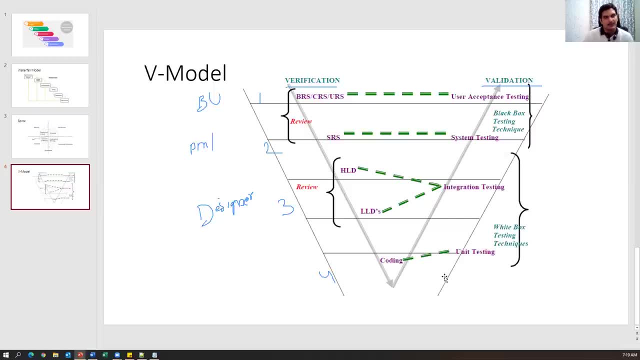 system testing phase and rest of the testings will be done by the respective people. but in the system testing phase, whatever testing we are conducting, done by the testers. okay, we don't need programming knowledge here, because we are getting the complete application. we don't know exactly what developer. 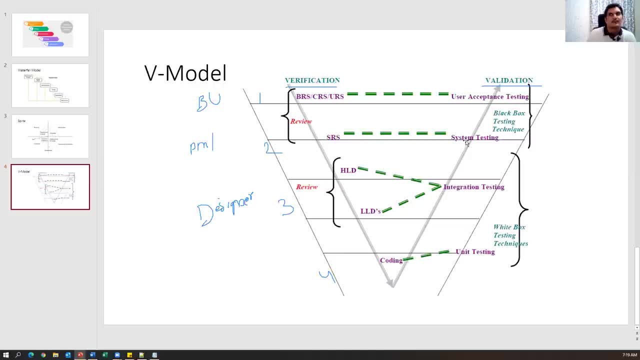 has written internally. we don't know the code. that is the reason we can call it as a black box testing technique. what is black box means? black box means we don't know exactly what is inside the box. what is there inside the box, right? so system testing comes under black box testing. 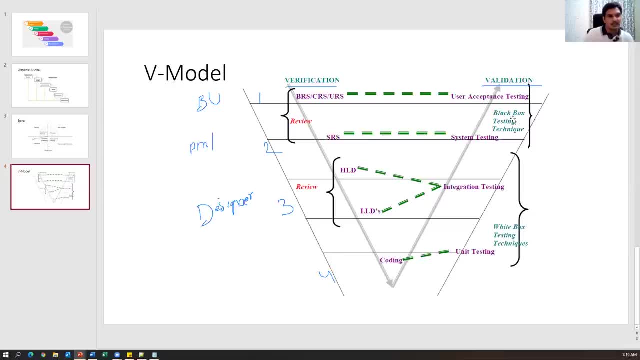 technique, because we don't know exactly what developer is written internally. we are just testing the application or testing the software whether it is working according to customer requirement or not, whether it is satisfying the customer requirement or not. so as a user point of view, how functionality is working. i'll test that so that comes under the system testing. there is a 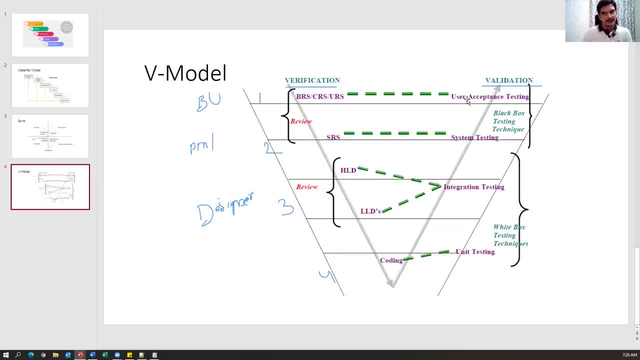 next level of testing and the last phase is user acceptance testing. after completion of system testing, user or customer will do some kind of testing at their level. that is user acceptance testing. this is also done by the testers along with customers, uead testing, and here also we don't. 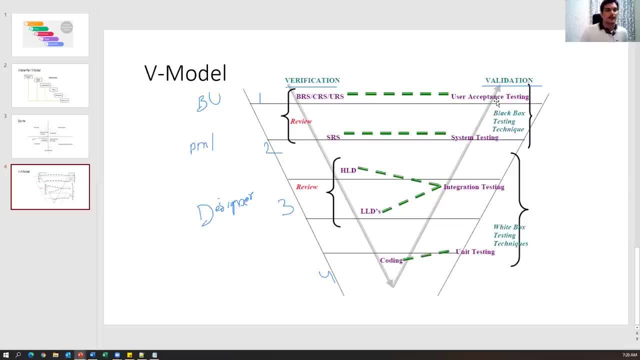 need to understand the code. so which is also comes under black box testing. okay, now observe this carefully. let us start with the brs document, then srs will be prepared, then hld and lls will be prepared. so these first one, two, three phases are document level. so in each and every phase we conduct testing in the 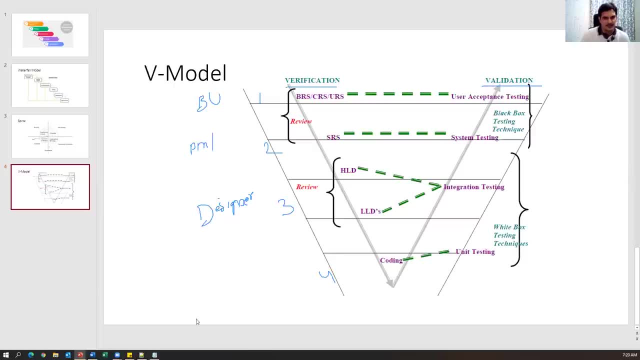 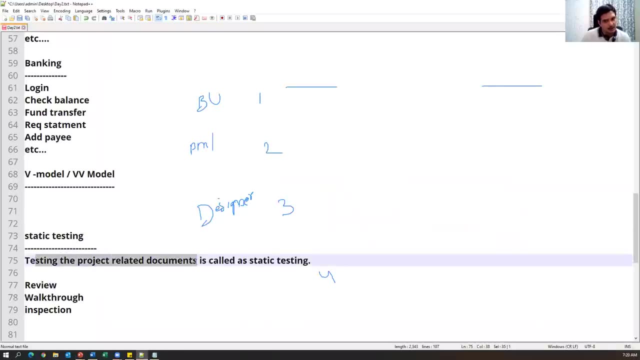 form of reviews, work throughs and inspections. so that is called as a static testing. static testing, in the sense testing the project related documents, is called as a static testing. and what are the techniques we use? review, walk through, inspection. so these are the three techniques we have to use. 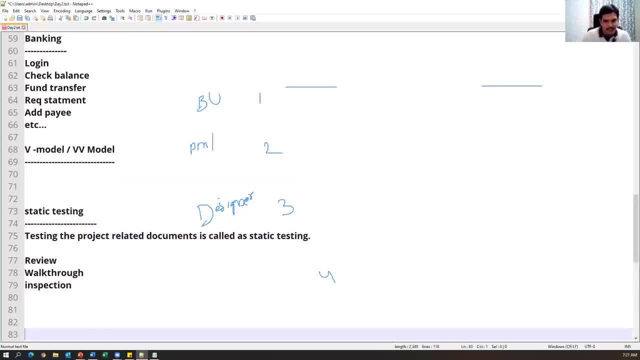 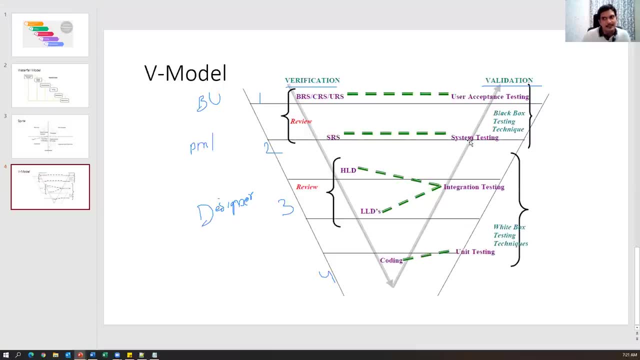 to perform the static testing. now, the other side: if i just look at here, whatever testing we are doing here- unit testing, integration testing, system testing, user accept testing- where exactly we are doing this testing on the software? because at the coding stage the software will be developed. after developing the software we are doing these kind of testings. so these tests, these kind of 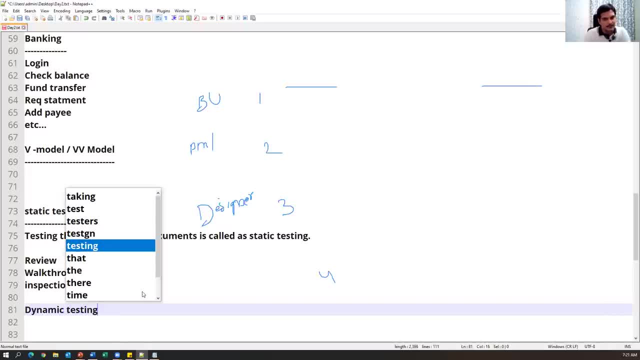 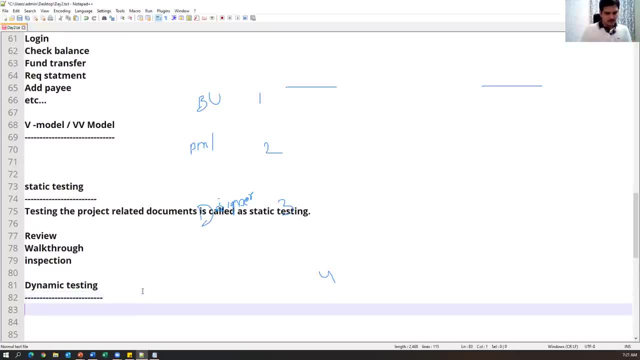 testings are called dynamic testing. dynamic testing in the sense we are actually testing the softwares, not the documentation. okay, so the dynamic testing means testing the actual software, testing the actual software. okay, but in the static testing we are testing the project related documents in the form of reviews, walkthroughs and inspections. when you come to the dynamic testing, we are: 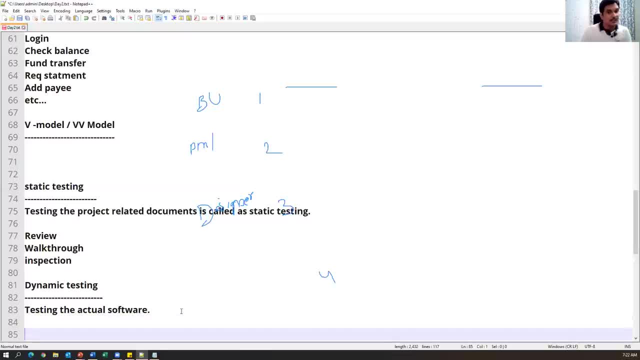 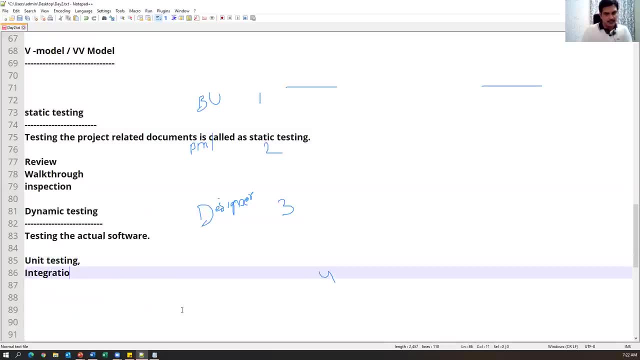 testing the actual software. but what are the techniques we are using here? we are using unit testing technique and we are using integration testing. we are using system testing. we are using uat testing, user acceptance testing. okay, these are the different techniques which we have to use in dynamic testing and these are the 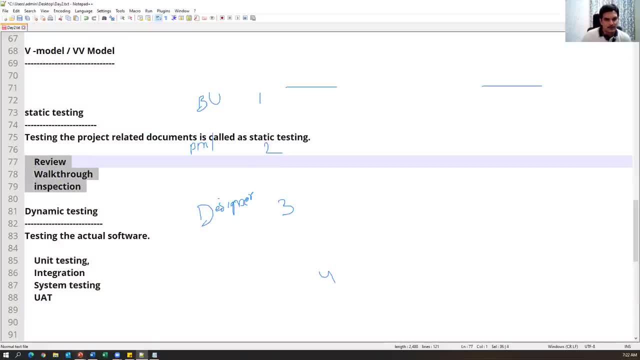 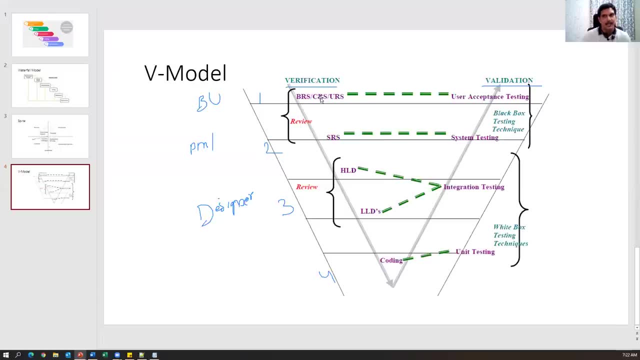 techniques we use in static techniques. so in the v model, one side, we can call it static testing. so just verifying the documentation part and verifying the actual software which is called as a dynamic test, understood, guys? so static testing and dynamic testing, because until, unless we enter into the 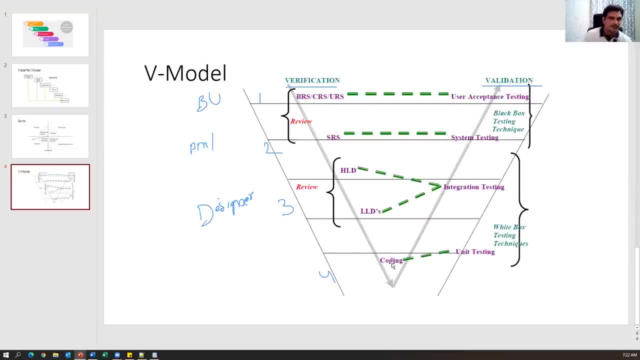 coding part. actual software is not ready. and what is there for testing? only documentation is there. so we review the document, srs hld, lld. so this is a kind of a testing. after completion of the coding software will be ready, then we will conduct unit testing, integration testing system testing and. 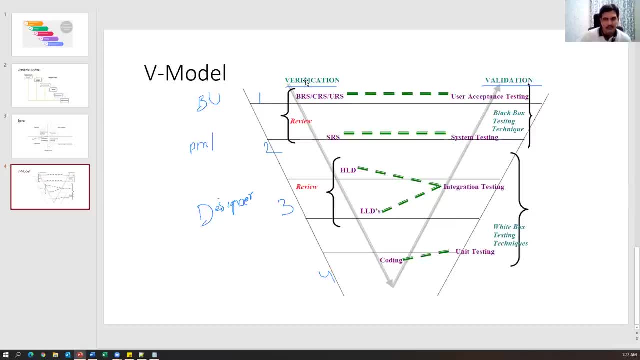 uat testing. so one side, the reviews, inspections, walkthroughs are comes under static testing techniques and unit testing, integration testing, system testing, uit testing comes under dynamic testing techniques, which is called as a dynamic testing techniques, and again, unit testing, integration testing. if you want to conduct, we have to know the coding part, we have to know the. 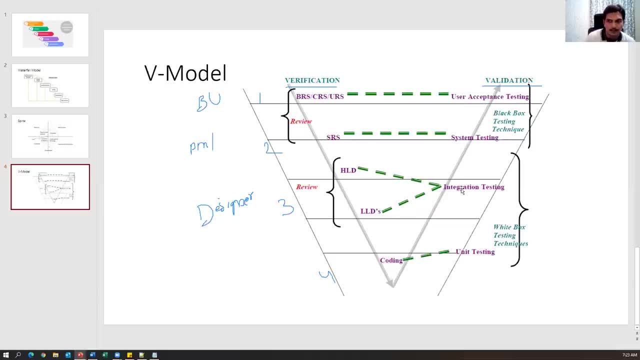 programming knowledge. we have to know, we have to have the programming knowledge. so that is the reason we can call them as a white box testing technique. integration testing, unit testing, comes under white box testing, because we have to test what is there in that model, what kind of code they have. basically, we are testing. 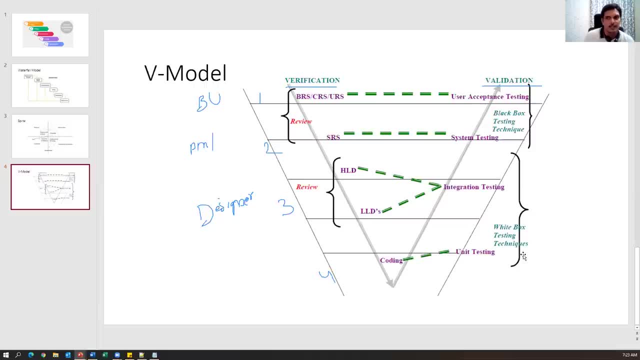 the code, not exactly application. we are testing the code. so the developers will conduct unit testing and integration testing, and after completion of integration test testing, then testers will involve. what testers will do? testers will perform system testing and here actually we are verifying whether software is working according to customer requirement or not. so 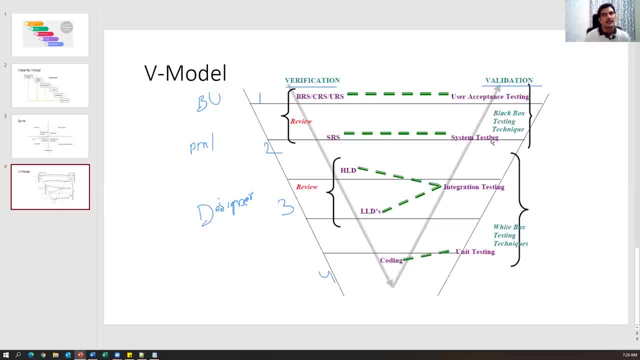 during the system testing. what testers will do? they will understand the requirements. they will write the test plan. they will write the test cases. they will execute the test cases. they will find the defects. they report the defects to the developer. so all these activities will be done during system testing phase. so that that is a tester job. actual testers will be involved during. 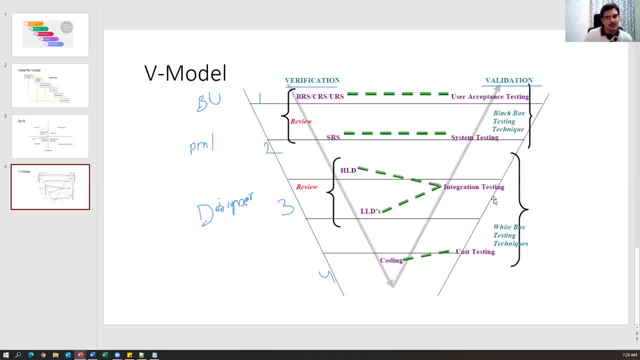 system testing phase. but integration testing, unit testing, is also done by the developers because they have to know the code, so they know the coding part. so if you know the coding then you can also do integration and unit testing. but as a tester most of the time we don't know exactly what developer has written internally. 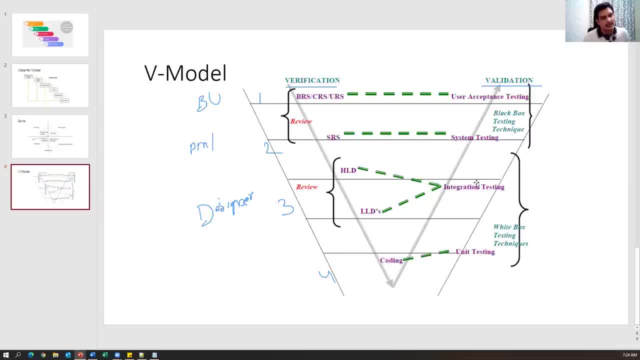 so that is the reason: integration unit testing is always done by the developers and system testing will be done by the testers, and user acceptance testing will be done by the testers along with the users or customers, because, uh, what is the end users here? end user is nothing. 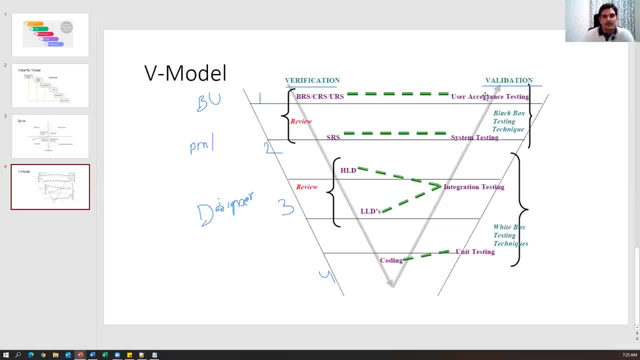 but finally, who is using the software? they are called the end users and finally, they are called the end users. end users, so they have to know how to use the software. so they will also do some kind of testing before using that software in their environment. so testers also will help them. 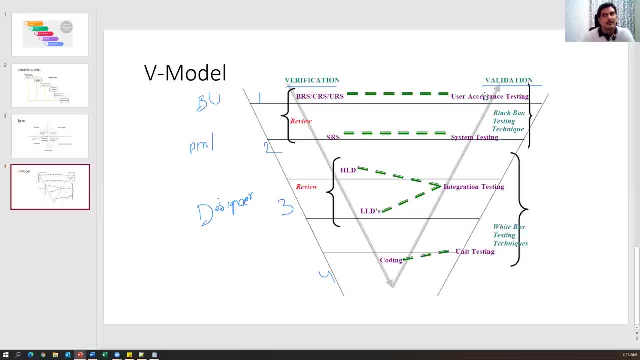 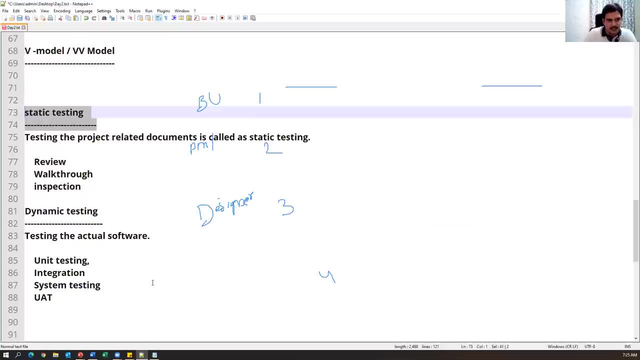 and collectively, testers as well as customers sit together and do some kind of basic testing, which is comes under UAT testing, user acceptance testing. okay, right, so we have understood one side, which is static testing. other side is a dynamic testing. now let us understand what is verification and validation. let me just clear it. I already told you verification and 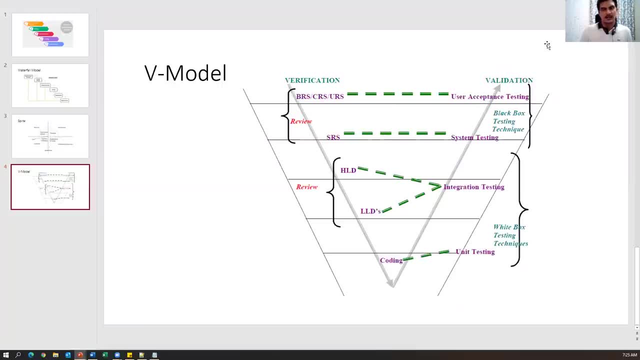 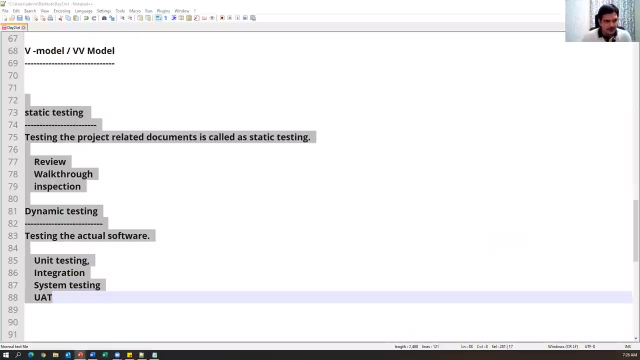 validation. if I just look at, this part is verification, this part is validation. this is very, very important question in interview guys. please focus on this. what is verification, what is validation? it again depends on these two things, okay, okay. so verification and validation. observe this carefully. I am writing some notes here. 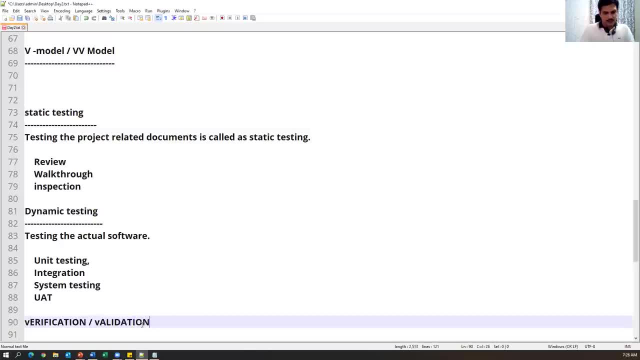 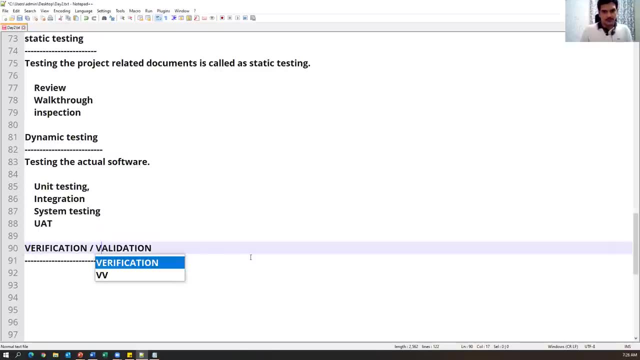 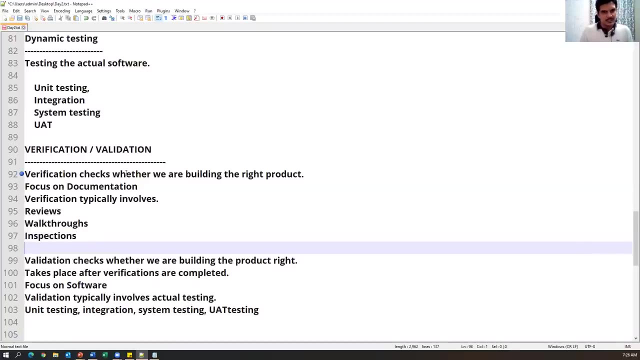 verification and validation. what is the difference between verification and validation? so this is verification and validation. let me put some important points. okay, so verification checks whether we are building the right product. verification checks whether we are building the right product. verification: we are verifying each and every stage. if I just look at the v model, we prepare vibrant and we are checking. the document is. 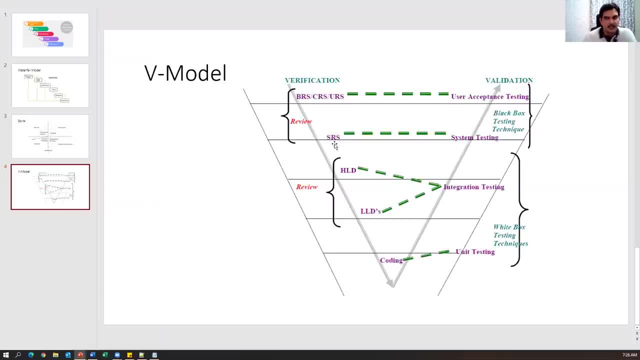 correct or not. then again we prepare srs document. again we are checking which is correct or not, which is prepared well or not, and then a HLD document, then LLD document. what exactly we are doing here? in every stage we are checking each and every document is correctly written. 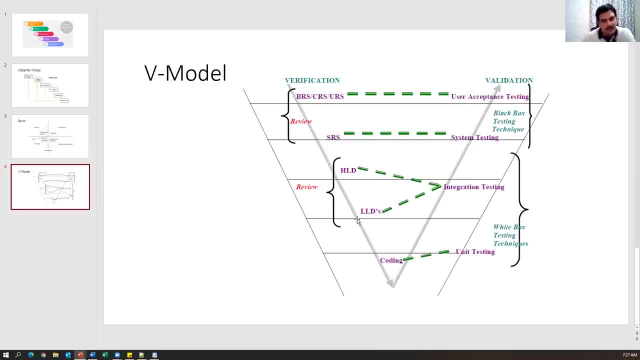 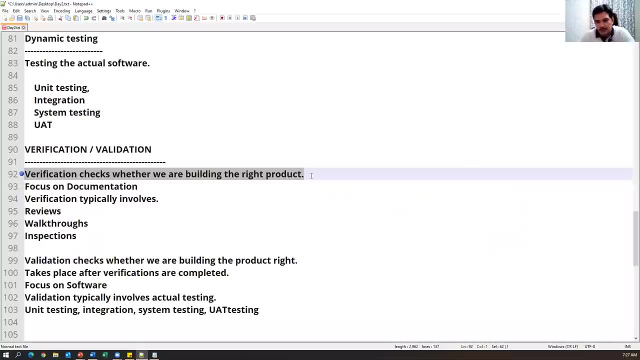 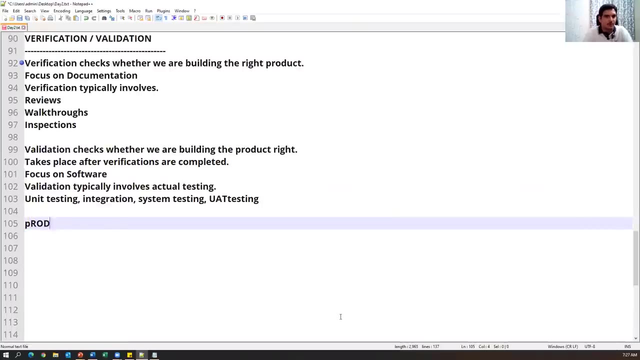 or completely written or not, And this is called as a verification. So verification means what Checks whether we are building the right product. whatever we are doing is correct or not. Suppose what is our ultimate goal. Our ultimate goal is to develop some product. 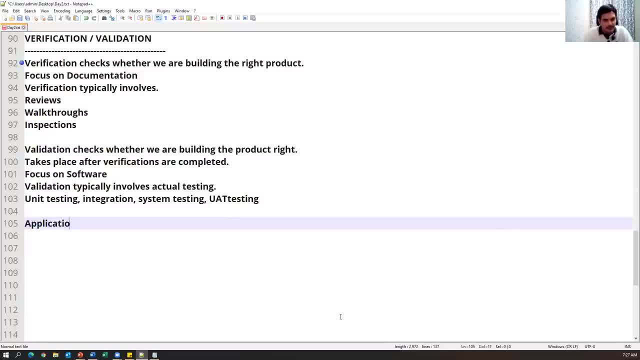 to develop the application. To develop this application, we have to follow certain process. like different stages we have to follow, I'll say, stage one and then stage two and then stage three, and so on, So then we will finally achieve the application. 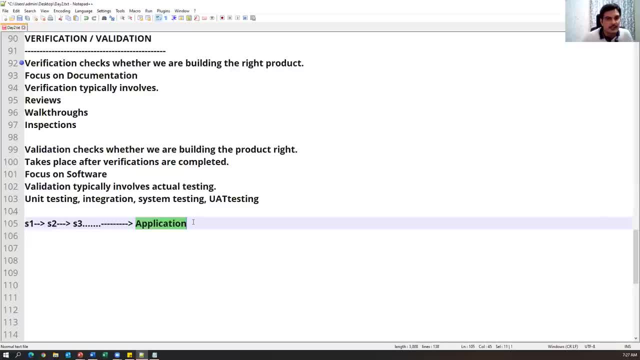 We finally will develop the application. So what verification is representing? whatever activities we are doing in every phase, which are correct or not we are doing correctly or not, we are implementing the product correctly or not, that comes under the verification part. Okay, each and every verification, everyone can do that. 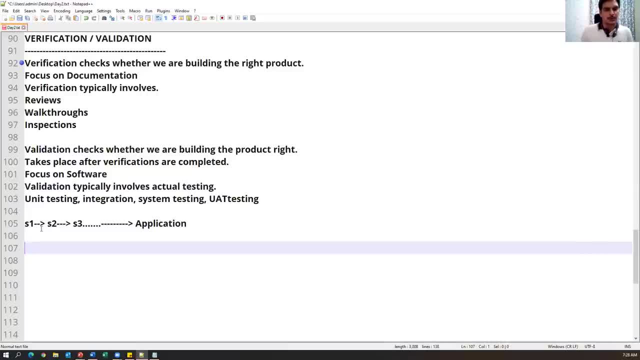 Everyone can do that verification. Suppose: if I give some document to you, you can verify that, And if I give some document to the developer, developer can verify that. So anyone can do the verification. So what is meant by verification? Whatever activities we are doing in every phase, 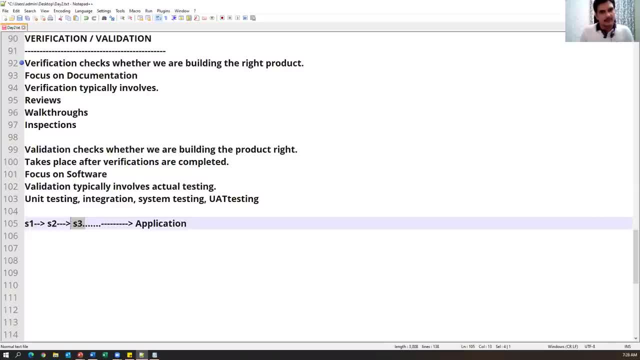 are correct or not we are doing correctly or not. that is verification. So if I just look at the definition once again. so here validation checks whether we are building the right product. Whether we are building the right product means what We are doing correctly or not. 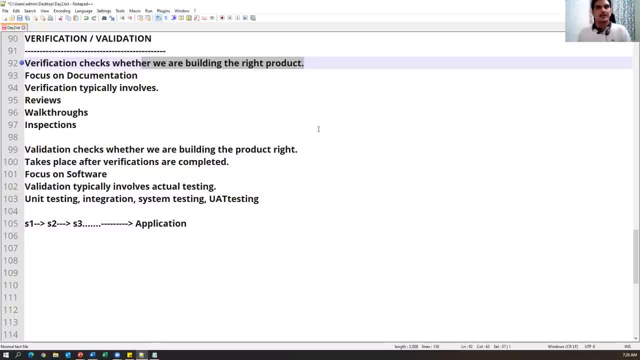 We are following proper process, correctly or not. Each and every step we are verify And here we mainly focus on the documentation. Okay, in the verification we are mainly verify the documentation Where verification comes under, when verification come into picture. If you have some document, I'll verify that. 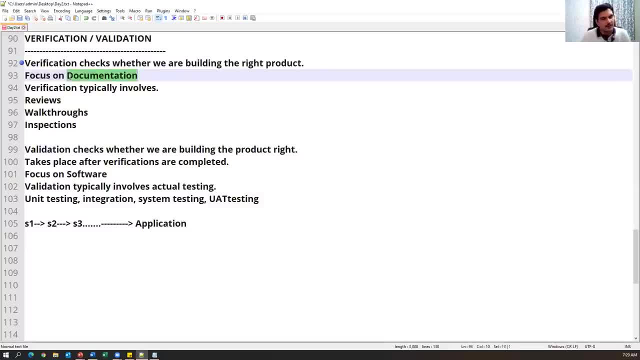 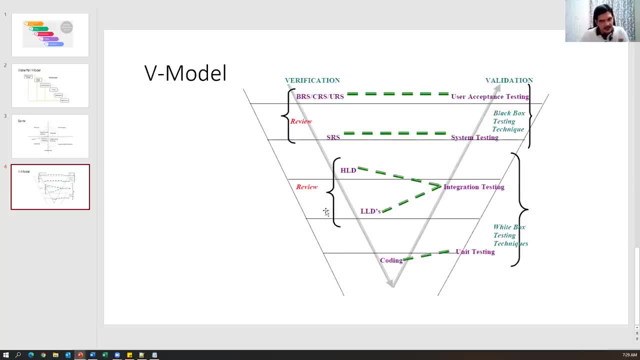 So verification always focus on documentation And if I just look at it, if you look at this picture once again in this particular stage, BRS, SRS, HLD and LLD. So these are all documents, These are all documents. 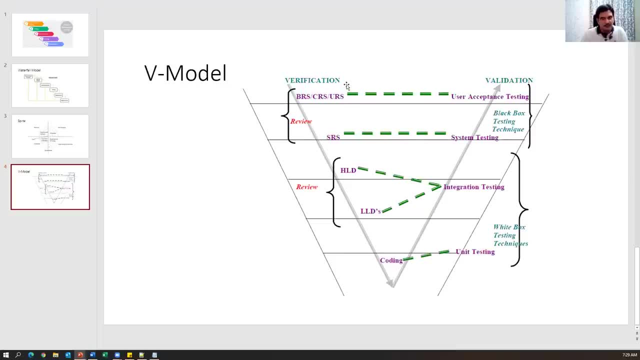 We are conducting testing on these documents, So this comes under the verification part. We are checking each and every document is right or wrong. We are checking each and document is having proper content or not. So that is verification. So these phases comes under verification. 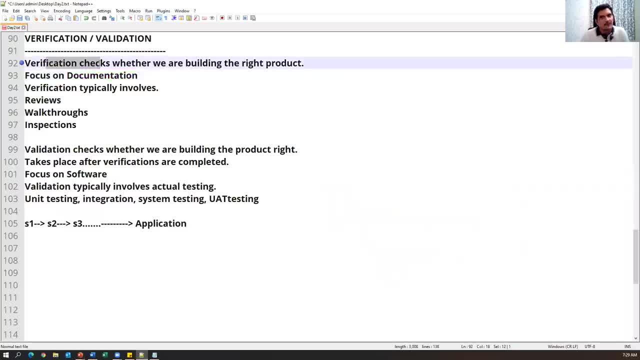 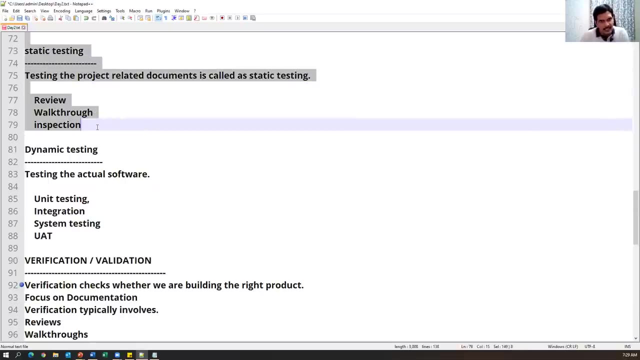 That's the first thing. So verification checks whether we are building the right product or not And focus on the document, And verification typically involves, again, reviews, fluxes, inspection. Whatever the static testing techniques we have used, the same techniques we'll use in verification also. 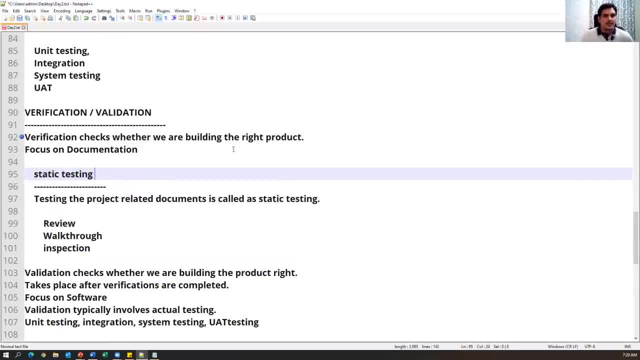 Same thing. So this comes under verification. So static testing techniques will be used in verification process. Okay, these two are interrelated. So verification checks whether we are we are building the right product. It mainly focus on the documentation And we use static testing techniques. 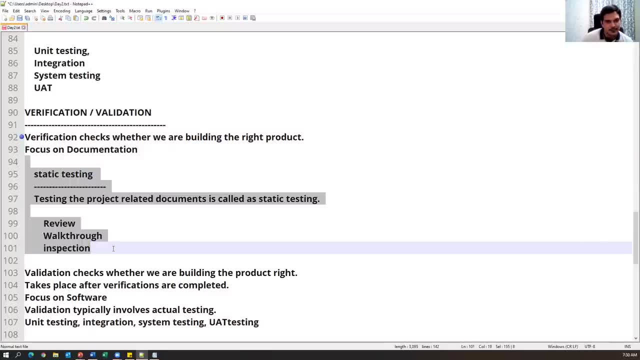 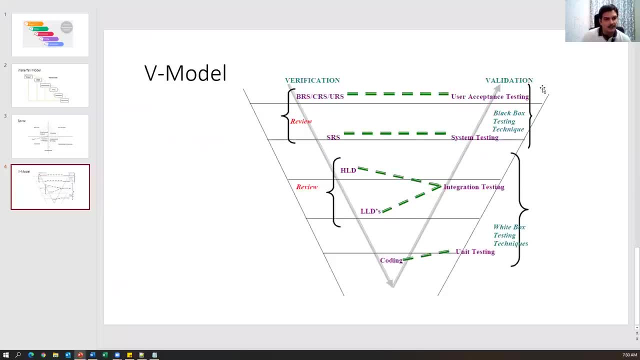 to perform the verification Because it is a document. Now come to the validation, The other side, if I just look at this: the validation When. to perform validation Once the software is ready. Here we are actually testing the software During unit testing, integration testing. 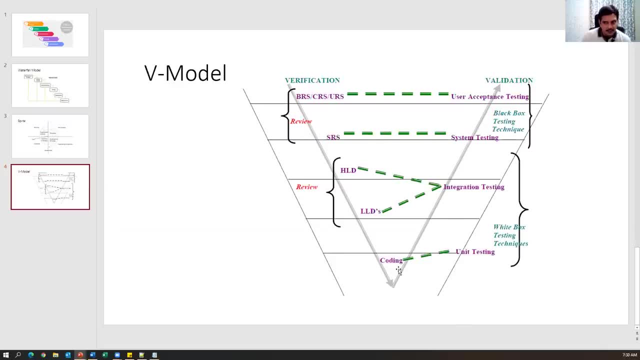 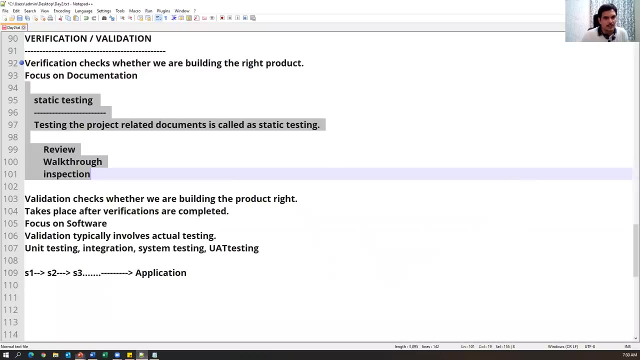 system testing, UAT testing. What exactly you are testing Here? we are testing the software. Once the coding is completed, software is ready, So we are testing the software. So what is validation means? Validation checks actual software working according to customer requirement or not. 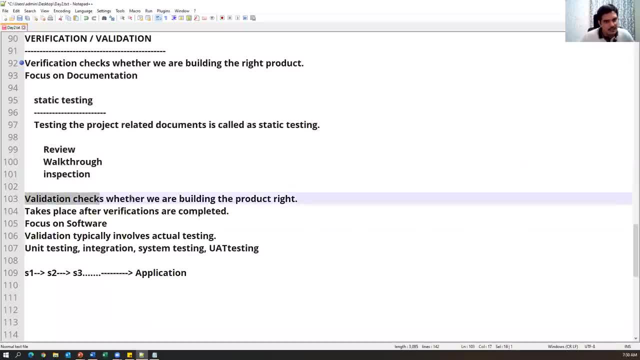 So, if I just look at the definition, validation checks whether we are building the product right. Small difference guys. So validation checks whether we are building the product right. Whatever product we already built, we are building the product We already built, which is right or not. 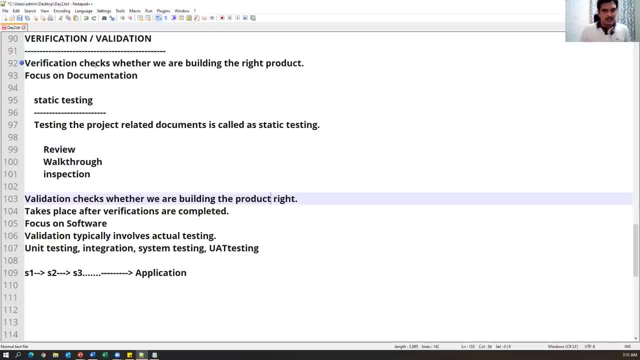 That we are checking here. But in the verification checks whether we are building the right product. But here we are. product is not ready yet. Product is not yet ready. We are just checking the documentation. Are we building the product correctly or not? 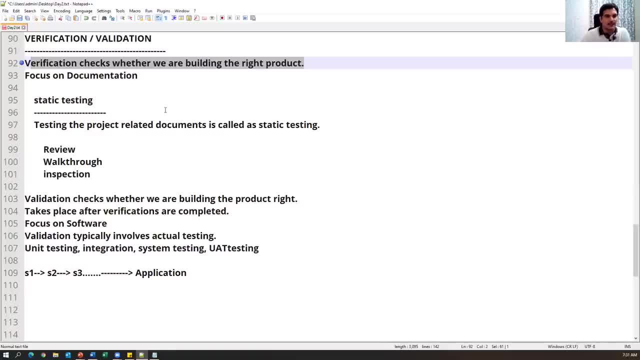 Whatever steps we are involving is correctly going or not. That is a verification part. But once you come to the validation part, once you come to the validation part, product is ready, The software is developed And whatever the software is developed, which is right or right? 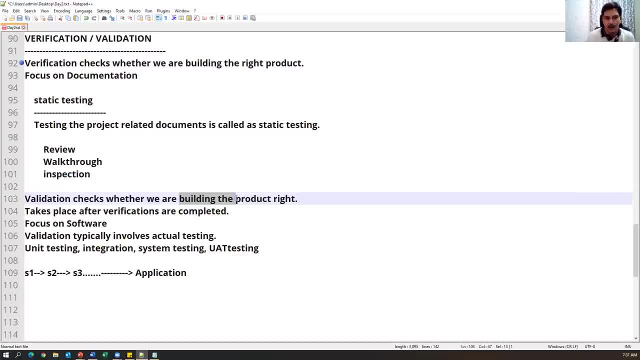 which is right or not, which is working according to customer requirement or not, So that we are testing during validation. So before software is ready we conduct verification. After software is ready, then we do validation And takes place after verifications are completed. 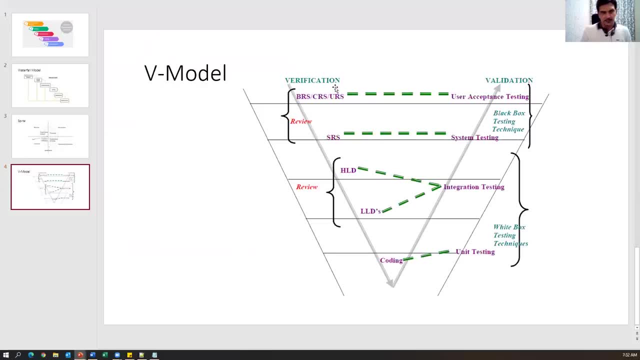 If I just look at this picture once again: after verification phases are completed, then validation phases are started. So after verification phases are completed, then validation phases are started. So after verification phases are completed, then validation phases are started. Unit testing integration system. user acceptance. 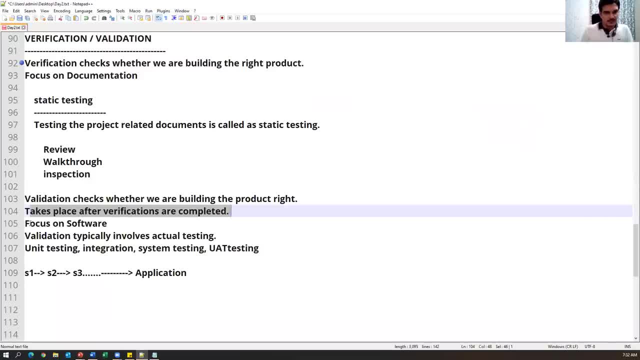 So these testings are comes under validation And which is focused on the software, not the documentation. Verification focus on the documentation. So we use static testing techniques And if you walk through an inspection, But validation, focus on the software, not the documentation. 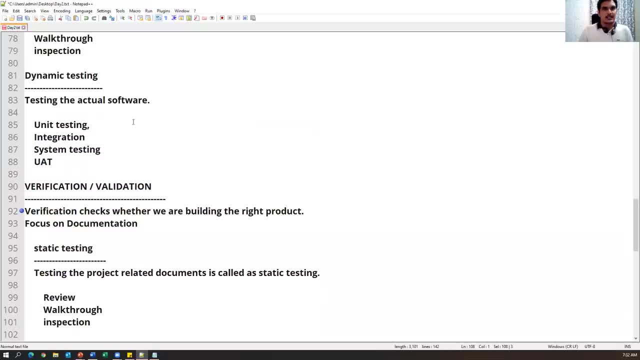 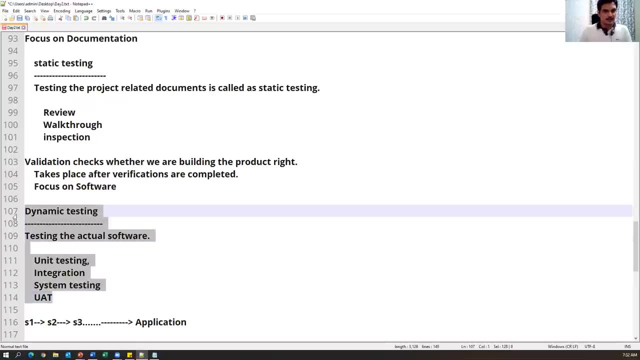 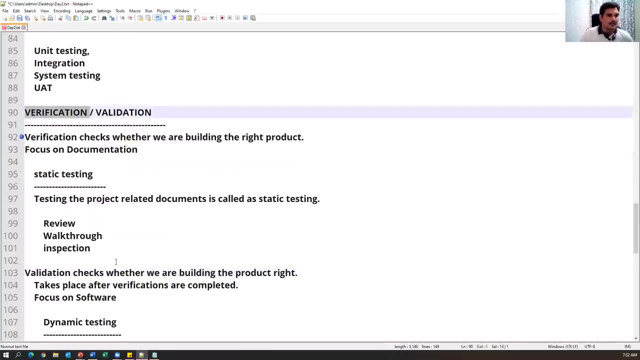 So we use dynamic testing techniques. So, whatever the dynamic testing techniques we use, the dynamic testing techniques we use to conduct the validation. So this is dynamic testing belongs to validation. Static testing is belongs to verification, So validation checks whether we are building the product right. 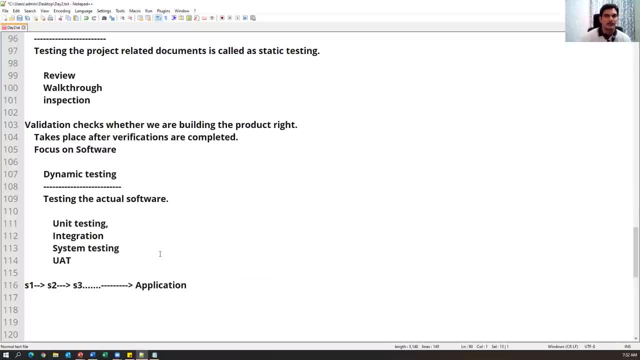 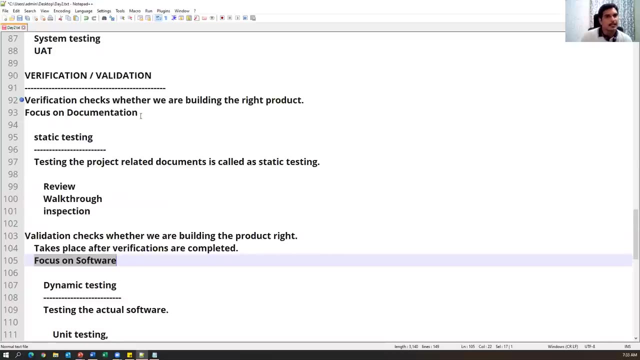 Because by the time product is already built. So whatever the product is built, which is working according to customer requirement or not, which is working properly or not, We are validating it. In that context we are saying validation, So focus on the software and verification, mainly focus. 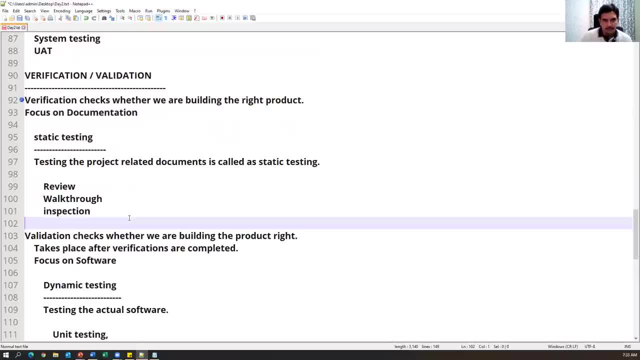 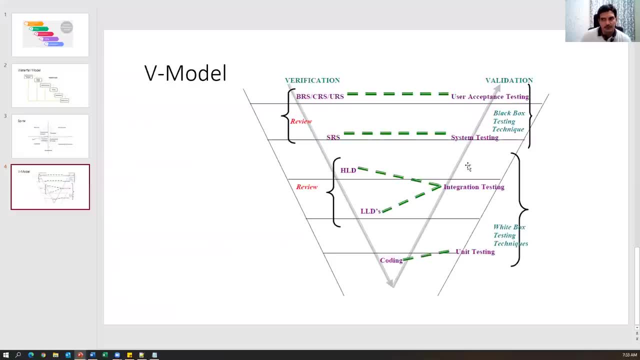 on the documentation part. And so here again, if you come to this picture, white box testing and a black box. So again in four different stages. unit testing and integration testing comes under white box. White box means what We have to know, internal logic of the program. 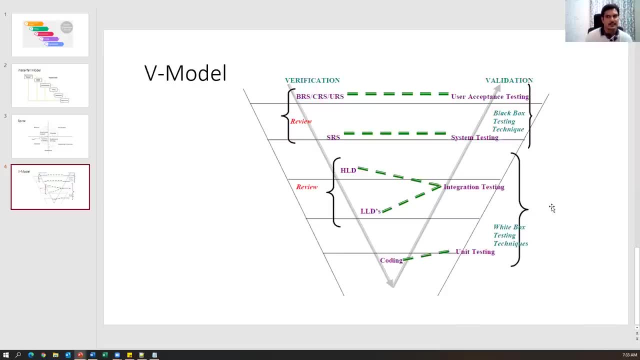 So they are exactly testing the code. They are exactly testing the code, not the application, So which is called as a unit testing and integration testing, And then next level of testing is system testing. After that, next level of testing is user acceptance testing. 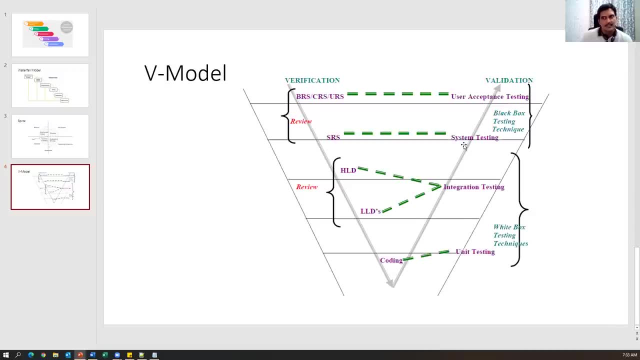 And unit testing. integration testing is done by the developers, System testing is done by the testers. User acceptance testing is done by the testers, as well as users or customers. Okay, So this is a. one part is called verification testing, Other part is validation. 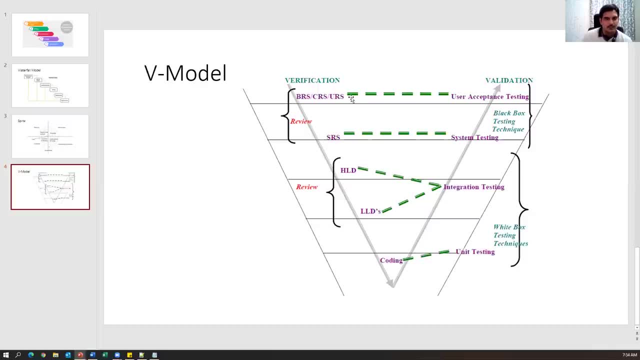 So verification means what We are exactly testing: the documents in the form of reviews, walkthroughs and inspections, which is basically called as a static testing techniques, And in the validation, we are exactly testing the actual software in the form of dynamic testing techniques. 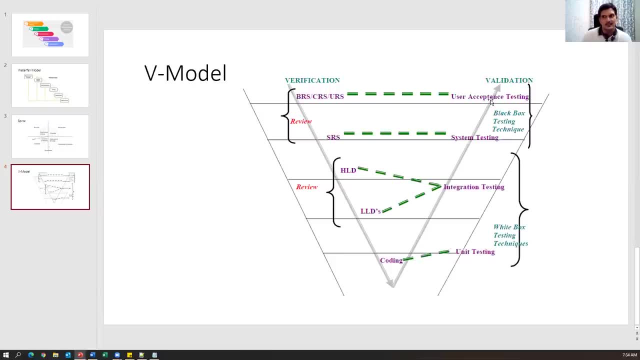 What are they? Unit testing, integration testing, system testing and user acceptance testing. So these are the validation techniques, Or dynamic testing techniques. So these terms are interrelated. guys. If anyone asks you what is the difference between static testing and dynamic testing, 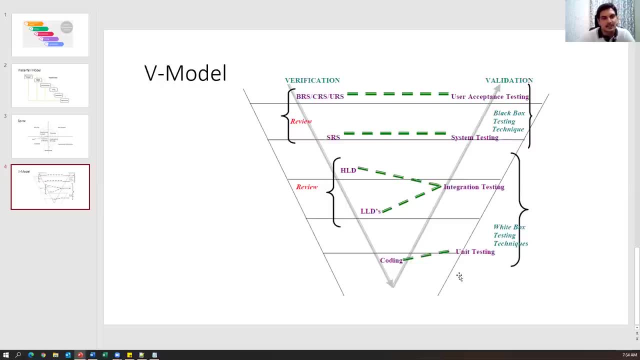 What is the difference? Static testing means we are exactly testing the documents in the form of reviews, walkthroughs and inspections. So what is the? dynamic testing means We are actually testing the software by using unit testing technique, integration system and user acceptance testing. 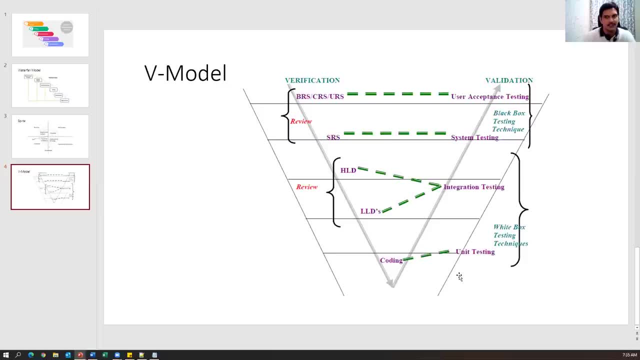 And, similarly, what is the difference between verification and validation? Verification means we are exactly testing the documents, whether we are following right process or not. That is verification part, And we mainly focus on the documentation. Once you come to the validation, we are exactly testing the software, validating the software. 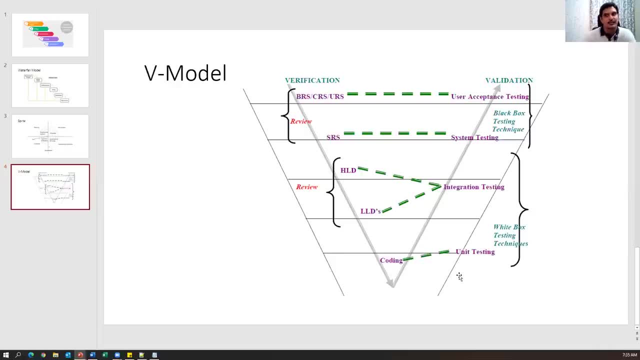 by giving different inputs and observing the outputs, Because by the time software is ready. so we do validation part. So actually testing the software by giving different inputs and getting the output and observing the output Whether it is working or not, Whether it is working or not. 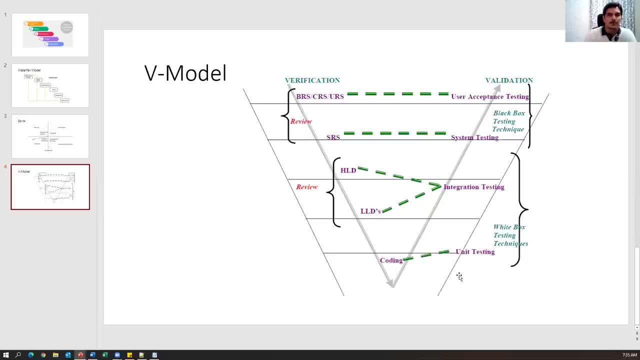 Whether it is a customer requirement or not. That is a validation. So unit testing, integration testing system, user acceptance testing- these testing comes under the validation part, Verification and validation. So verification will be done before software is ready, Validation will be done after software is ready. 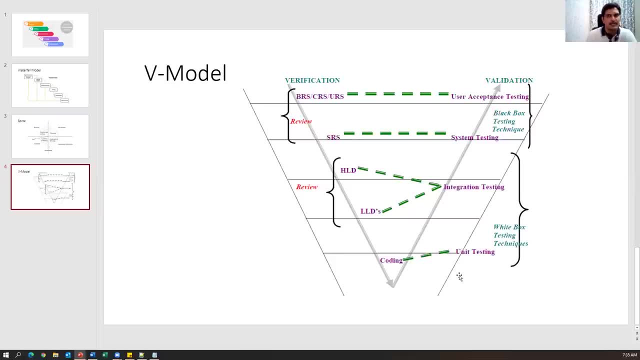 After completion of software development. So static testing is related to verification. Dynamic testing is related to validation. Static- the name itself is static. Static means what Document? Document is always static. Dynamic means always changing, So software is always keep on changing. 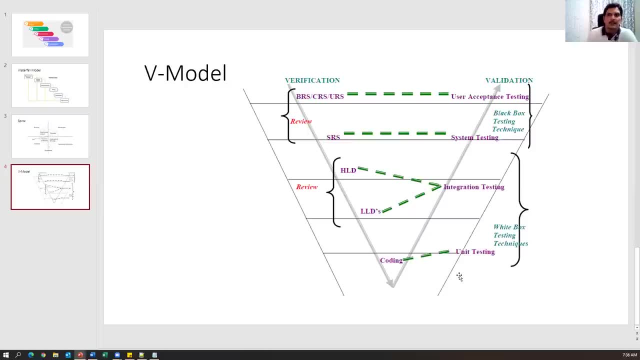 As soon as we added some code or remove a code. So dynamically we can provide some input to the software, We can get some output from the software and we can validate that output. So that is a dynamic test. So these are all important terms which we need to understand from the V model. 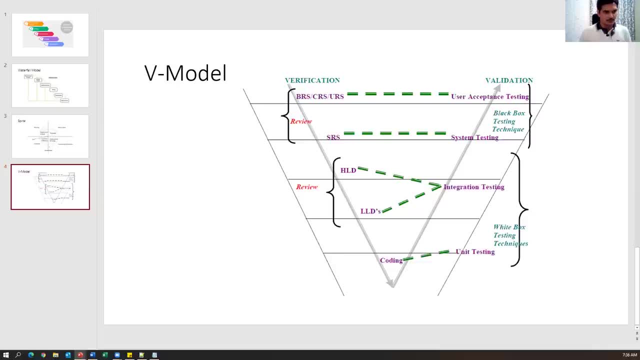 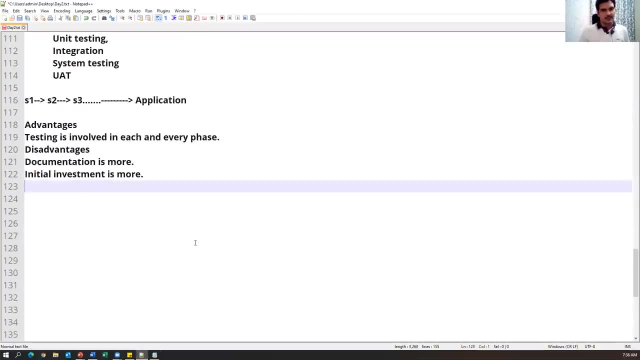 So if I just look at the advantages and disadvantages of V, Let me just put here- and I will also discuss this in detail, guys, in the next sessions- What are the levels of testing, unit testing system testing. So advantages are: testing is involved in each and every phase. 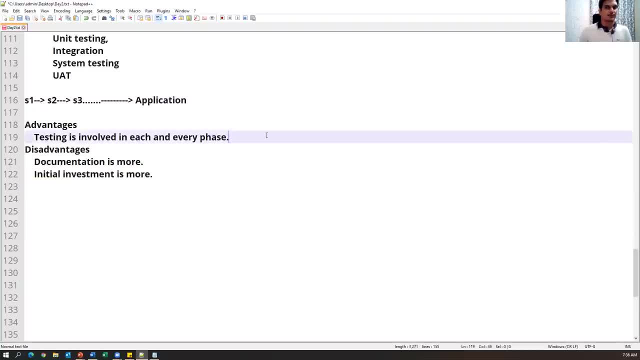 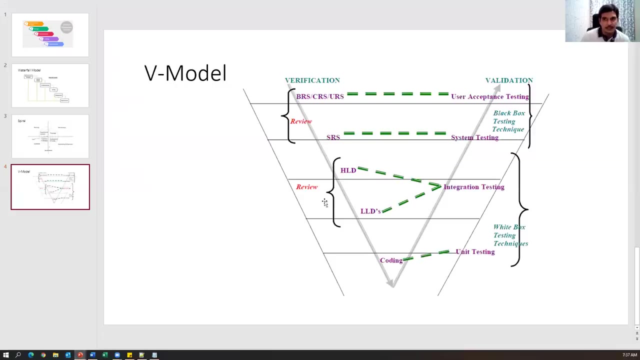 And disadvantages are: documentation is more, because everything is a documentation, And initial investment is also more. That is a disadvantage of V model. Why initial investment is more. Why initial investment is more? because in the V model, all the people have to hide in the beginning itself, along with the developers and testers. 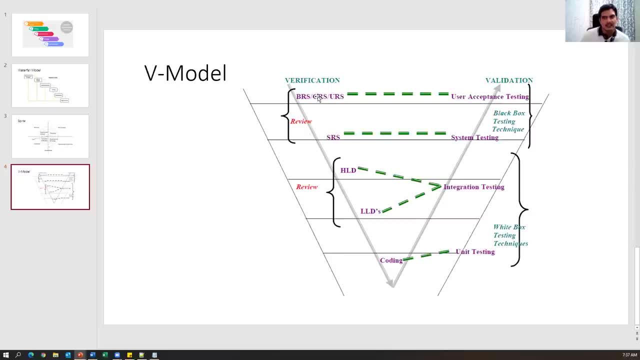 And one more important point, guys, Here the activities will go parallel. Suppose if a coding is there and unit testing will be conducted, And after completion of unit testing, integration testing will be conducted. So what is the input of integration testing? These people will refer these documents. 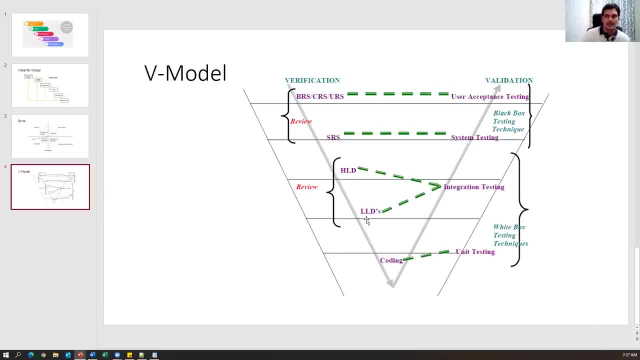 LLD and HLD documents are having main modules and sub modules. So in integration testing what we will do, we will conduct- we are checking the communication between the modules and those modules are interacting properly or not. inputs are properly taking or not? are we getting proper output or not? 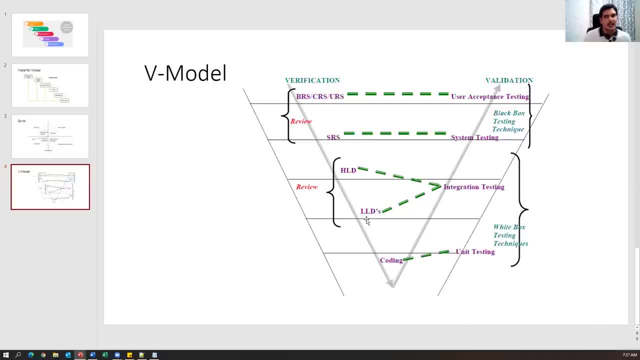 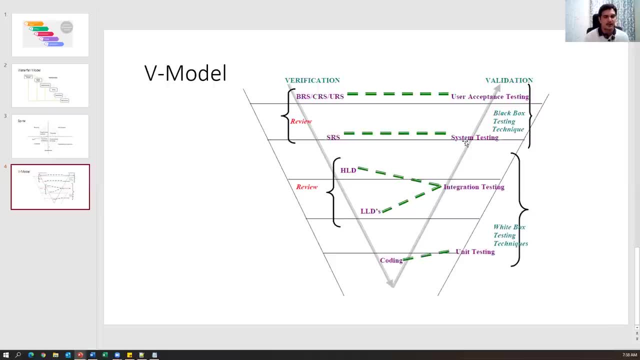 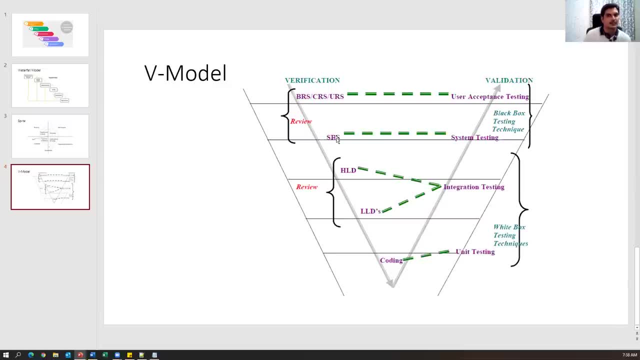 information, we need SRS document, that is the input document for us to perform system testing. Similarly, to perform user acceptance testing, they will refer BRS document. So in every stage of testing we need some input. Okay, So here Available, Available. 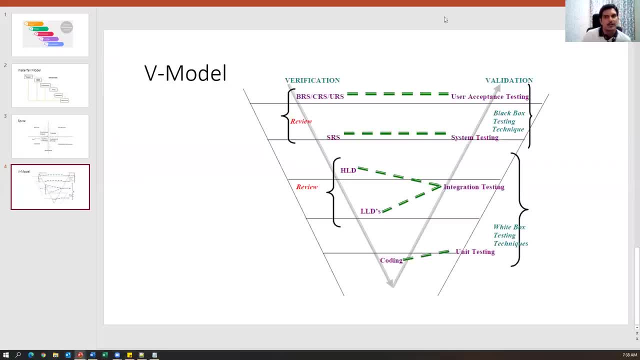 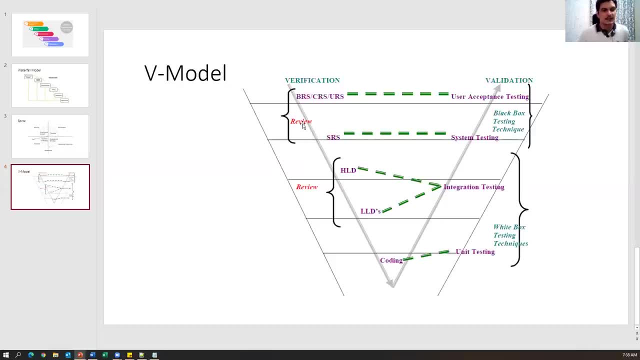 Because in every phase, suppose in the first phase, reviews in the sense everybody will, probably everybody will conduct the review's, Review's, Walkthroughs. inspection means developers as well as tests. everybody will involved in that. In that page we have to hire the people at the beginning itself, before starting a software. 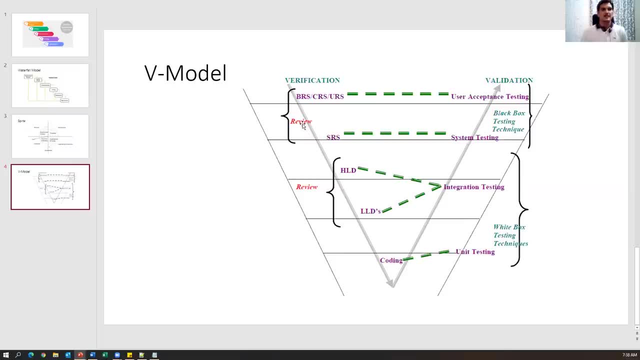 development issues we have to have developers and tester. But in Waterfowl model is not like that. After completion of few number of phases, the tests will be higher than all the moving few number of phases. the testers will be hired, But here the testers and developers. 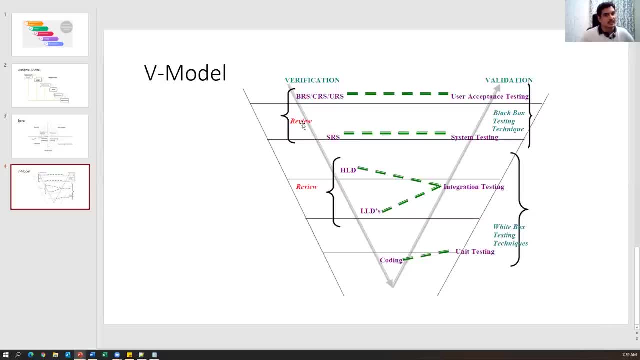 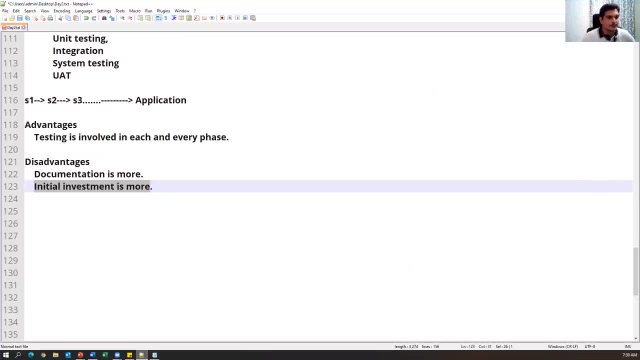 will be there from the beginning of software development process. So that is the reason cost is high. Initial investment is more because we have to pay them from the beginning itself And documentation will be there in each and every phase. That takes a lot of time: Preparation. 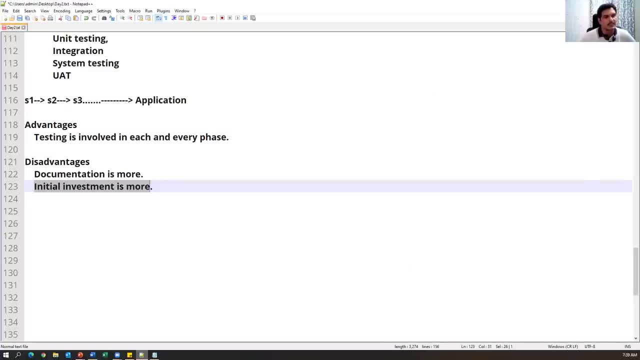 of document is not simple thing. It takes a lot of time to document each and everything. So these are the disadvantages in B model. And the advantage is in every phase we have testing involved. So that is the reason in the coming phases there are less number of 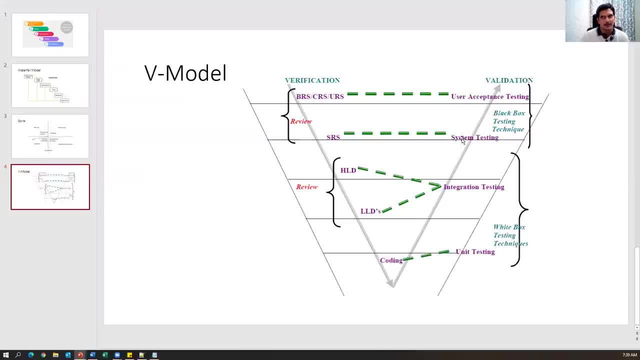 chances are there to get the bugs in system testing, because once we reach this level already, different levels of testing are done, So very less number of chances are there to get the bugs in the later stages. OK, So these are the advantages of B model. So 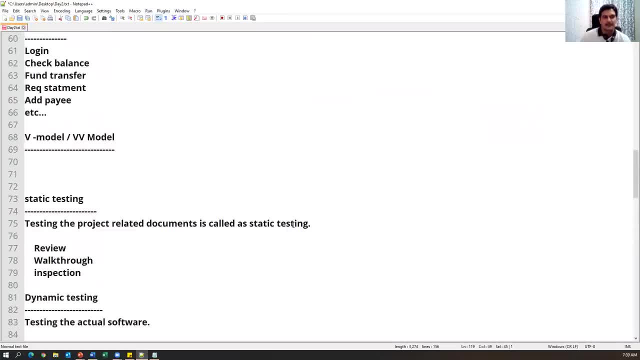 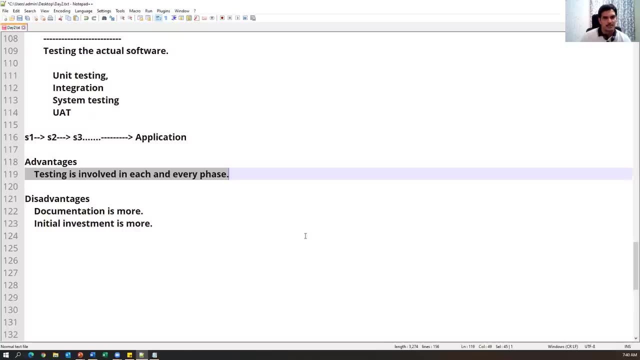 these are the 3 main advantages of B model. models comes under sdlc. we have discussed about waterfall model, then spiral model and then v model. okay, so understood guys. so let me just uh write some notes. okay, so we have. let me open the document. so we have discussed what is sdlc, what is software development life cycle, basically it. 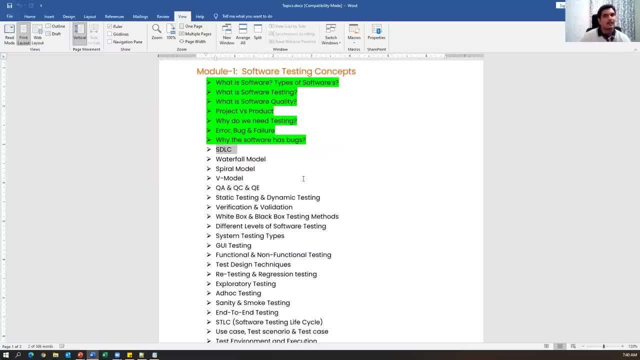 is a process, step-by-step process, which you have to follow to develop the software and what it includes. it includes requirement analysis, design, coding, testing, deployment and maintenance. that is sdlc. and waterfall model, spiral model, v model. so these three are sdlc models you can call them. 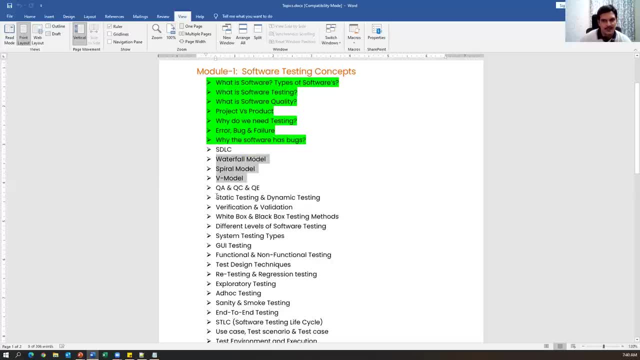 as sdlc models, and we have also discussed about static and dynamic testing. so static testing means what we are testing: the documents in the form of reviews, walkthroughs and inspections. dynamic testing means what we are actually testing: the software, unit testing, integration testing, system testing- uid testing comes under dynamic testing again. 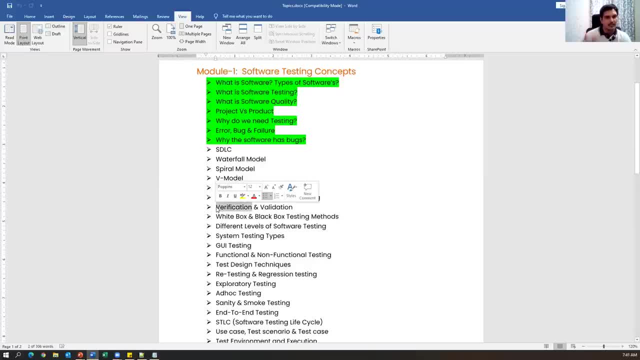 verification means what we are checking: whether we are following correct process or not. we are documenting correct or not. documents are right or wrong. that is, verification will be done before software is ready and once the software is ready, we do. validation means what? whether software is working according to requirement or not by giving different inputs, observing the output from the. 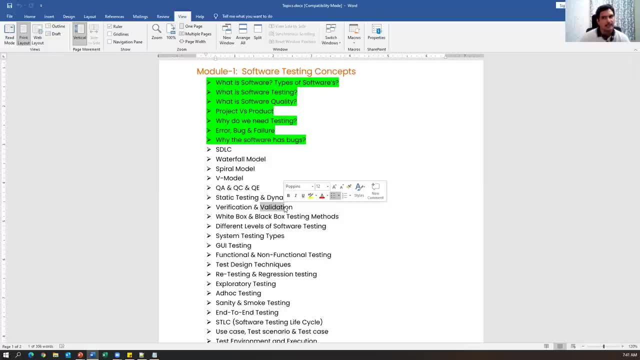 software. we are doing validation, you know, inside the developing text field we are getting the been testing as well. so you can see these three, threeны26. it is defining two types of testing. we do not know exactly. we have to know exactly what is there inside the model, the coding part we have to know. so that is the reason only. 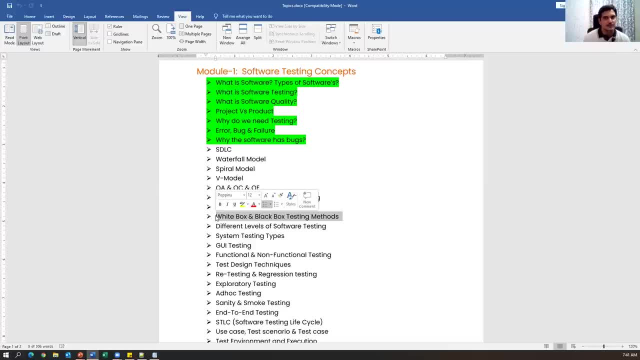 developers can do the testing. so white box testing means you need testing and integration testing comes under white box. and black box testing means what system testing and user accept testing. we do not need to know the code pack. so this is a good process. so the first thing we have to